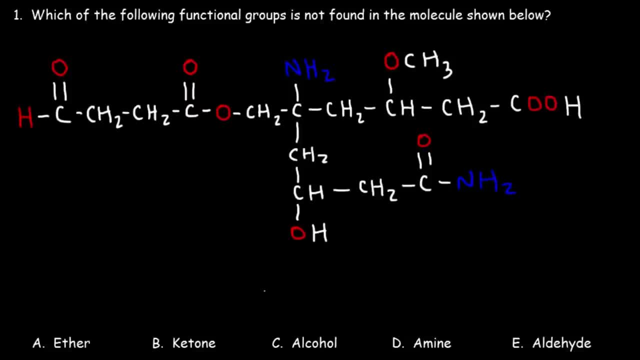 This multiple-choice final exam review is for those of you who are taking the first semester of organic chemistry, So let's go ahead and begin. Number one: which of the following functional groups is not found in the molecule shown below? For each of these questions, pause the video and work on the problem first See if you can get the right answer. 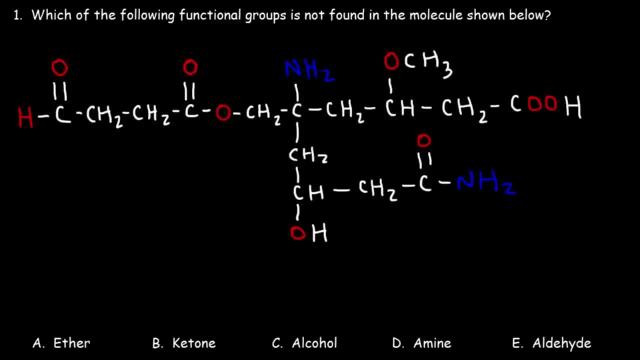 And then, once you have selected your answer, unpause the video to see the solution. So let's go ahead and begin. Our goal is to find out which functional group is not found in the molecule. So let's identify all the functional groups that are in the molecule. 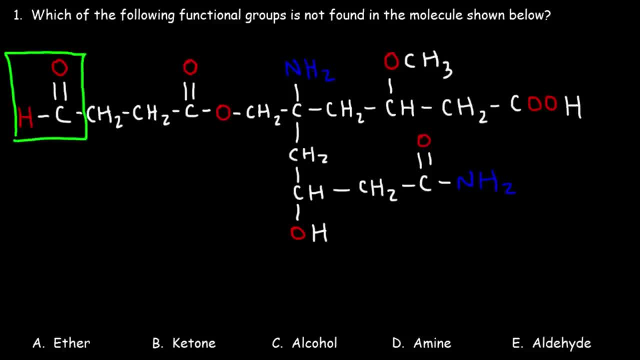 So what is this? What functional group do we have here? CHO- This is equivalent to this expression here. That is an aldehyde, So therefore we can eliminate answer choice E. Now what about this functional group, This functional group in the middle with two oxygens? What is that called? 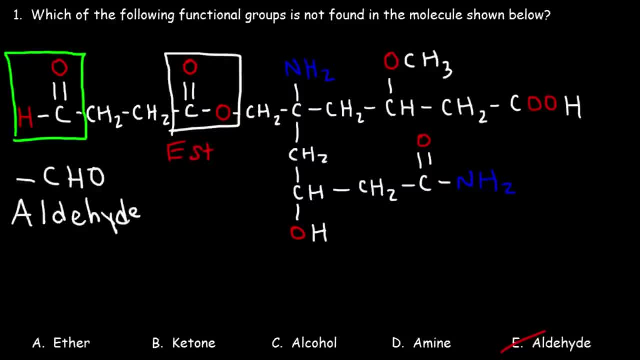 That functional group is known as an ester. An ester has this general shape: It has a carbon with two oxygens and it has an R group, One attached to the carbon and the other attached to the single bonded oxygen atom. So that's an ester. 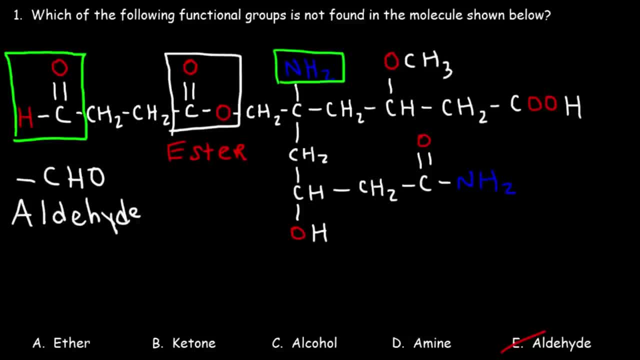 After that we have an NH2 group. This is known as an amine. You can also divide it as R and NH2.. So D is out of the question. What about this group, This OCH3 group? What functional group is that? 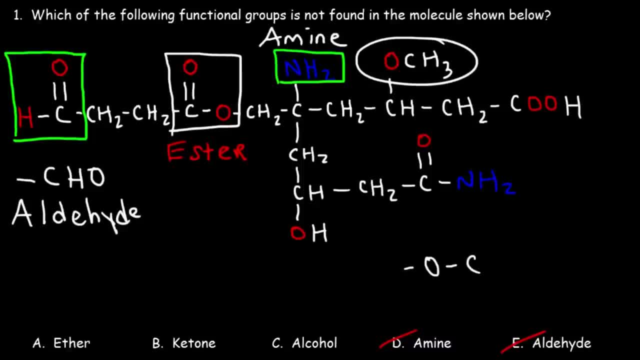 So notice that we have an oxygen attached to two carbons, Which is basically equivalent to an oxygen attached to two R groups. This is known as an ether, So A is eliminated. Next we have a COOH group. That is known as a carboxylic acid. 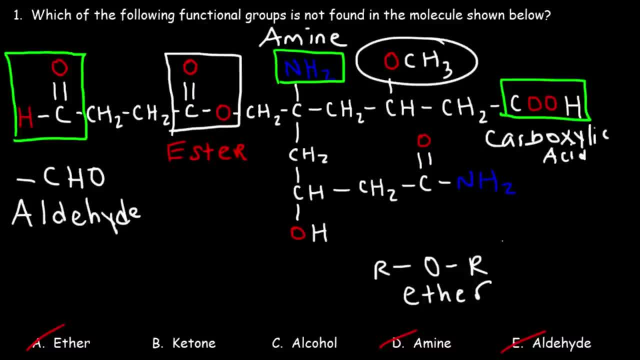 Which, if you write it out, it will look like this: You have an R group and then you have a carbon which is double bonded to an oxygen and it has an OH. So that's a carboxylic acid And this is an ether. 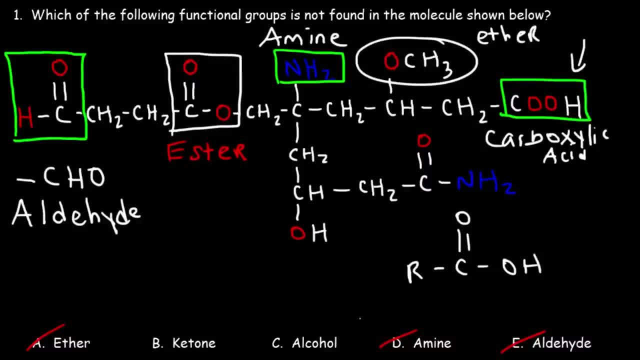 Now, the carboxylic acid is not listed as an answer, so we don't have to worry about that. Next, we have this OH, which is an alcohol, So C is eliminated, which means that B is the right answer. 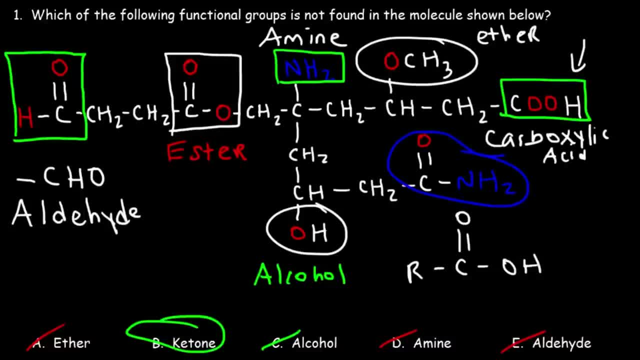 And what about this group? What is this group called? So, as you can see, if you see a carbon attached to an NH2 group, that's an amine. If you have an NH2 group attached to a carbonyl group, 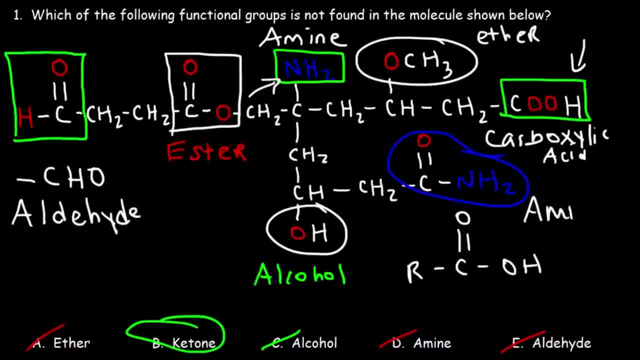 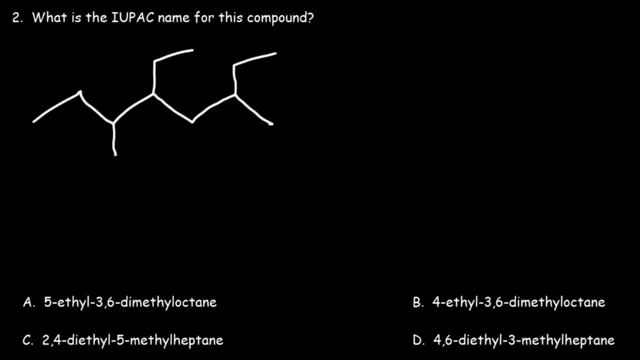 that is known as an amide, Or amide Which is not listed. So therefore, answer choice B is the right answer for this problem. Number two: What is the IUPAC name for this compound? Is it A, Is it B? 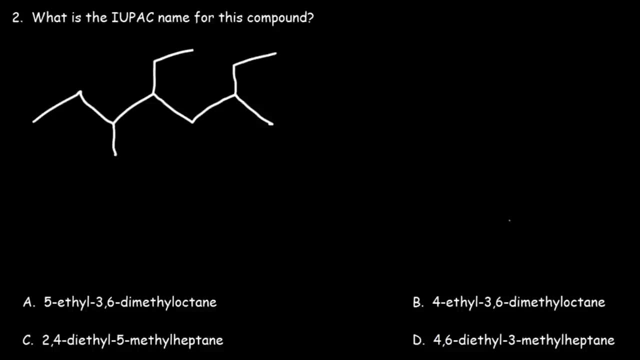 Or is it C or D? Well, let's find out. The first thing that we need to do is we need to identify the longest chain, So let's begin counting from left to right. This is one, two, three, four, five, six. 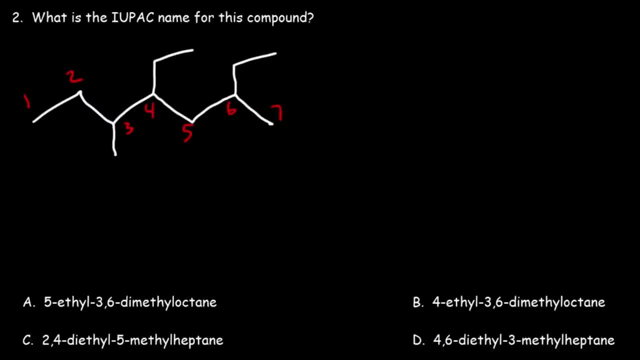 If we go to the right it's seven, But if we go up it's eight. So that is the longest chain. Eight carbons is associated with octane, So we can eliminate answer choice D And C because the parent name is heptane. 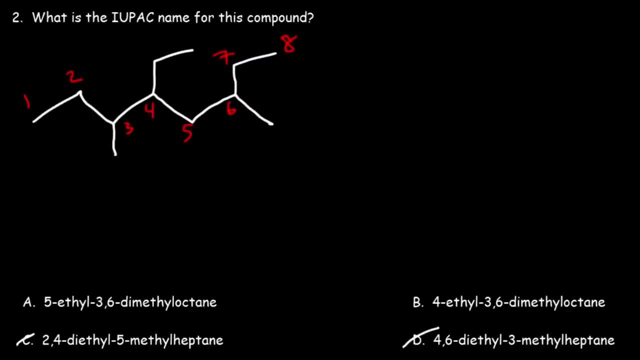 Now here's a question for you: Should we count it from left to right Or right to left? If we count it the way we have it, notice the substituents. We'll have a methyl on three, a methyl on six. 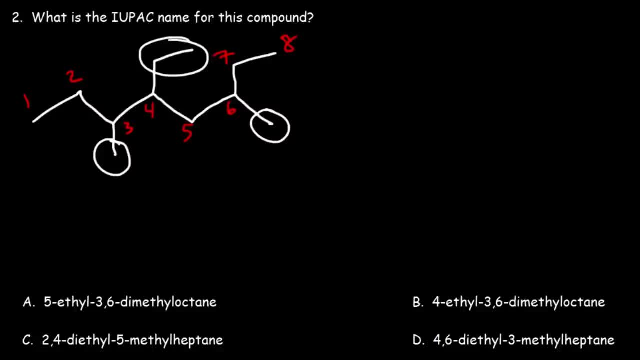 and an ethyl on four, Which correlates to answer choice B. B has an ethyl on four and two methyls on three and six. Now, if we count it the other way, notice that we still have a methyl on three and six. 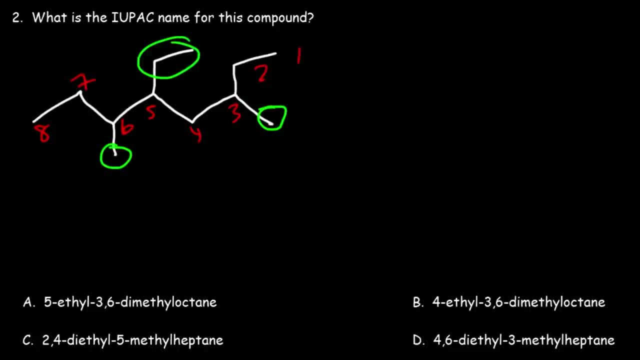 but we have an ethyl on five, Which correlates to answer choice A. So do we want the ethyl to be on four or on five? You want to count it in such a way that the substituents have lower numbers, So therefore B is the right answer. 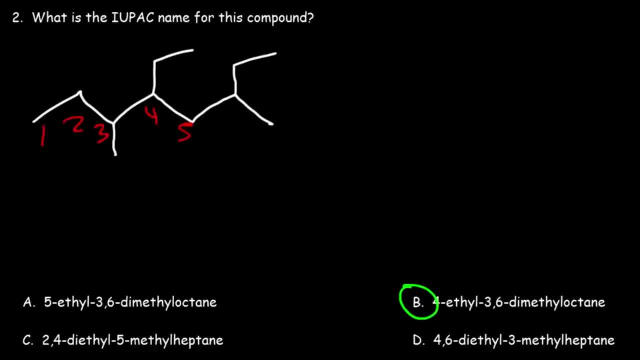 So you want to count it in this direction. So when you name it, you want to start with ethyl, Since E comes before M, And then we have a three, six, dimethyl, And then, because we have an eight carbon chain, it's octane. 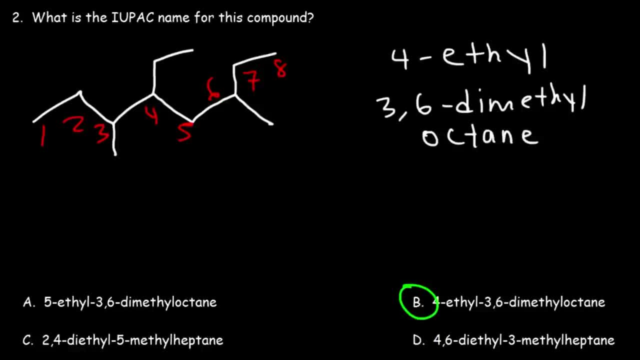 If you recall, methane is associated with one carbon, ethane, two, propane, three, butane is four, pentane is five, hexane is six, heptane is seven, octane is eight, nonane is nine and decane is ten. 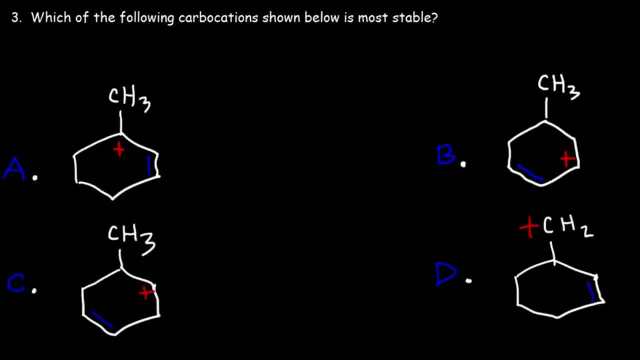 So B is the right answer for this problem. Number three: Which of the following carbocations shown below is most stable? So what do you think the answer is going to be? So go ahead and take a minute and work on this example. Now, what we need to keep in mind is that 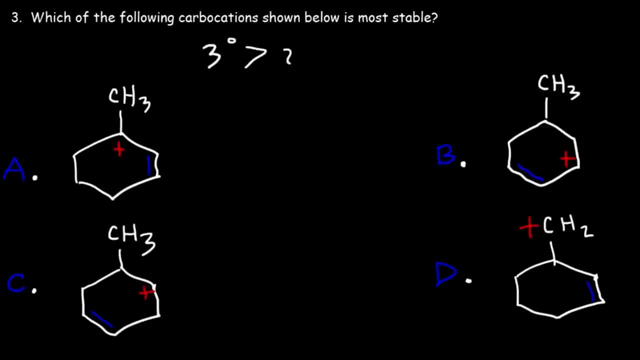 tertiary carbocations are more stable than secondary carbocations, which are more stable than primary carbocations, And the reason for this is due to the inductive effect and hyperconjugation In the inductive effect the carbon atoms, which are electron donating groups relative to the positive charge. 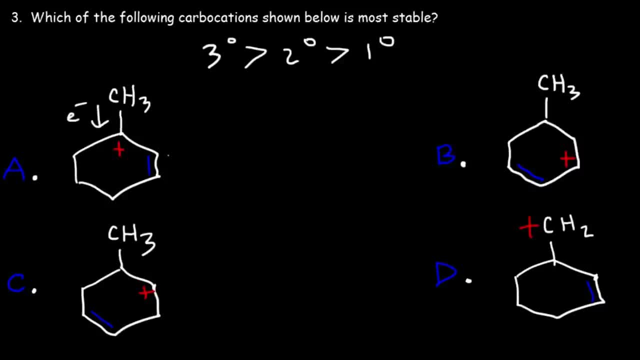 they can donate electron density to the positive charge by means of the inductive effect, that is, through the sigma bond. So that's one way they can donate electron density to a starving carbocation which really wants electrons. The other way is by means of the overlap of atomic orbitals. 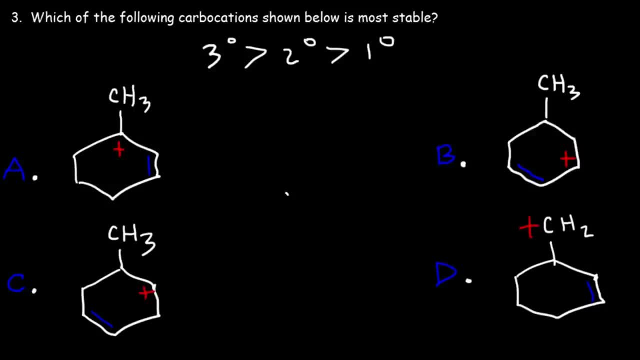 which is known as hyperconjugation. So let's say, if you have a carbon atom with a plus charge and let's say there's another CH3 group and so here's a CH bond that's next to it, So there are electrons in this orbital. 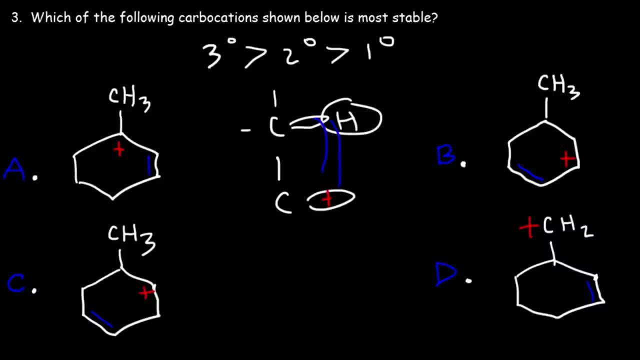 and that orbital can overlap with the MTP orbital below it. And so that's how electron density can be donated to the carbocation: by means of hyperconjugation, which is through the overlap of atomic orbitals. So when these two orbitals overlap, 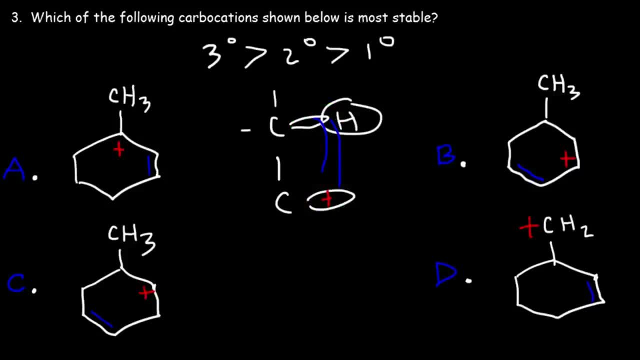 electron density can be shared. So those are the main reasons why tertiary carbocations are more stable than primary ones. A tertiary carbocation is basically a carbon that has three other carbons attached to it, And the carbon in the middle has a plus charge. 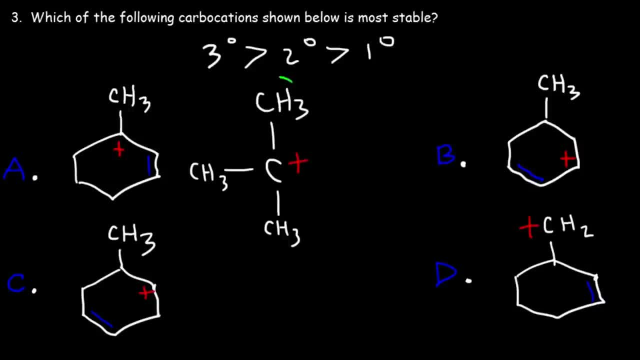 so it's a carbocation. So that's why it's called tertiary, because there's three carbons attached to the carbon, with the plus charge, And the more methyl groups that you have next to the carbocation, the more electron density that can be donated. 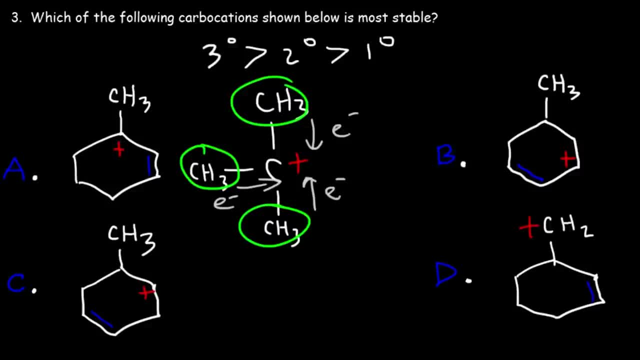 which means you have a more stable carbocation. Now what about allylic carbocations? A secondary allylic carbocation is more stable than a regular secondary carbocation. An allylic carbocation is one that has a plus charge, one carbon away from the double bond. 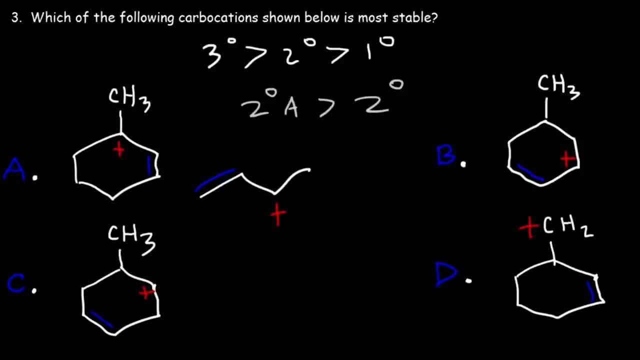 And the reason why allylic carbocations are relatively stable is due to the resonance stabilization of the carbocation. This double bond can move here, creating a resonance form that looks like this: So, as you can see, the plus charge is shared between two carbon atoms. 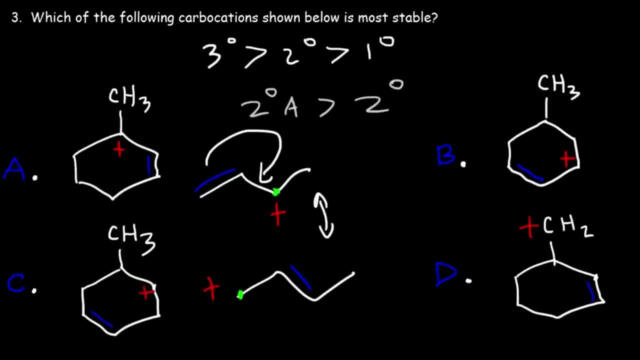 as opposed to one And, as a result, they're more stable. So those are the main things you need to look for. So keep in mind that tertiary carbocations are more stable than secondary and primary ones, and that allylic carbocations are more stable than those that are not allylic. 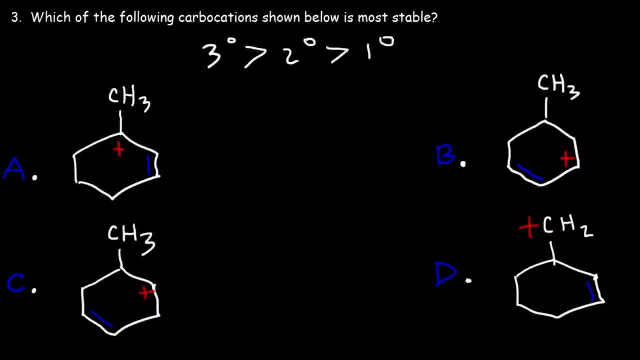 Now let's identify the type of carbocation that we have in every choice. So let's start with part A. What type of carbocation do we have? So let's focus on the carbon with the plus charge. How many other carbons are attached to it? 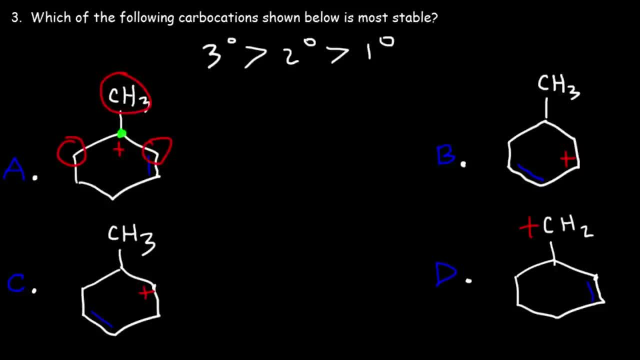 So we have one, two, three, Because there are three carbons attached to it. it is a tertiary carbon, And notice that it's one carbon away from a double bond, which means it's tertiary and it's allylic. Now, what about B? 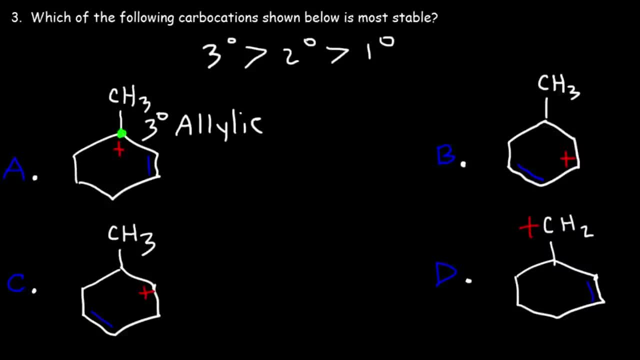 What type of carbocation do we have? So, focusing on the carbon with the plus charge, that carbon is attached to two other carbon atoms And it's adjacent to a double bond, which means that it's secondary and it's allylic. So, moving on to part C, 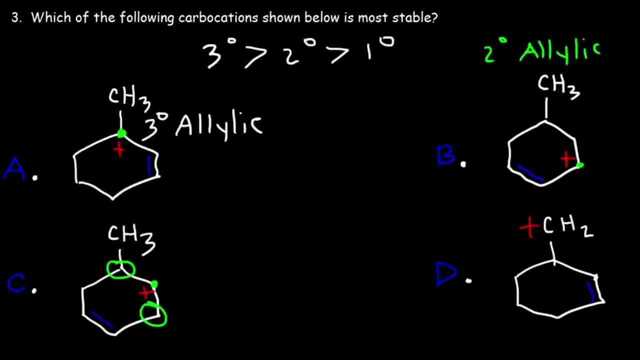 The carbon with the plus charge is adjacent to two other carbons, but it's too far away from the double bond, So it's simply a secondary carbocation. And now this carbon with the plus charge is only attached to one carbon atom, which means it's a primary carbon. 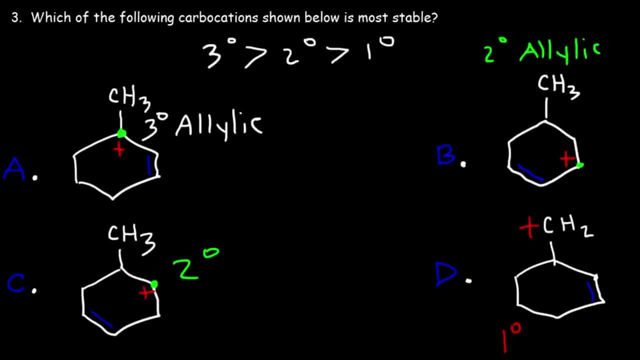 and it's too far away from the double bond, so it's not allylic. So therefore D is the least stable. Primary carbocations are not stable at all. The most stable is answer choice A. It's tertiary and it's allylic. 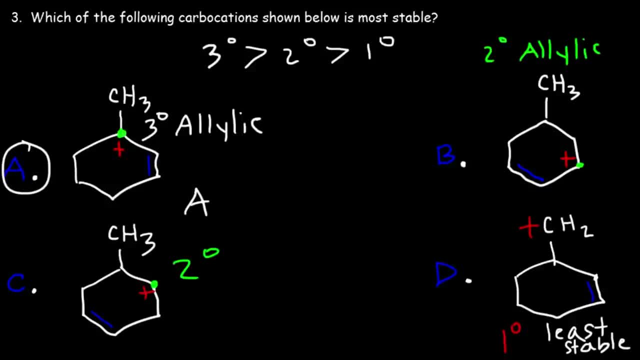 So if we had to rank it compound, A is the most stable. After that, the next most stable is B. A secondary allylic carbocation is more stable than a regular secondary carbocation due to resonance, And then B is more stable than C. 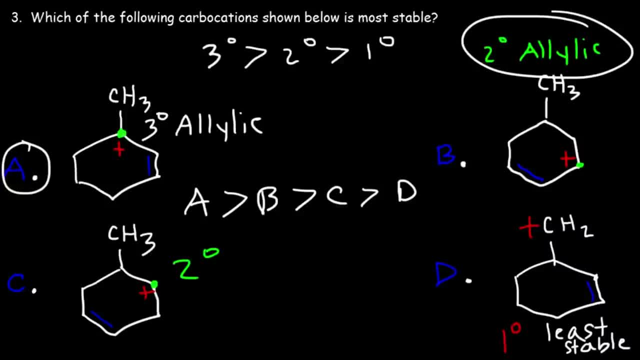 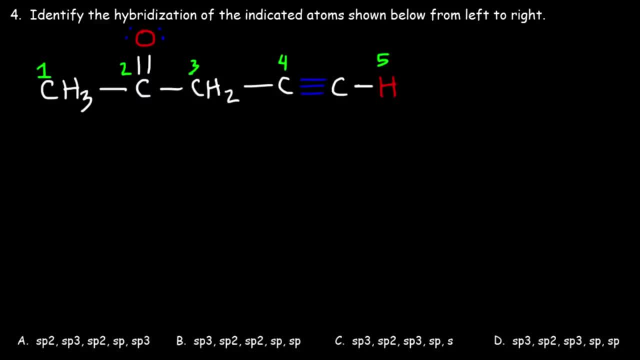 and D is the least stable, But answer choice A is the answer. That's the most stable carbocation that we have in this selection. Number four Identify the hybridization of the indicated atoms shown below from left to right. So is it A, B, C or D? 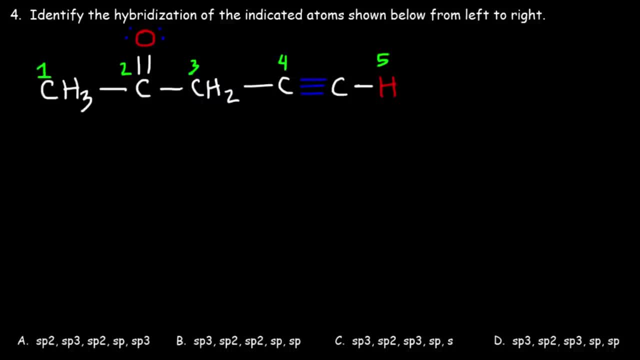 How can we determine the hybridization? So feel free to try this one Now. before we work on the solution, let's review how to find the hybridization of an atom. So let's start with methane, CH4.. So what you want to do is count the number of groups. 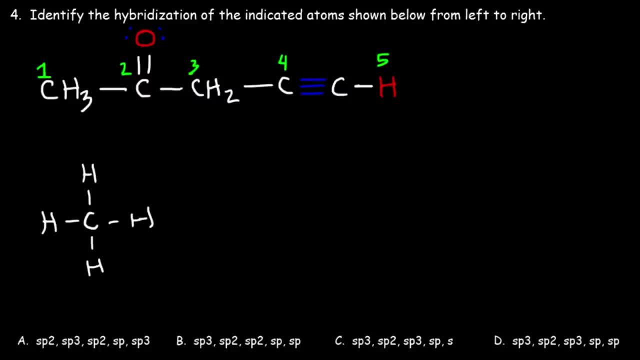 and lone pairs attached to the carbon. Single bonds, double bonds, triple bonds. count them as one group. So one, two, three, four. The carbon atom has four groups. Four groups correlates to sp3, s1p3. 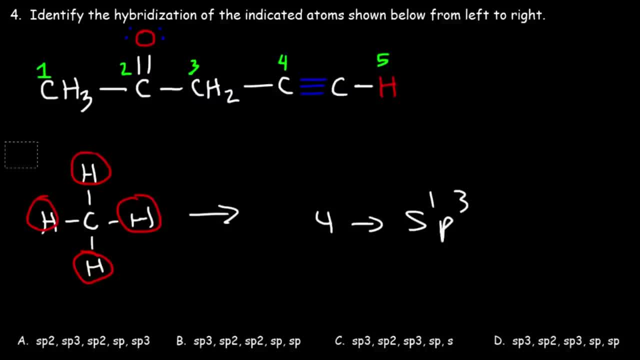 One plus three adds up to four. So that's the hybridization on the center carbon atom. So let's do some more examples so you can get familiar with this. Next, let's try formaldehyde, since it has a double bond. Now how many groups are attached to the carbon atom? 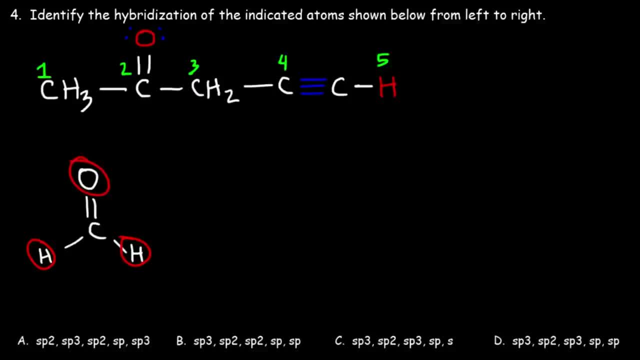 One, two, three Treat the double bond as one group, don't count it as two. So we have three groups, which corresponds to sp2.. One plus two adds up to three. Three groups will always correspond to sp2.. Four groups will always correspond to sp3.. 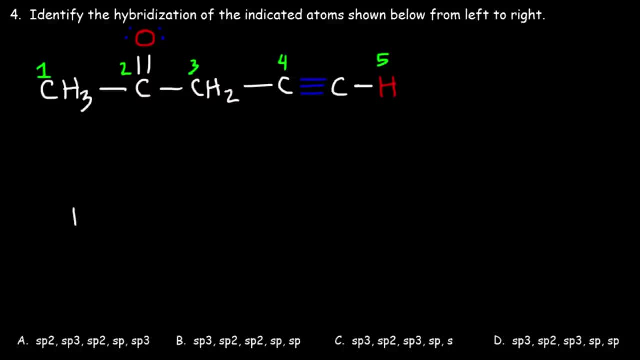 That's a quick and simple way to find the right answer. Now let's try acetylene. What is the hybridization at the carbon and at the hydrogen? So if we focus on a carbon atom, that carbon atom is attached to a hydrogen and a CH group. 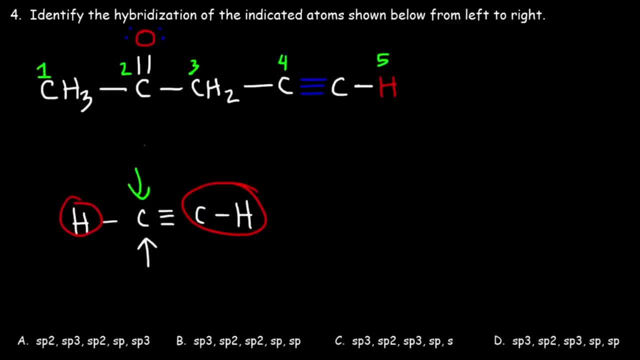 So it has two groups, which means that it's sp hybridized. Two is basically one plus one. If you don't see an exponent, it's one. Now what about the hybridization on hydrogen? Hydrogen is only attached to one atom. 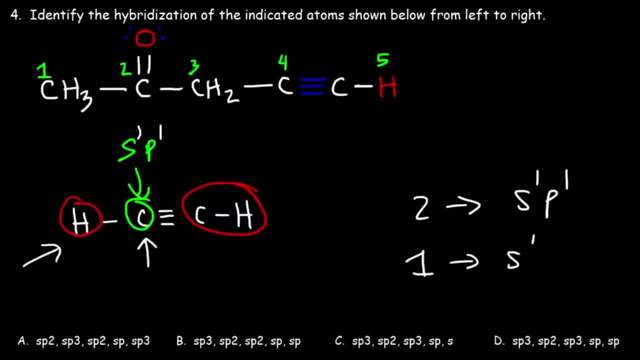 So it only has one group. One group correlates to s. Now what if there are lone pairs? Let's use ammonia as an example: NH3. What's the hybridization on the nitrogen atom? So what we need to do is count the number of groups and lone pairs. 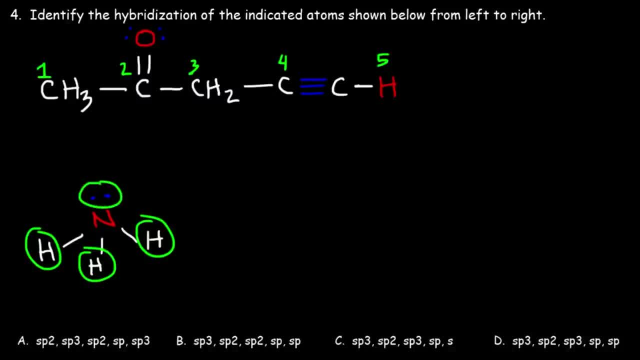 So nitrogen has three atoms and a lone pair, so it has four groups And four correlates to sp3.. One plus three adds up to four. Next, let's use sulfur dioxide as an example. So here's the Lewis structure of SO2.. What's the hybridization on the sulfur atom? 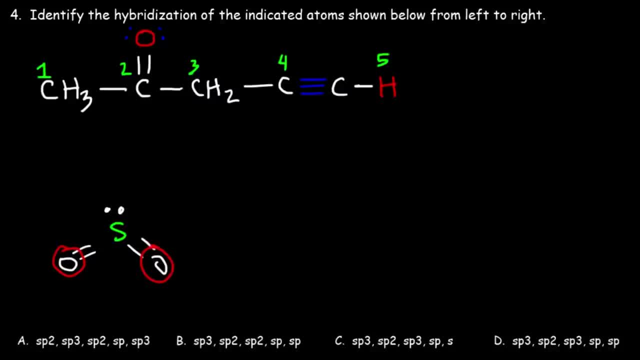 So sulfur has two groups and a lone pair, So it has a total of three groups, which is sp2.. So it's sp2 hybridized. Now what if we have more than four groups? Let's use phosphorus pentachloride, for example. What's the hybridization on a central phosphorus atom? So here we have a total of five groups, So it's going to be s1p3d1.. s only has one orbital, so there's no s2.. p only has three orbitals, so you shouldn't have p4.. 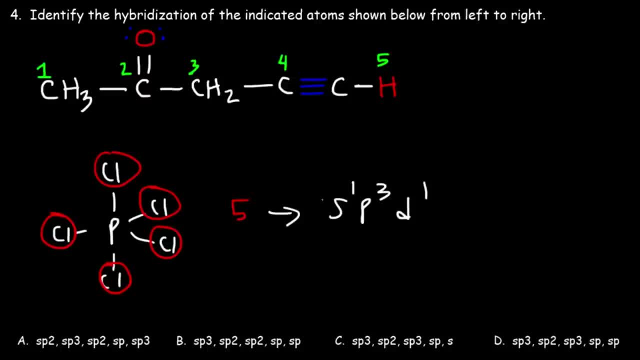 d has five orbitals, so we don't have to use all five. The exponents have to add up to five. One plus three plus one is five. So therefore, what do you think the hybridization will be for sulfur hexafluoride. 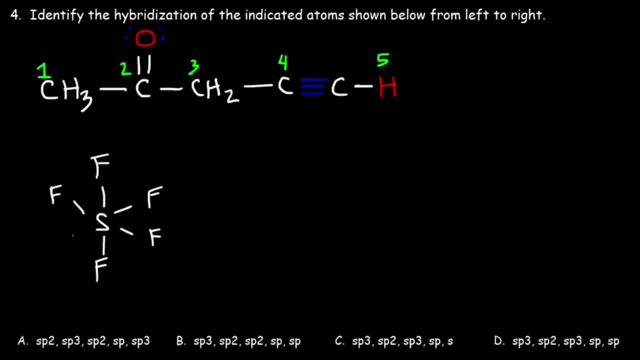 Sf6. So sulfur has six groups in this case. So six corresponds to s1p3d2.. One plus three plus two is six. So now that you know how to find the hybridization of an atom, go ahead and finish this problem. 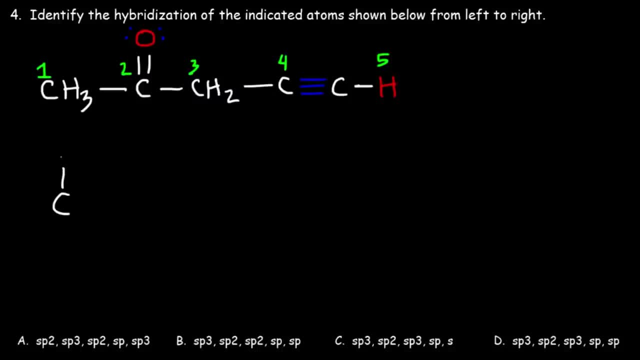 So let's start with CH3.. So we have a carbon attached to three hydrogens and it's attached to carbon at the right. So let's put C here. So this carbon has four groups attached to it, which means that it's sp3 hybridized. 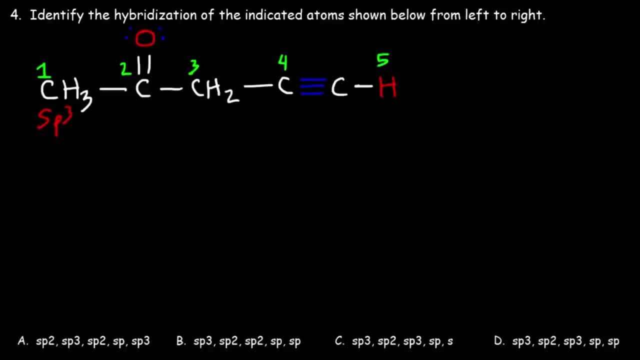 So let's put sp3 here. Now we need to go in order from left to right. So in each answer choice the first answer should be sp3.. We can eliminate A, which is sp2.. So we're between B, C and D. 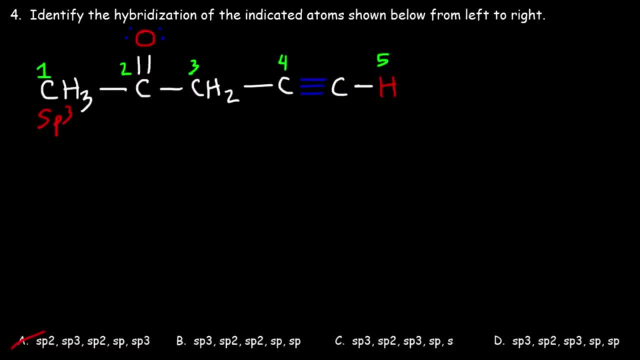 Now let's move on to carbon number two, So that carbon, we can see, has three groups. It's attached to the CH3 on the left, the CH2 on the right and the oxygen. Three groups correlates to sp2.. One plus two is three. 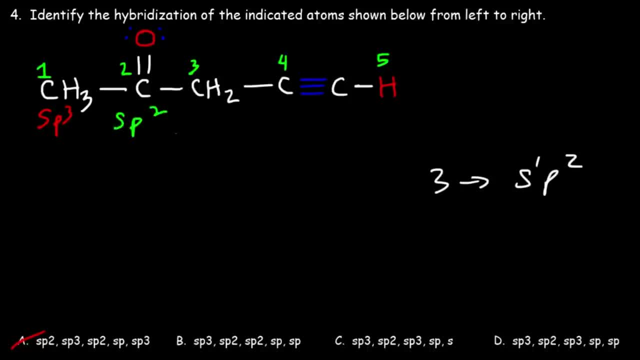 So that's the second answer: It's sp2.. So we can keep B, C and D the same. As you can see the second answer: they're all sp2.. So we can't eliminate anything at this point. Now let's move on to carbon, number three. 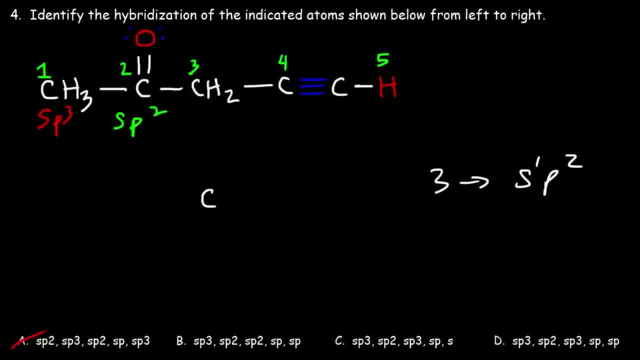 So we have a carbon that has two hydrogens, So we can draw it like this, And then to the right we have another carbon And to the left we have another carbon. So the carbon, the CH2 carbon, has four different groups. 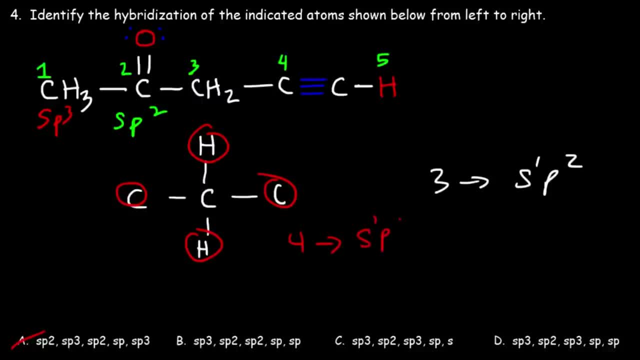 And, as we know, four correlates to sp3.. We can eliminate answer choice B because the third option is not sp3.. We need to keep C and we need to keep D. So, looking at C and D, we can see that the next option is sp. 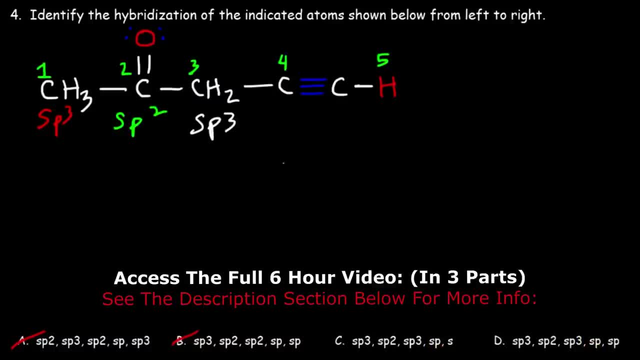 What we need to focus on is the last one. But if you look at this carbon, you can see why it's sp hybridized. It's attached to a carbon and another carbon, So it has two groups, which correlates to sp. 1 plus 1 is 2.. 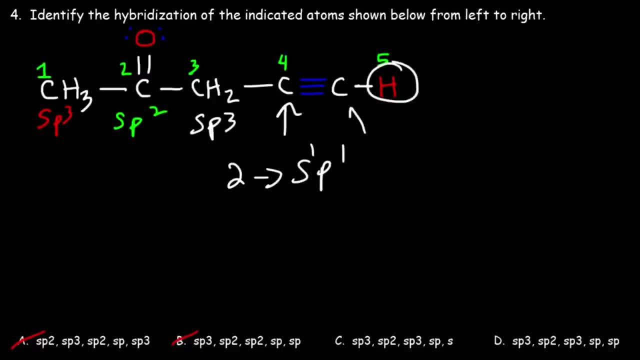 Now, if we focus on the hydrogen, that hydrogen is only attached to one group. It's attached to one carbon atom And one group correlates to s. So the hybridization for any hydrogen atoms is always s, because hydrogen cannot form two bonds. 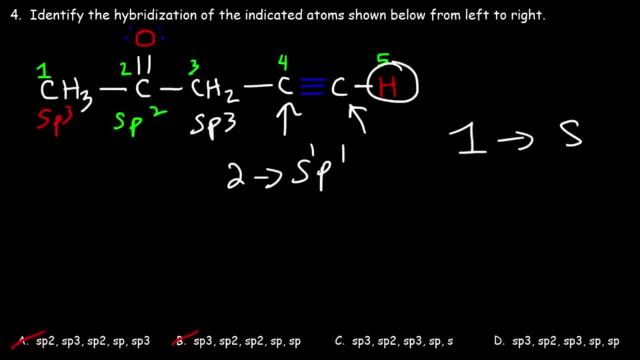 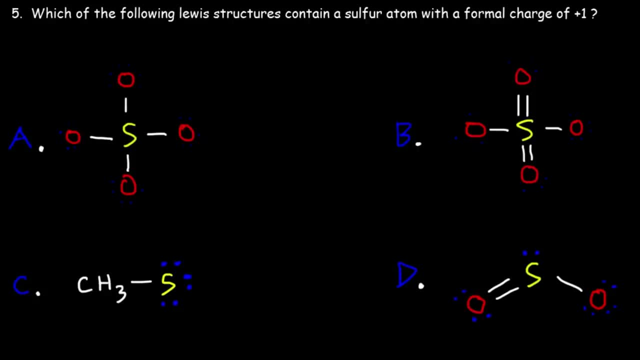 It can only form one bond, Which means that C is the right answer. D doesn't have s as the last option, So this is it, Number 5.. Which of the following Lewis structures contain a sulfur atom with a formal charge of plus 1?? 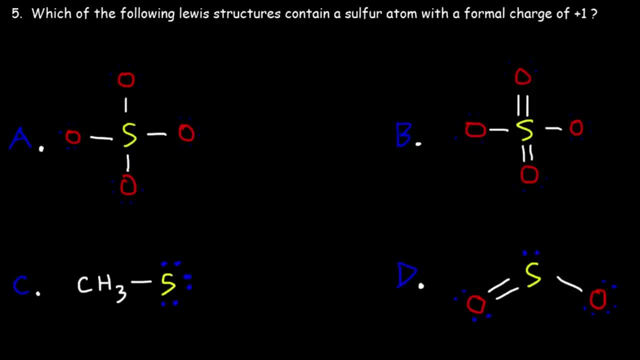 So go ahead and try this problem. The formula that I like to use is this one: The formal charge is equal to the number of valence electrons minus the number of bonds, plus the number of dots in the structure. So let's start with answer choice A. 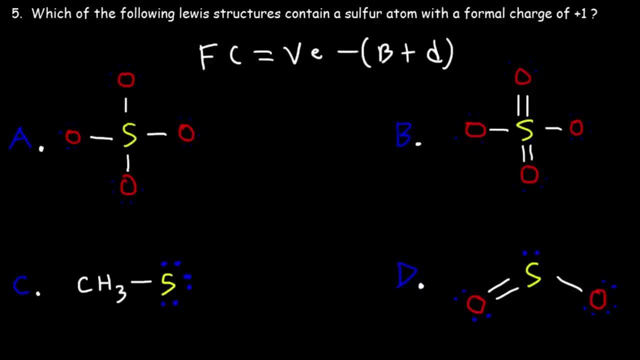 Sulfur has six valence electrons. If you go to the periodic table you'll find that sulfur is in group 6A of the periodic table And typically elements in that group have six valence electrons. So all of the sulfur atoms. 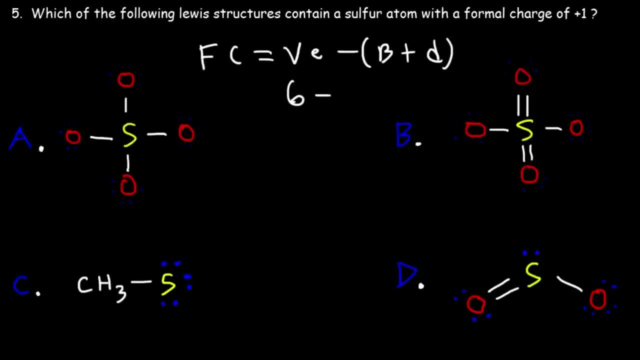 in each of these molecules have six valence electrons as a free atom, Now in structure A or in compound A. sulfur has four bonds: 1,, 2,, 3, 4. And it doesn't have any visible lone pairs. 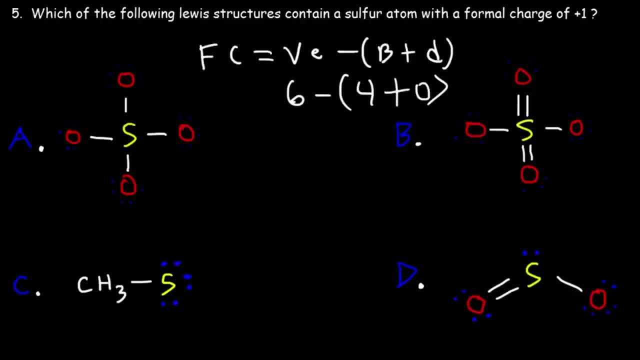 So it has zero dots. 6 minus 4 is 2.. So the formal charge on this sulfur atom is plus 2. So we can eliminate answer choice A. Now let's move on to B. Sulfur has six valence electrons. 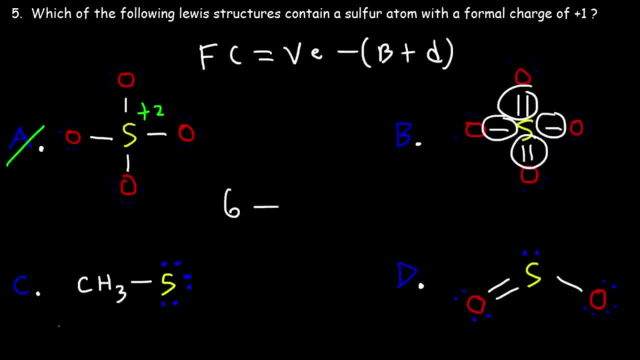 In B. it has six bonds: 2,, 3,, 4, 6.. It doesn't have any lone pairs, So the number of dots is zero. 6 minus 6 is zero, So we can eliminate answer choice B. 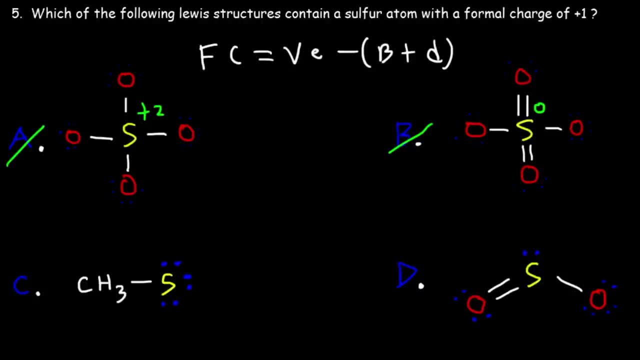 It's neutral in that molecule. Now let's move on to C. Sulfur has six valence electrons And in this structure sulfur has only one bond, But notice that it has six dots: 2,, 4,, 6.. 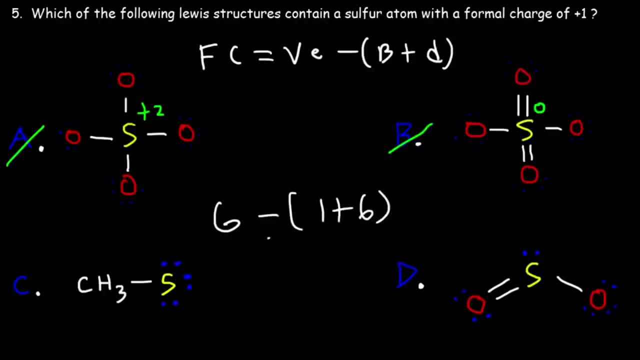 1 plus 6 is 7. And 6 minus 7 is negative 1.. Therefore we can eliminate answer choice C. So D has to be the answer, But let's go ahead and use the formula to get the answer. 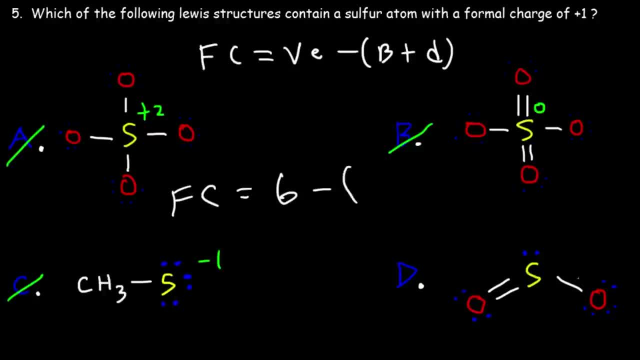 Sulfur has six valence electrons And this structure has one bond plus 2.. So that's three bonds in total And we can see that it has two dots or one lone pair. 3 plus 2 is 5.. 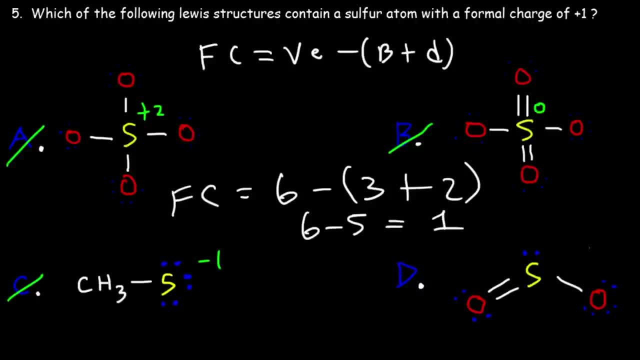 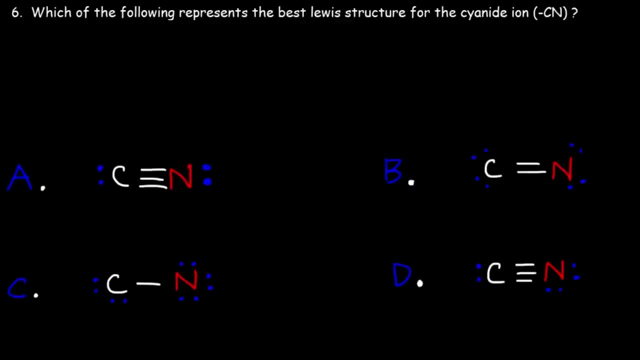 6 minus 5 is 1., And so that's the formal charge of sulfur in answer choice D. So D is the answer. That's what we're looking for, Number 6.. Which of the following represents the best Lewis structure for the cyanide ion? 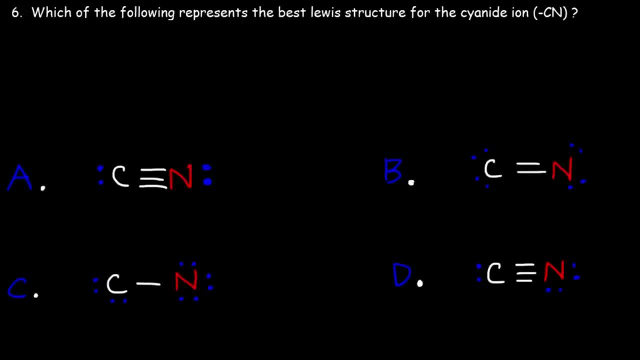 Is it A, B, C or D? So which answers can we eliminate? We're looking at answer choice D. Notice that nitrogen, which is a second row element, has more than eight electrons. Every bond represents two electrons, So it has a triple bond. 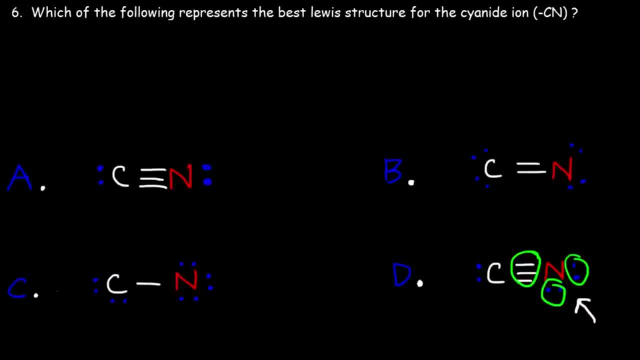 which equates to six electrons and two lone pairs. So nitrogen has ten electrons around it, which violates the octet rule. Elements in the second row, like carbon, nitrogen, oxygen and fluorine. they cannot have more than eight electrons. 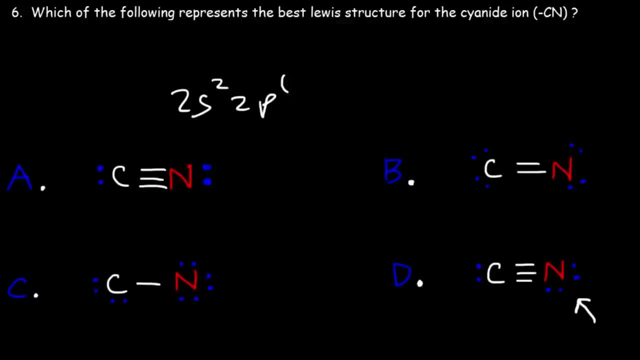 In the second row you have 2s2, 2p6, there is no 2d10.. So second row elements can have at most eight electrons. 2 plus 6 is 8.. So we can eliminate D. 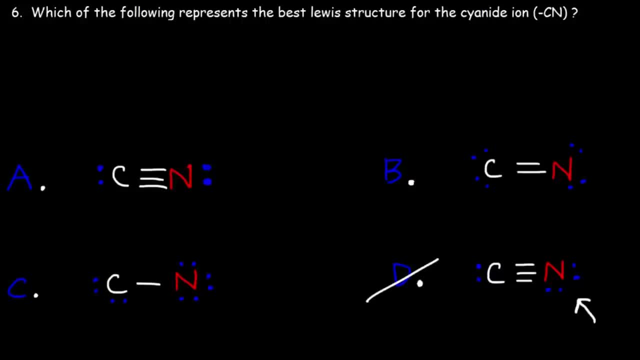 Nitrogen violates the octet rule. Now in answer, choice C. what's the issue here? Carbon has an incomplete octet. Notice that it doesn't have eight electrons. it has six. Now it's possible for an element to have six. 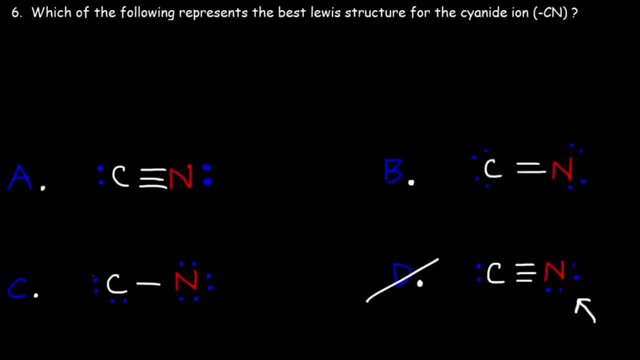 However, it's not stable. It's not the best Lewis structure. It has two, four, six electrons, so we can eliminate answer choice C. Answer choice A and B: Carbon and nitrogen both have eight electrons, which means that their octet requirements are satisfied. 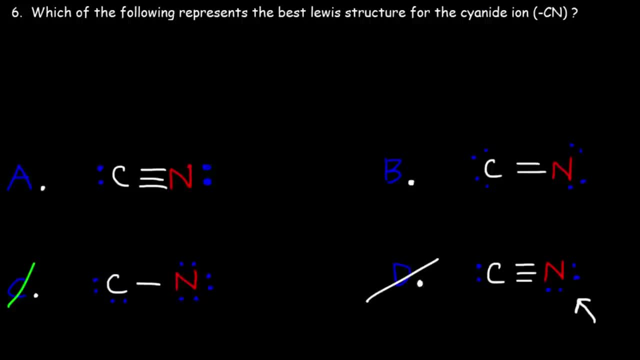 Now what we need to look at is the formal charge. We need to find out which one is more stable. The compound that is most stable is the one with the minimum formal charge, where the formal charge is closest to zero. So let's start with B. 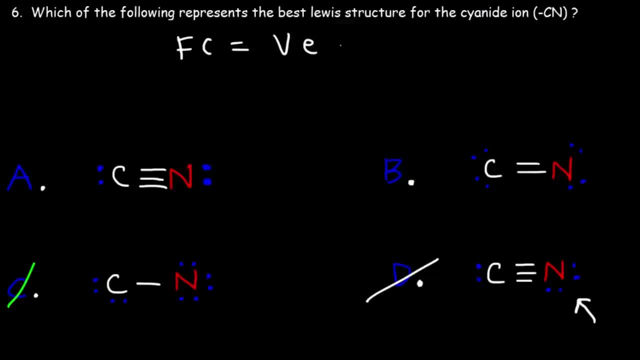 Let's calculate the formal charge. We know it's equal to the number of valence electrons minus the bonds, plus the dots. So, starting with carbon, carbon has four valence electrons. naturally It's in group 4A of the periodic table. 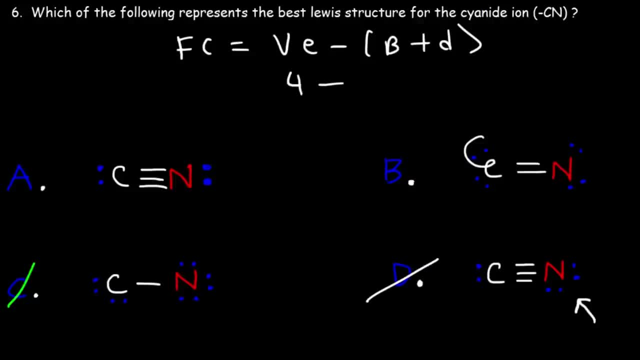 And in this structure it has two bonds and it has four dots. Two lone pairs corresponds to four dots. Every lone pair has two dots. So two plus four is six, and four minus six is negative two. So that is the formal charge. 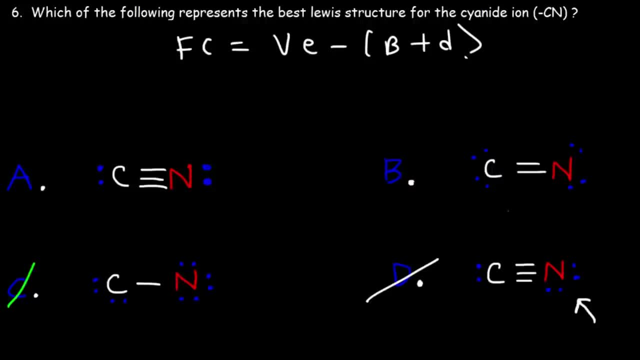 of carbon in this structure. So let's go ahead and write that. Now what about the formal charge of nitrogen? Nitrogen naturally has five valence electrons, It's in group 5A of the periodic table And in this structure it has two bonds. 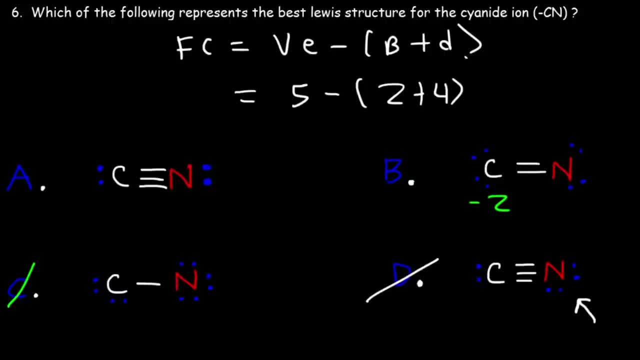 and it also has four dots. So two plus four is six. five minus six is negative one. Now let's go ahead and calculate the formal charge of carbon and nitrogen in the other compound. So, starting with carbon, we can see that it has three bonds. 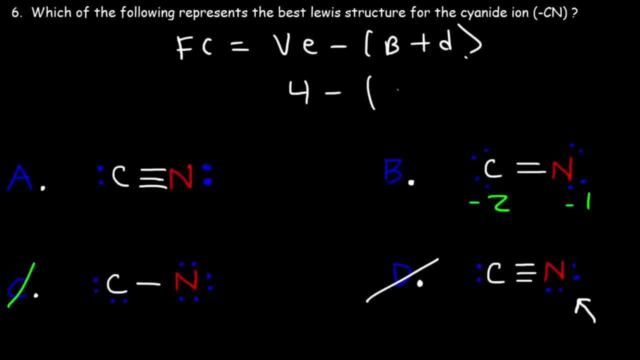 one lone pair. So it has three bonds and two dots. Three plus two is five. four minus five is negative one. Now what about nitrogen? Nitrogen has five valence electrons. It too has three bonds. It has a triple bond. 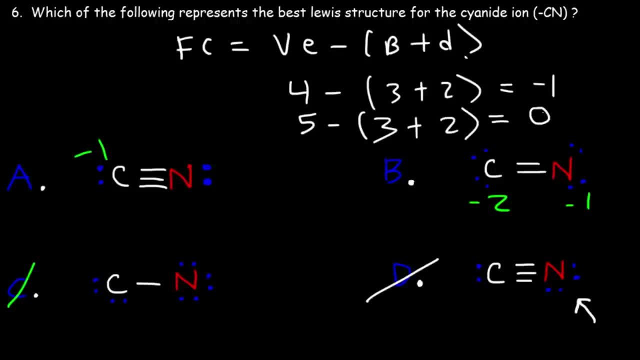 And it has a lone pair, so two dots. Five minus five is zero. So is it better to have a formal charge of negative one and zero or negative two and negative one? Negative one is closer to zero than negative two is, So we can eliminate B. 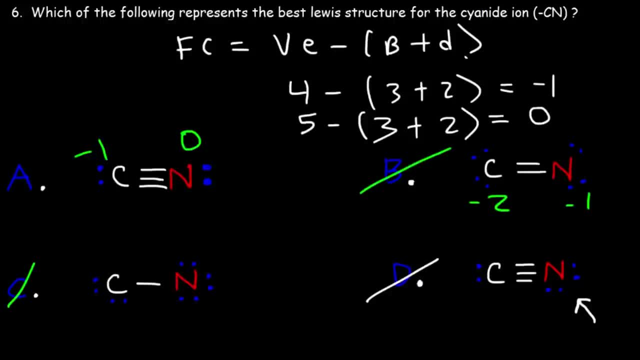 If you have a formal charge of negative two, it's not good, It's not stable. Also, the total charge for cyanide has to add up to negative one. If we add these charges, they add up to negative one. If we add these two charges, 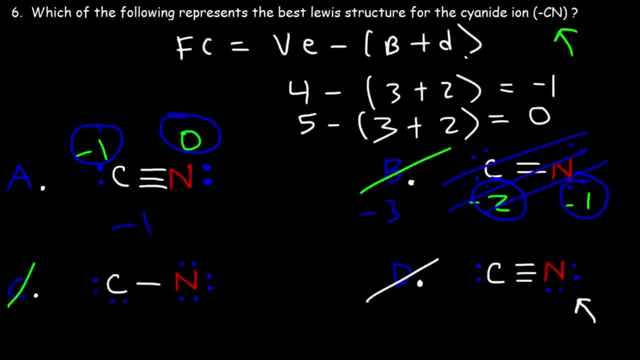 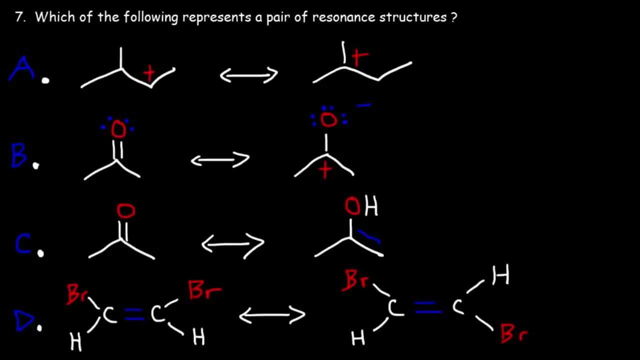 they don't add to negative one. So this is not the correct Lewis structure for cyanide. This is it. Number seven, Which of the following represents a pair of resonance structures? Do you think the answer might be A, B, C or D? 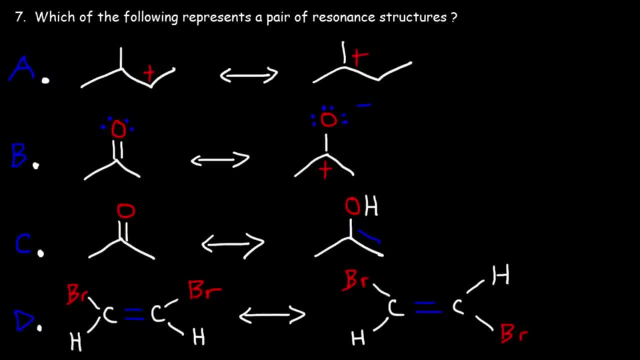 So what can we do in order to identify a pair of resonance structures? Is there a better way of figuring this out instead of drawing everything? It turns out that there is A quick way to identify a pair of resonance structures is to identify the ones that are not. 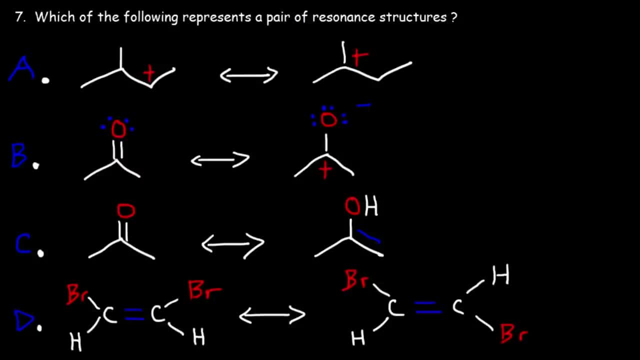 resonance structures. If any atoms are moving from one spot to another spot, it's not a resonance structure. If you want to draw a resonance structure, only the electrons are free to move and not the atoms. So if we look at answer, choice A- 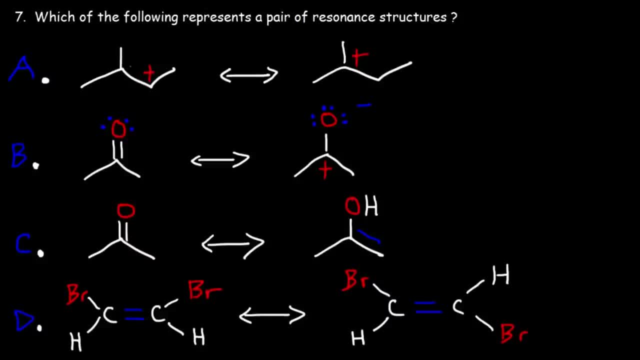 this represents a hydride shift. The hydrogen moves from the tertiary carbon to the secondary carbon And when that happens the plus charge is going to move from the secondary carbon to the tertiary carbon. So basically they trade places. So because the hydrogen was moved, 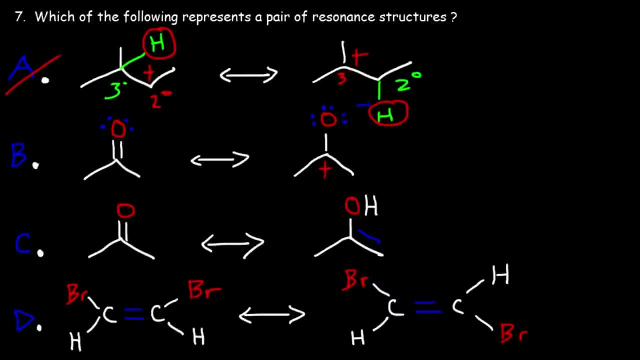 this is not a pair of resonance structures. Now, looking at D, we can see that the location of the bromine atom and the hydrogen atom were reversed. So anytime you're moving around atoms it will not be a resonance structure. So D can be eliminated. 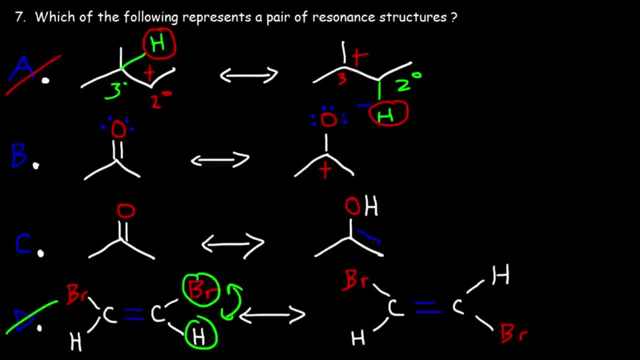 In fact, these are basically cis and trans isomers. This is the cis isomer and this is the trans isomer. In the cis isomer, you have two groups facing one side And in the trans isomer, the two groups are on the opposite sides. 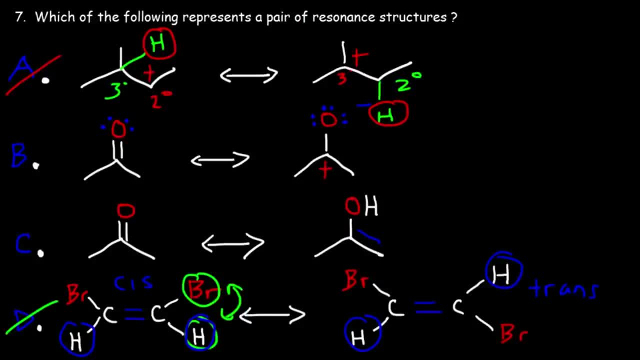 Now let's move on to part C. Notice that we have a ketoenol tautomerization going on here. A hydrogen was moved from this carbon onto the oxygen. Before there were three hydrogens and now we only have two, So hydrogen was transferred from one part of the molecule. 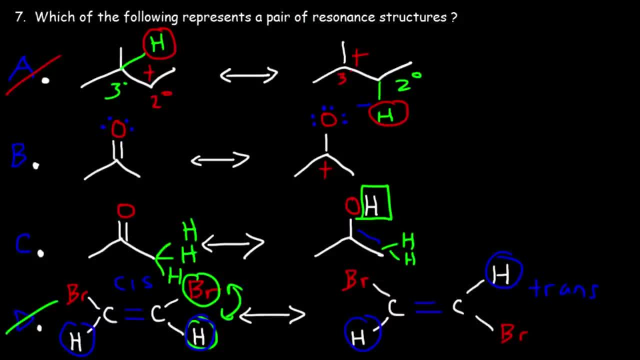 to the other part of the molecule, Which means that these two do not represent a pair of resonance structures. The only answer is answer choice B. If you draw all the hydrogen atoms, notice that none of them were moved. We still have six hydrogen atoms. 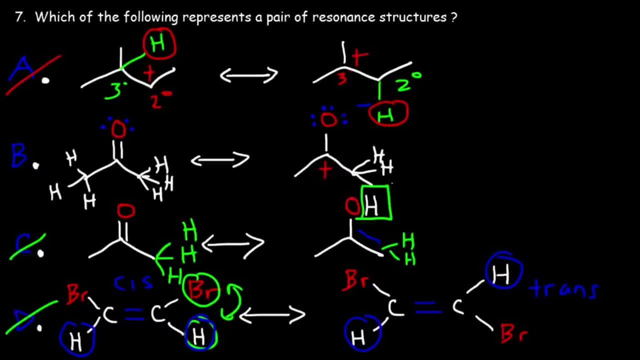 three on each carbon, and so no hydrogens were transferred. The only thing that moved were the electrons. Two pi electrons in the double bond was transferred to the oxygen, as we can see here, And any time you move electrons without moving atoms. 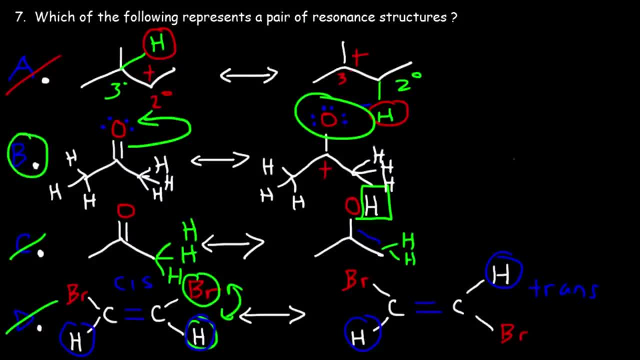 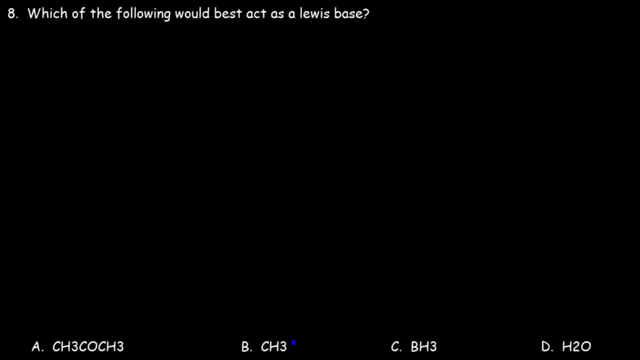 you're going to generate a resonance structure, So answer choice B is the right answer. Number eight: Which of the following would best act as the Lewis base? So in this problem we need to identify which ones are the Lewis acids and eliminate them. 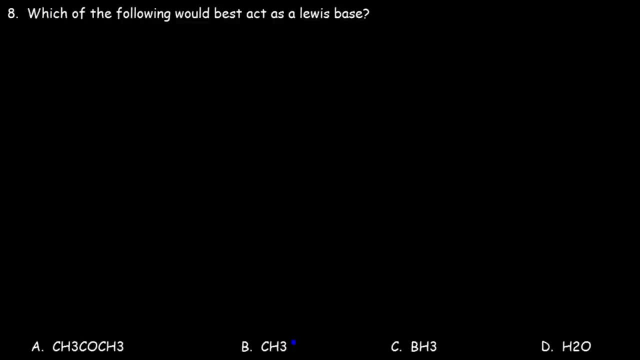 And then we can easily see which one's going to be the Lewis base. A Lewis base is a nucleophile. It's electron rich, It's full of electrons, Which means that it has a lot of lone pairs, and it may have a negative charge. 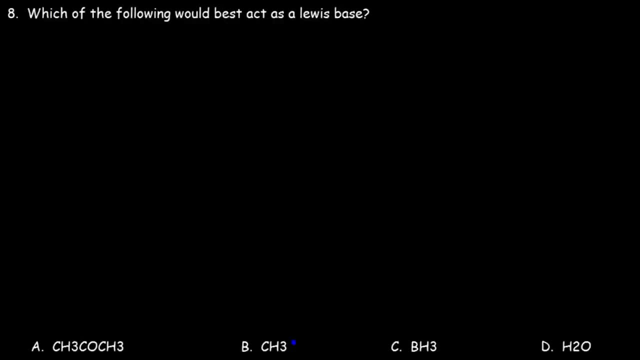 A Lewis base can donate a pair of electrons. Lewis acids, on the other hand, are electrophiles. They're electron poor, They're deficient in electrons And typically they may have a positive charge. But the most important thing you need to know, 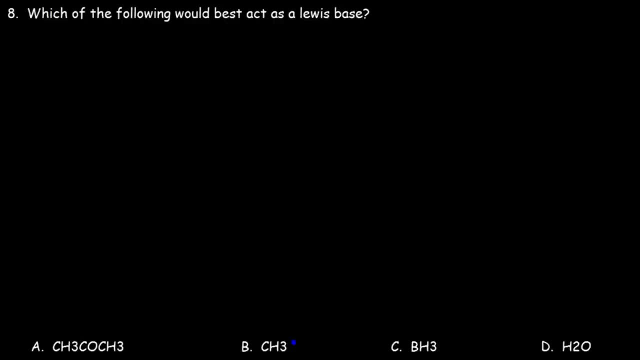 is that they have the ability to accept a pair of electrons. So let's look at answer choice A. Is it a Lewis base or is it a Lewis acid? Can it accept a pair of electrons Or will it donate a pair of electrons? 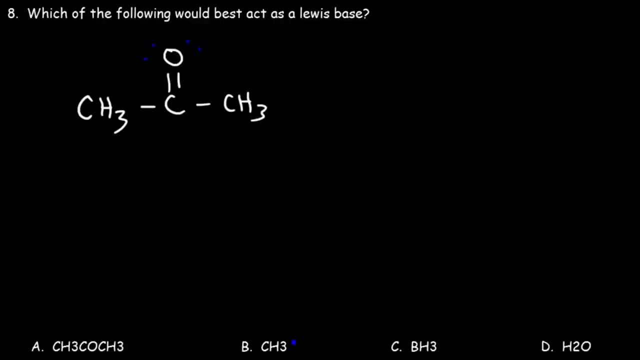 If we draw the resonance structure, notice that the carbon atom will have a positive charge. The oxygen now has a negative charge. So therefore the carbonyl group, which correlates to aldehydes and ketones. they're typically electrophilic. 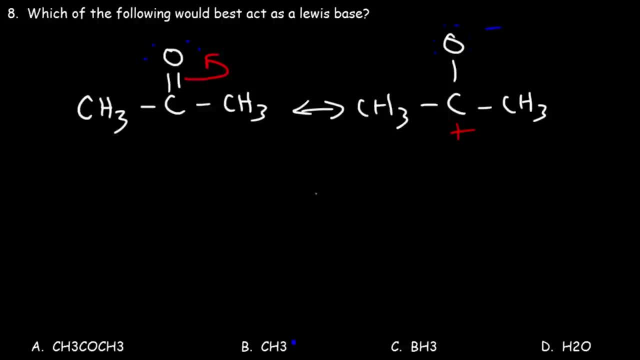 They tend to act as Lewis acids. Let's say, if we take a Lewis base like hydroxide, Hydroxide can donate a pair of electrons to the carbon, Which means that acetone and ketones and aldehydes are all electrophilics. 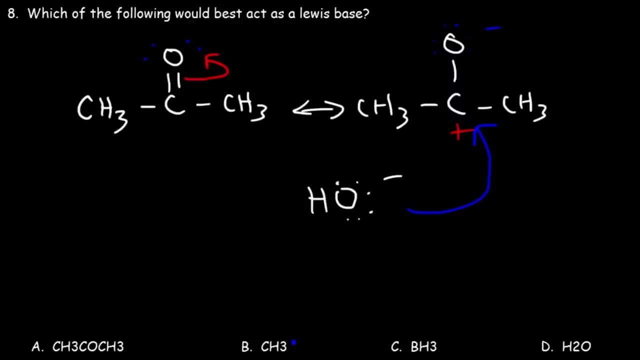 I mean electrophiles, Which means they're Lewis acids. So we can eliminate answer choice A. Now what about answer choice B? Is it a Lewis acid or is it a Lewis base, Or is it neither? Let's find out. 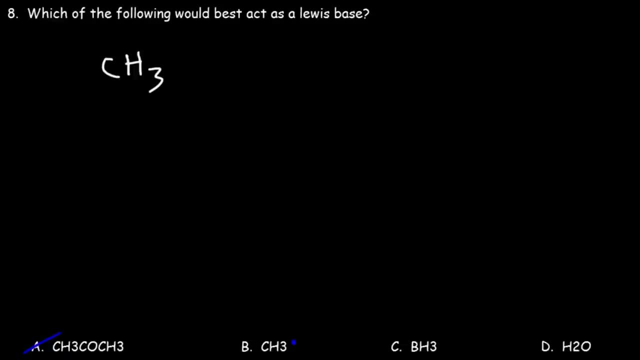 So the methyl radical has an unpaired electron. Since it doesn't have a pair of electrons, it cannot act as a Lewis base. For anything to act as a Lewis base, it has to donate a pair of electrons, Which means two electrons. 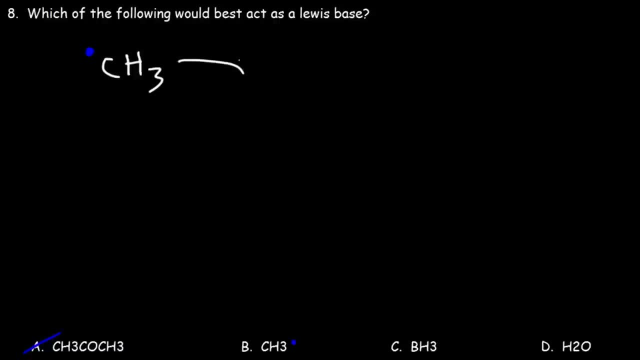 The radical only has one electron, So it can't donate two electrons. It just doesn't have it. Now, can the methyl radical accept a pair of electrons? So let's say, if we react with hydroxide, Can hydroxide donate a pair of electrons? 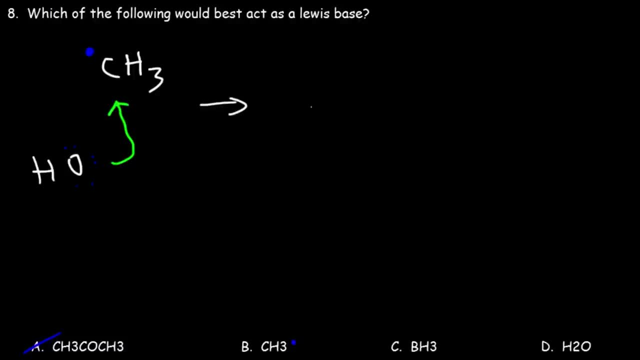 to it forming a bond. Let's say, if it did, This bond will be created And the oxygen, which had three lone pairs, now has two. The carbon still has the three hydrogens And it should still contain the radical or this unpaired electron. 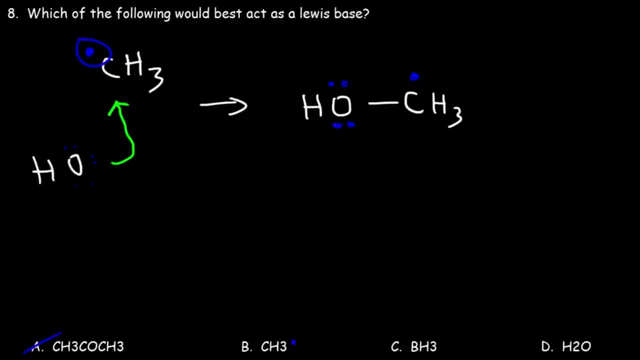 Notice that this structure is not possible. Carbon cannot have four bonds and at the same time have an unpaired electron. That would violate the octet rule and it's not possible. Carbon cannot have nine electrons, Which means that a radical cannot behave as a Lewis acid. 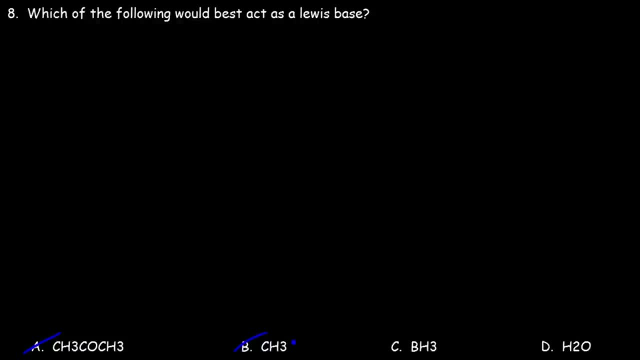 Nor can it behave as a Lewis base, Particularly this particular radical. Now what about BH3?? Is that a Lewis acid or is it a Lewis base? So we can see that boron doesn't have a lone pair, So it can't act as a Lewis base. 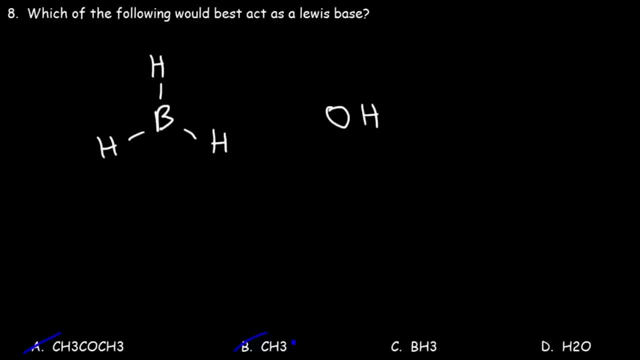 It can't donate a pair of electrons. However, it can act as a Lewis acid. It can accept a pair of electrons from hydroxide, And then what's going to happen is we're going to get this product. So in this example, 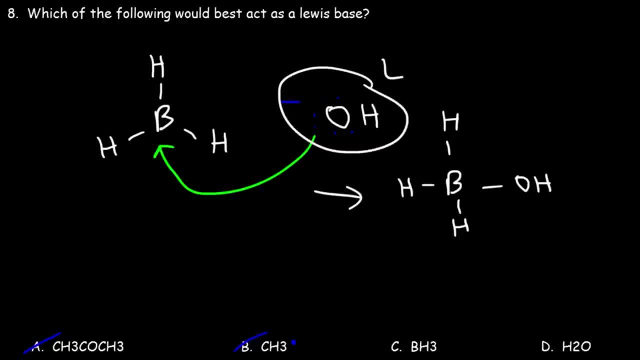 hydroxide, which donated the pair of electrons, is the Lewis base, or the nucleophile BH3, which accepted the pair of electrons, is the Lewis acid, also known as the electrophile. So, by default, the answer has to be water. And if we draw water, 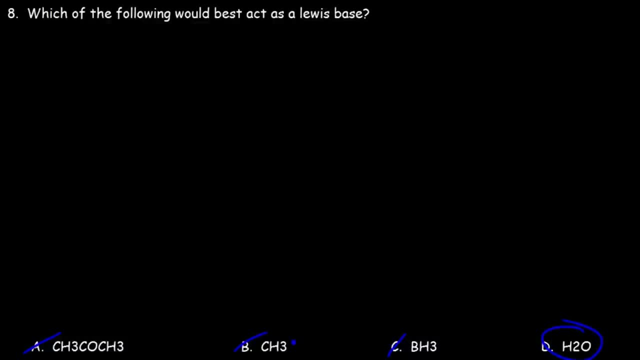 water has a lone pair. We can draw it like this: It has two lone pairs actually, And let's react it with BH3. So, like hydroxide, water can use one of its lone pairs and donate it towards the boron atom. 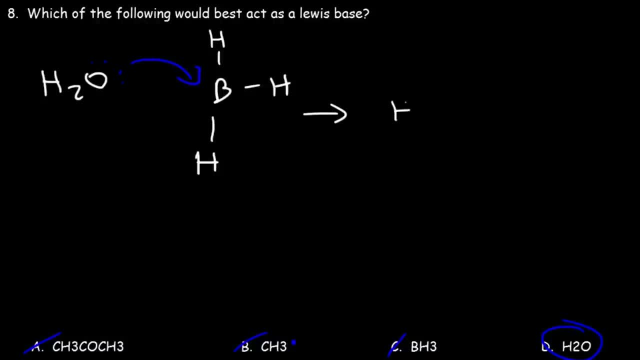 And so we're going to get a product that looks like this. So we're going to get boron. Boron is going to have a negative formal charge, Oxygen is going to have a positive formal charge, And so we can clearly see that. 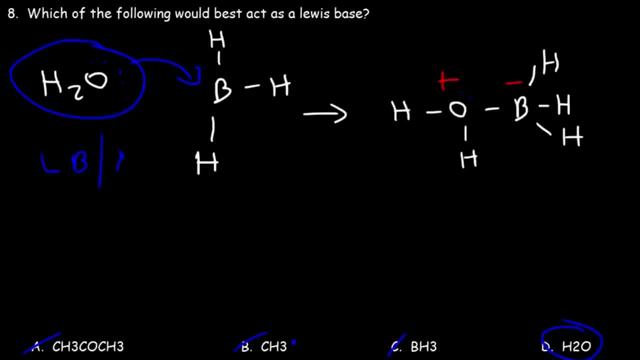 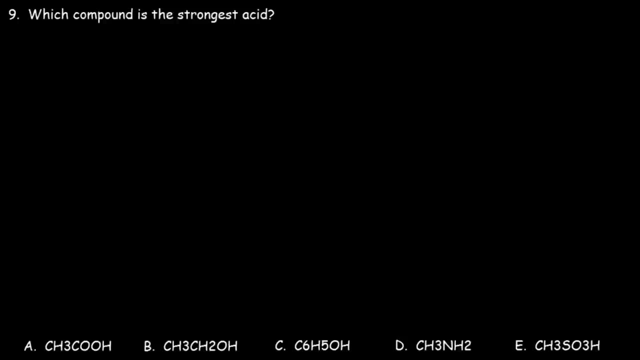 water is behaving as the Lewis base, which is the nucleophile. So D is the right answer. Number 9: Which compound is the strongest acid? So let's look at each answer choice. So for answer choice A, we have a carboxylic acid. 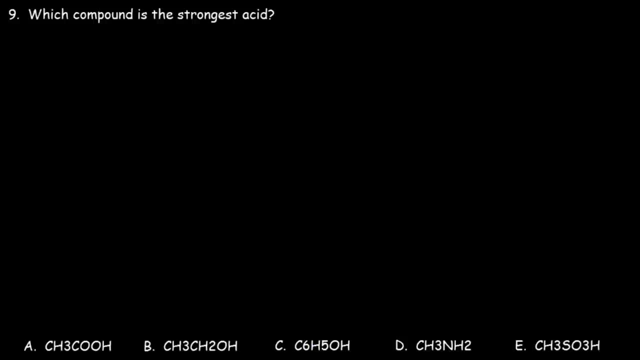 You can see the functional group COOH, And what you want to do is you want to be able to determine the pKa of each of these molecules. If you know the pKa, you can tell which one is the strongest acid As the pKa. 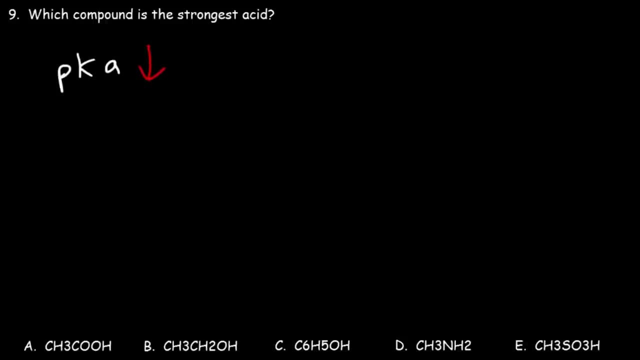 decreases, the strength of the acid increases. So the one with the lowest pKa is going to be the strongest acid. Carboxylic acid has a pKa of about 4 to 5.. Now answer choice B. we have an alcohol, which most alcohols have a pKa. roughly between 16 and 18.. In the case of ethanol, ethanol has a pKa of 15.9.. Answer choice C represents phenol. It has 6 carbons, 5 hydrogens and an OH group. Whenever you see C6H5. 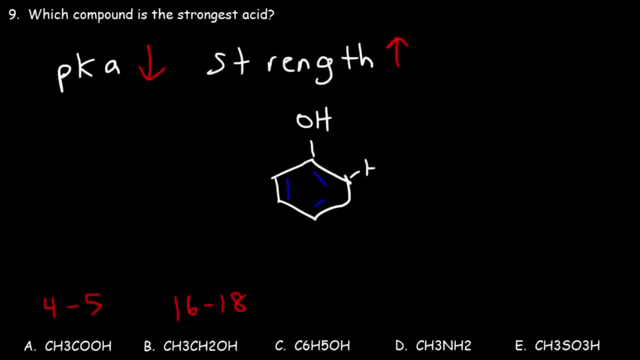 it's a benzene ring Attached to something else. Every carbon atom in a benzene ring has 5 hydrogen atoms. So C6H5 represents phenol, And phenol has a pKa of about 10.. Next we have methyl amine. 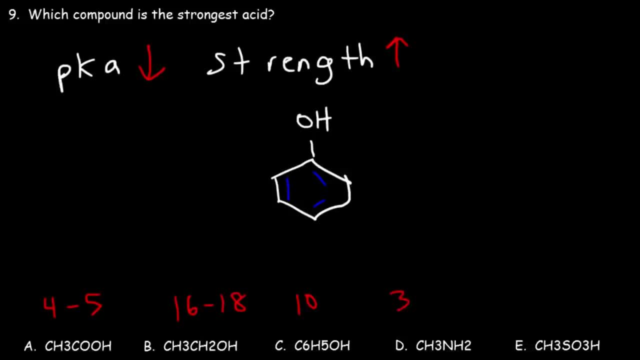 Most amines have a pKa roughly of about 35 to 40. And E is a sulfonic acid. Whenever you see an SO3H group, these acids are very strong. This particular acid has a pKa of about negative 2.. 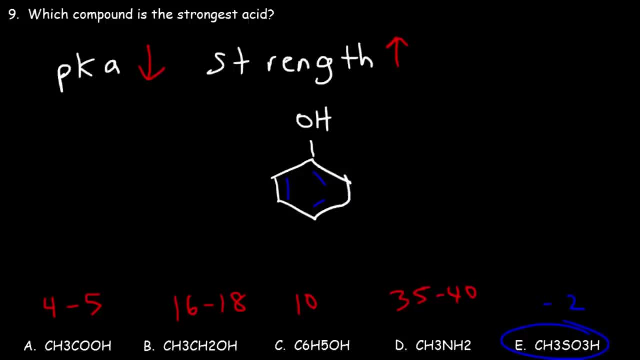 So the right answer is answer choice E. But now let's talk about it, Let's go over a few things. So how can we find out the answer if we don't know the pKa values? The first thing you want to compare is the element attached. 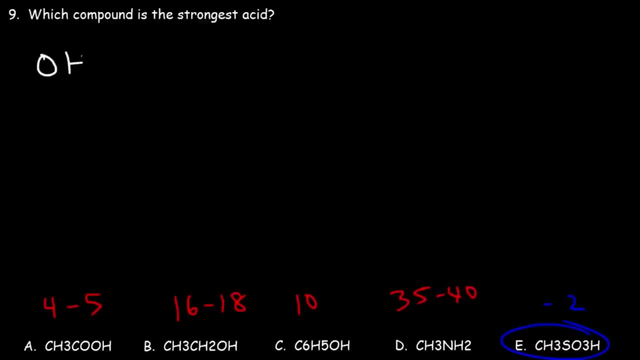 to the hydrogen atom. One of the most common examples is either an OH group or an NH2 group. The carboxylic acid has an OH group. The ethanol molecule and phenol has an OH group. Even a sulfonic acid has an OH group. The only one that's different is the NH2.. So whenever you have a different element attached to a hydrogen, you can use the trend found in a periodic table. Acid strength increases as you go to the right, due to increase in electronegativity, and as you go down. 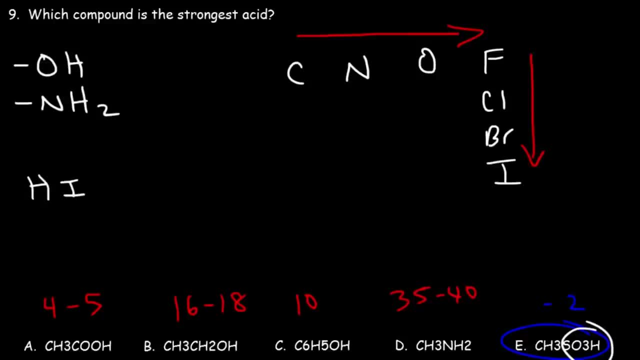 due to increase in size. So what this means is that HI is more acidic than HBr, which is more acidic than HCl, and that's more acidic than HF. HF is more acidic than water, and water is more acidic than NH3, which is more acidic than CH4.. 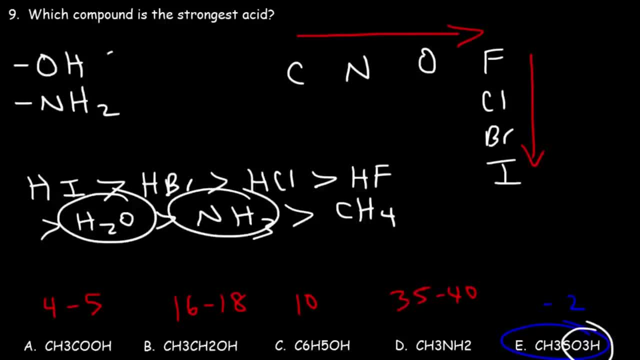 But let's focus on this. Water contains an OH bar and NH3 has an NH bond, So the OH bond is more acidic than the NH bond. if everything else is equal, assuming that they have the same charge, If one is positive and one is neutral. 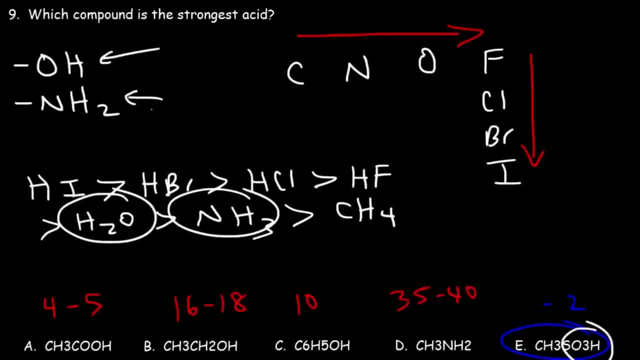 you can't use this comparison. Either they both have to be neutral or they both have to have a negative charge or both be positively charged. So the OH group is more acidic than the NH group, which means that D cannot be the strongest acid. So that's how you can eliminate D. without knowing the pKa values. Now let's look at B and C, because both of them contain an OH group. So ethanol has a pKa of 15.9 and phenol has a pKa of 10, and they both have an OH group attached to a carbon. 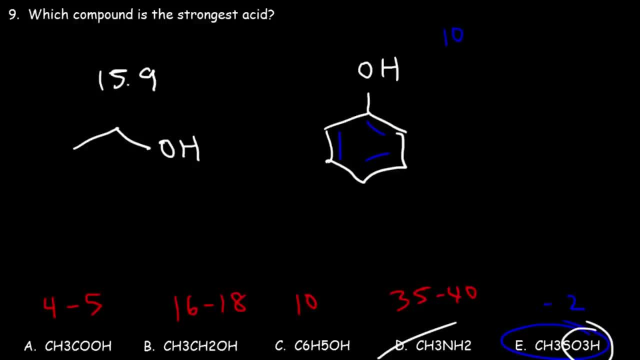 So why is phenol much more acidic than ethanol? The answer has to do with the stabilization of the conjugate base. The more stable the conjugate base is, the more acidic the conjugate acid will be. So that's the conjugate base of phenol. 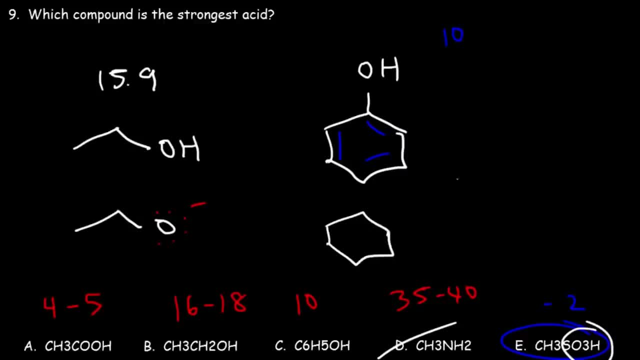 also known as ethoxide, And this is going to be the conjugate base of phenol, which is phenoxide. So the conjugate base of ethanol is ethoxide, in case I said that incorrectly, And the conjugate base of phenol is phenoxide. 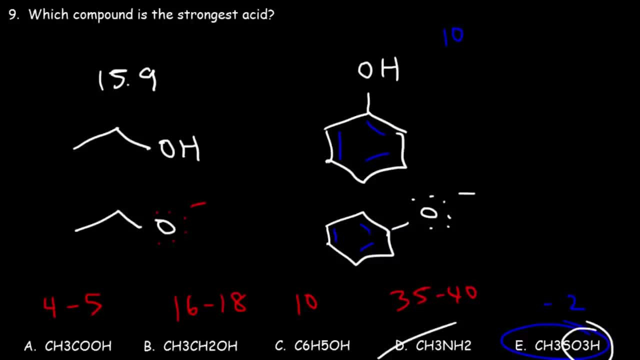 So notice that the negative charge on phenoxide is not localized, It's delocalized. It can move around. We can draw a resonance structure, take a lone pair, form a double bond and push the negative charge here, Because the negative charge can move about the ring. 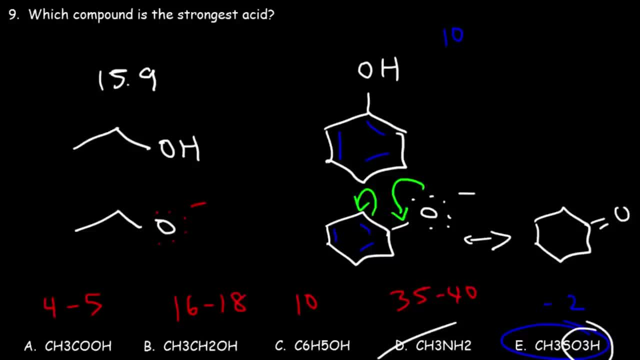 the conjugate base is more stable. And when you have a more stable conjugate base you're going to have a stronger conjugate acid. So the negative charge is shared between the oxygen atom and three other carbon atoms. The negative charge can jump every two carbon atoms so it can move. to these other positions indicated in red. So that's why phenol is more acidic than ethanol. It's due to the resonance stabilization of the conjugate base. So we can eliminate answer choice B, since C is more acidic than B. Now let's compare. 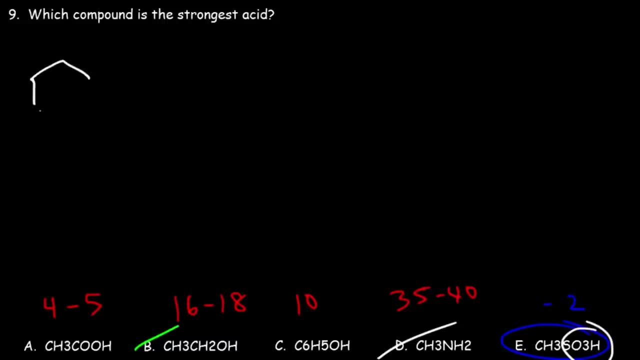 A with C. So let's start with the conjugate base of phenol, Let's redraw it, And if we draw the resonance structure, we know that this electron, or those pair of electrons, can move here, pushing a negative charge on the carbon atom. 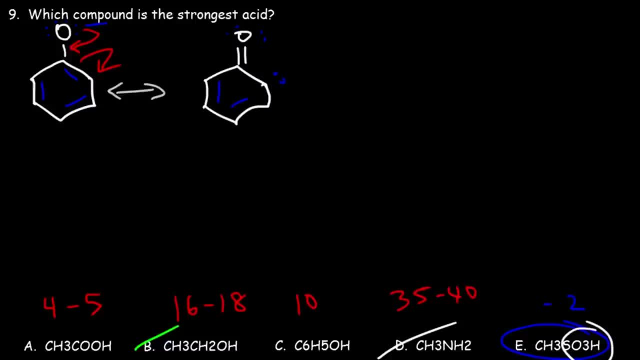 And that will give us this particular resonance form And we can draw two other resonance forms So this lone pair can move here and push the other two electrons on the next adjacent carbon. So now the negative charge is in that position. So the negative charge, 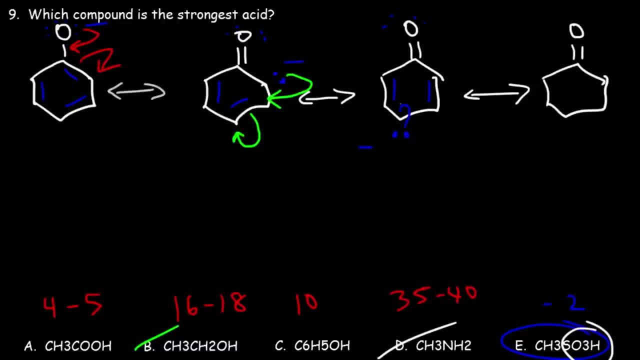 is going to keep jumping two carbons away. So now we can draw another resonance form. So, as you can see, the phenoxide ion has a total of four resonance forms. The negative charge can be placed on one oxygen atom or three carbon atoms. 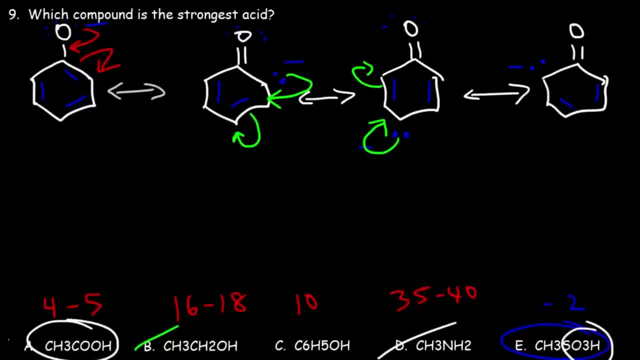 Now let's draw the conjugate base of acetic acid, which is known as acetate, And let's draw the resonance form. To draw the conjugate base, all you need to do is take off the hydrogen. Now this negative charge can move to the other oxygen atom. 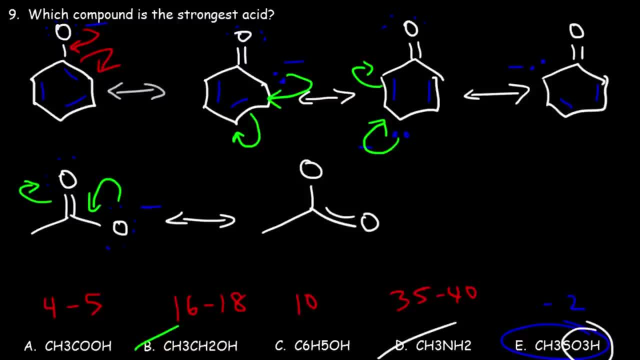 Giving us these two resonance forms. So here's a question for you: Why is it that phenol is more acidic than acetic acid? I mean, I take that back. Why is it that acetic acid is more acidic than phenol if an oxide ion? 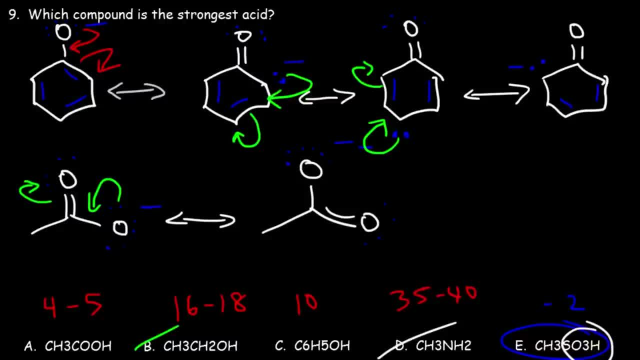 has more resonance structures, Because typically the more resonance forms that you have would indicate a more stable conjugate base, which means a stronger acid. But we don't see that Acetic acid is stronger And it only has two resonance forms. when we draw the conjugate base of acetic acid, 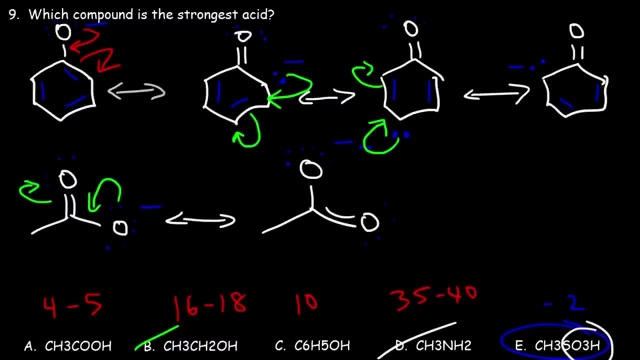 So why is it that acetic acid is a stronger acid when it should be phenol, if we look at the number of resonance structures? So not only should you look at the number of resonance structures, but you should look at where the negative charge is being placed. 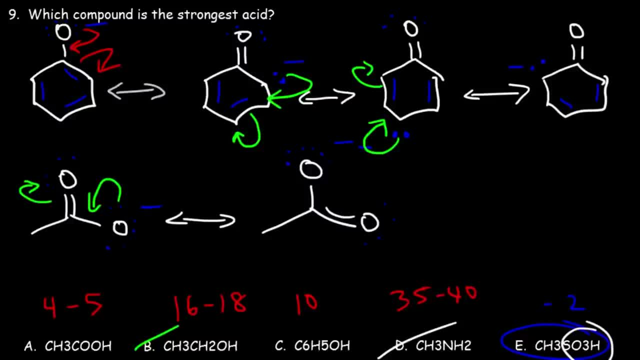 on what type of atom Is it better to put a negative charge? on an oxygen atom or on a carbon atom? Oxygen is more electronegative than carbon. Electronegativity increases towards the right, So it's a lot more stable to put a negative charge. 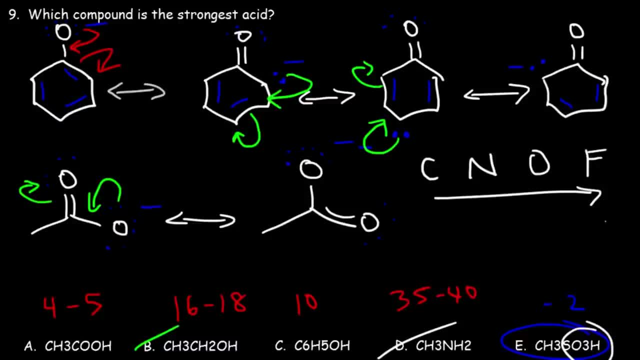 on an oxygen atom than a carbon atom. So if we look at the first resonance structure, the negative charge is placed on the oxygen atom, So let's assume that those two are equivalent. Now, in the second resonance form of the acetate ion, the negative charge, 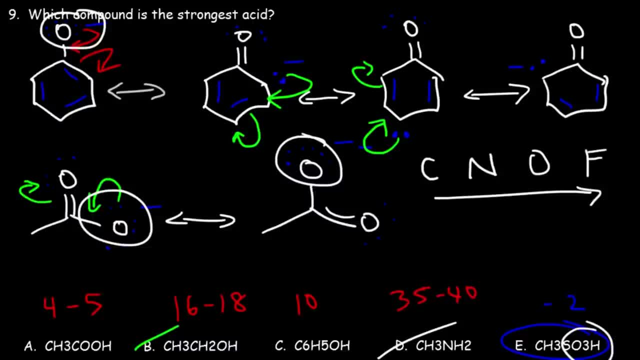 is also on an oxygen atom, But in the remaining three forms of the phenoxide ion the negative charge is on a carbon atom. It turns out that putting a negative charge on a single oxygen atom is more stable than putting a negative charge on two carbon atoms, Because carbon 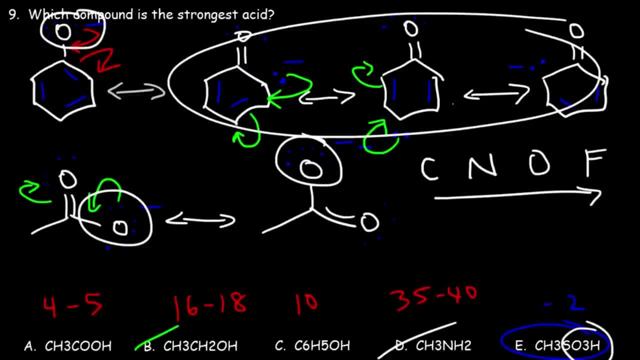 really doesn't want to have a negative charge. Oxygen can stabilize it better, And so that's why acetic acid is more stable or more acidic than phenol. It's because you have a negative charge on two oxygen atoms, as opposed to one oxygen atom in the case of phenol. 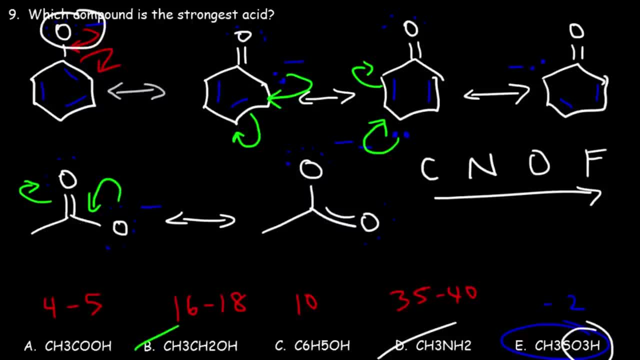 So putting a negative charge on a second oxygen atom increases the stability by a huge amount. as you can see, based on the number, Acetic acid is much more acidic than phenol. Now, this case is apparent if you compare answer choice A and answer choice E. 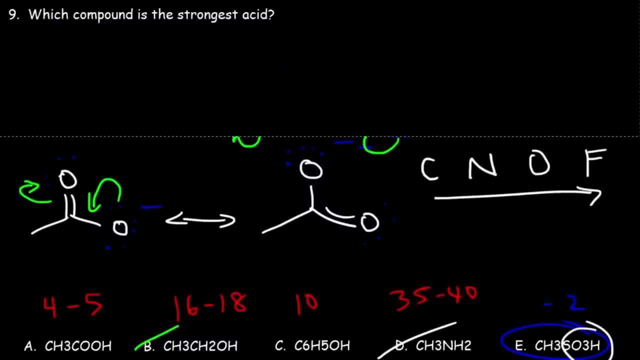 So let me get rid of this stuff. So let's draw the conjugate base of methane sulfonic acid Instead of drawing a methyl group. I'm just going to represent it with an R group. So we need to take off the hydrogen Now. if we draw the resonance form, 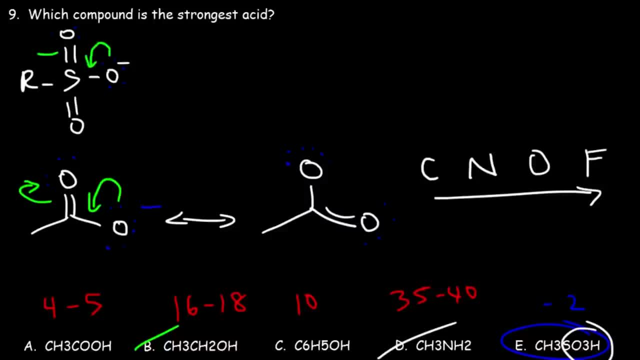 we can take a lone pair and form a double bond, causing the negative charge to move on the other oxygen atom. So we can get this resonance form And to get the next one we can use the lone pair, form a double bond, breaking the other pi bond. 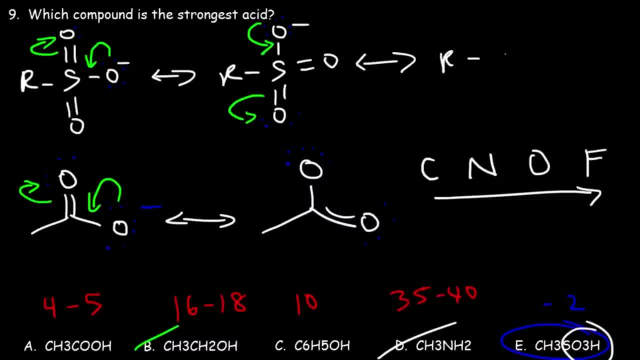 So, as you can see, because there's three oxygens, there's three different resonance forms that we can draw for the sulfonic acid. So the negative charge is shared between three oxygen atoms, as opposed to two in the case of acetic acid, And we can see that pKa2 is. 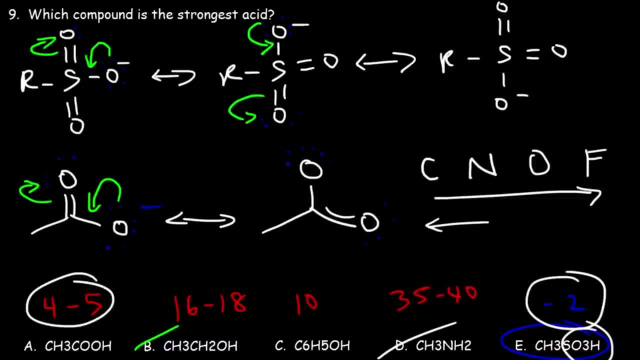 significant. So that's why methane sulfonic acid is the most acidic one. It's because first you're placing the negative charge on an atom that can stabilize it or that can take the negative charge, like oxygen And the quantity of oxygen atoms. there's three resonance forms. 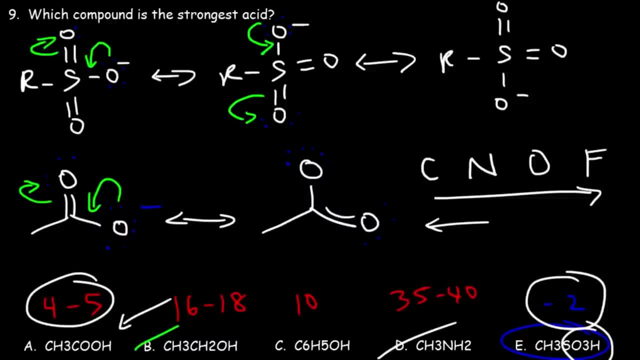 that negative charge can be shared between three oxygen atoms, as opposed to two in the case of acetic acid or as opposed to one in the case of phenol. So the more resonance structures that you have and if you can place it on an atom that can stabilize the negative charge, 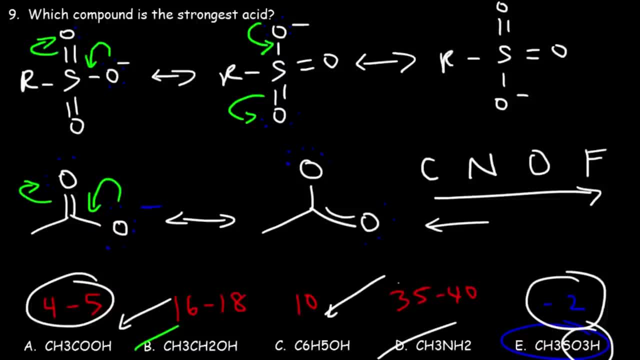 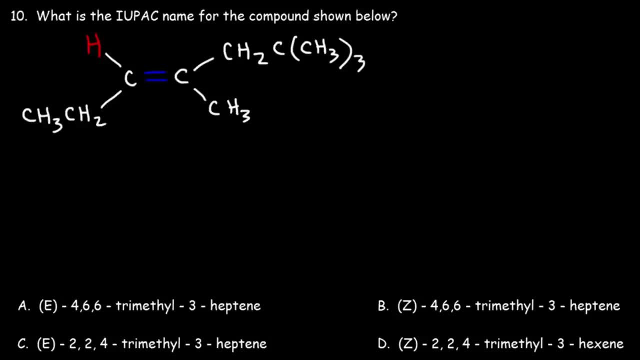 that will increase the stability of the conjugate base, making the conjugate acid more acidic. Number 10: What is the IUPAC name for the compound shown below? So take a minute and work on this problem. So what do you think we should do? 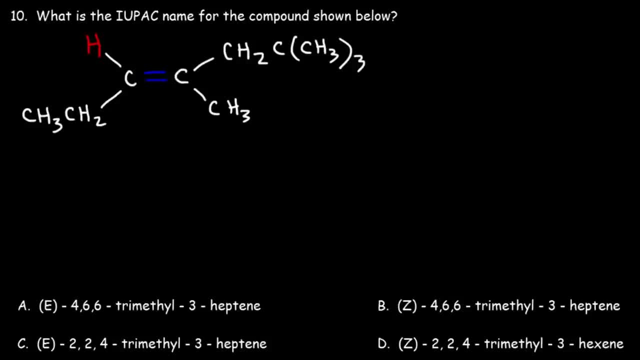 first. The first thing that I would recommend doing is to draw a length structure into a line structure. So we have a CH3 and a CH2. that's two carbons right there once you draw a single line, and then we have a carbon double bonded. 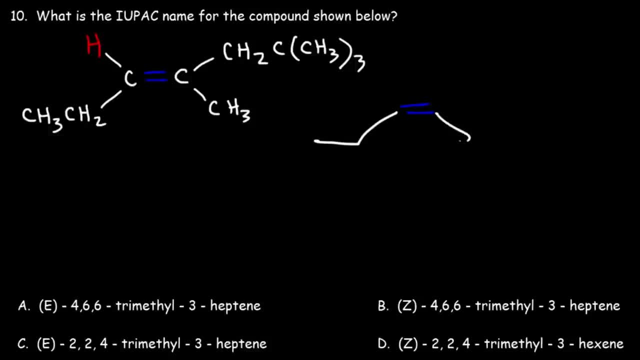 to another carbon, and then we have a CH3 on the bottom, a CH2 on the top, and then a carbon which is attached to three methyl groups, and then let's draw the hydrogen as well. So that's the line structure. Now the next thing we need to do is identify. 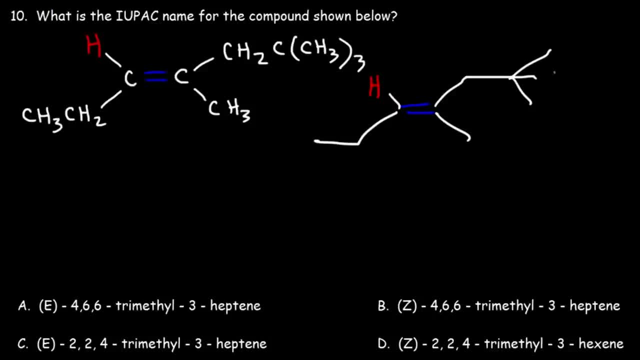 the longest chain. So if we start from this end, this is going to be carbon 1,, 2, 3, 4, 5, 6, 7, So it's going to be a heptane derivative as opposed to. 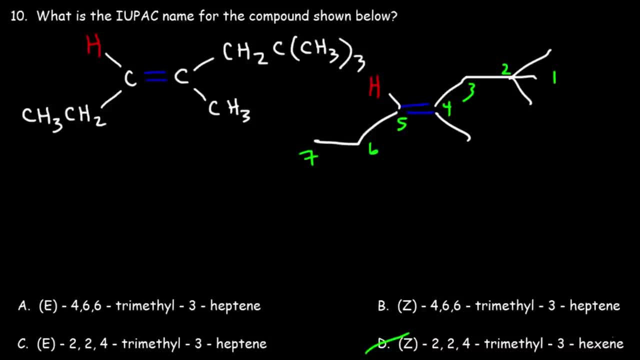 a hexane derivative, which means we can eliminate D. Hexene indicates that there's six carbon atoms in the longest chain, but we can see that there's seven. Now we need to know the correct, the right direction in which to count it. Should we count it from left to right or right to left? 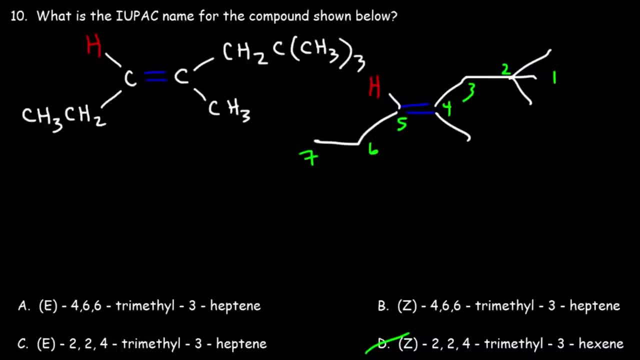 As we count it from right to left, notice that the double bond is between carbons 4 and 5. We need to give the double bond priority. Let's count it in the other direction. So let's say this is carbon 1, 2,, 3, 4. 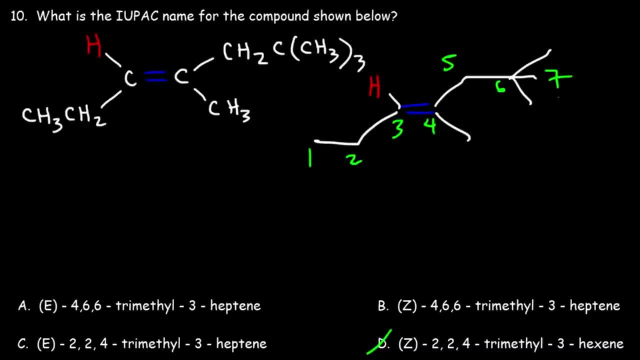 5,, 6, and 7. Notice that, if we count it from left to right, the double bond is now between 3 and 4 instead of 4 and 5, which is better. So now let's go ahead and name it. Notice that we have a methyl group. 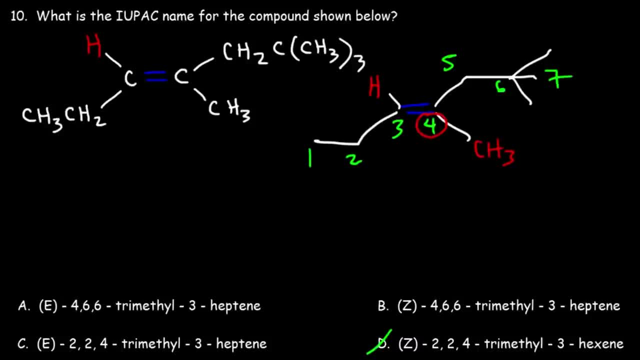 on carbon 4 and we have two methyl groups attached to carbon 6, So it's 4, 6, 6 as opposed to 2, 2, 4. Now we're between A and B. Everything looks the same, except one is E. 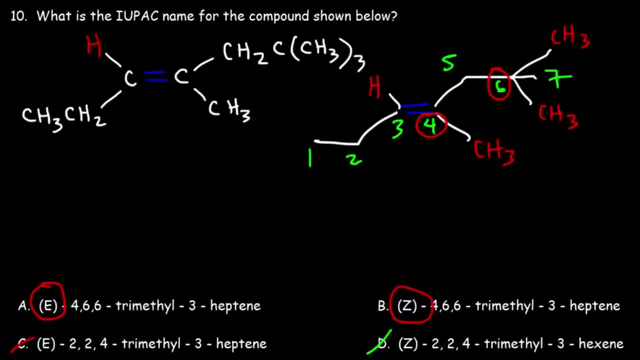 and the other is Z. We need to know which isomer do we have. Is it E or is it Z? So we need to determine which group has more priority. So on the left side, is it the hydrogen or the ethyl group? The ethyl group. 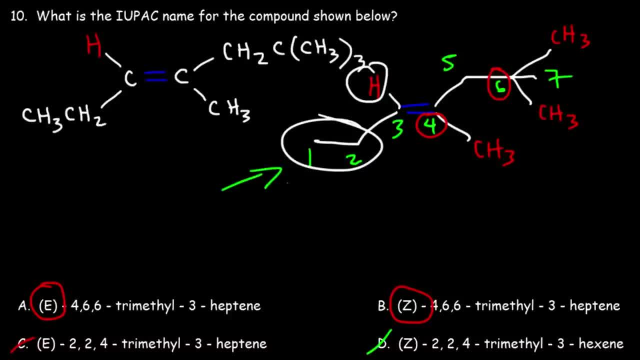 has more priority than the hydrogen. Carbon has a higher atomic number than hydrogen. Now, what about on the right side? Is it the methyl, or is it these groups of carbons that we see here? If you have a chain of carbons, that's the. 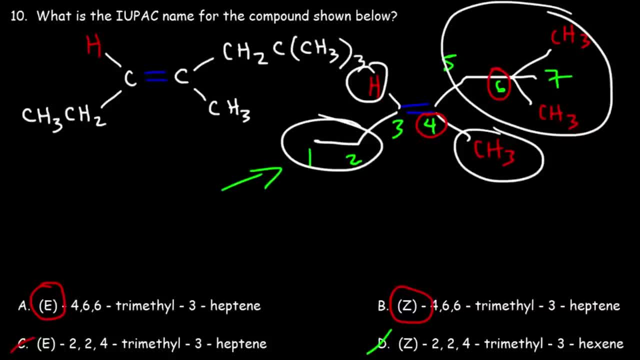 that's going to have more priority than a single carbon atom. If you analyze this, this is a methyl carbon compared to a secondary carbon. A secondary carbon has more priority than the methyl carbon, So the highest priority groups are on opposite sides. When they are on opposite sides, 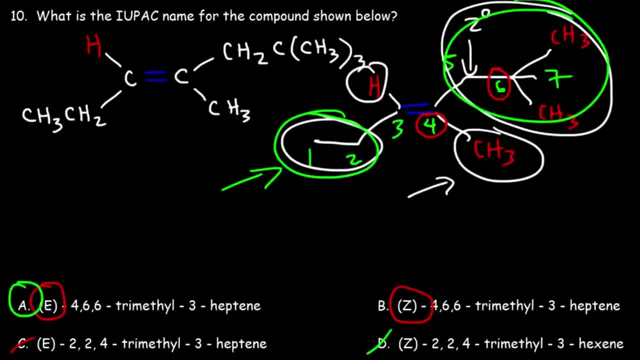 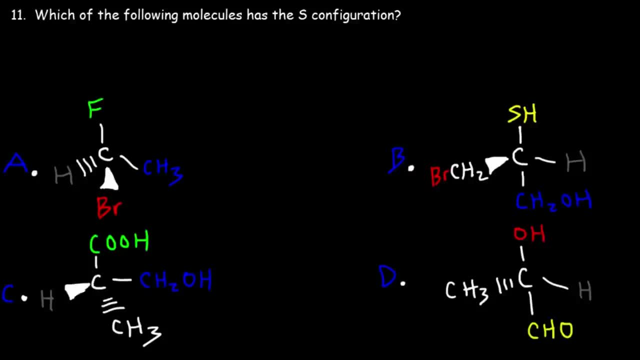 you have the E isomer. If they are on the same side, you have the Z isomer. So answer choice A is the right answer. Number 11: Which of the following molecules has the S configuration? A, B, C or D? Well, let's find out. 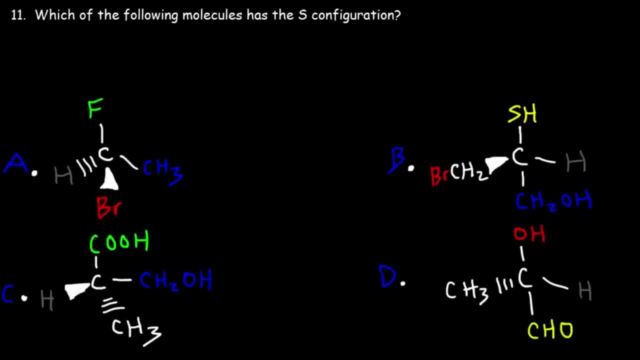 Let's start with A. So first we need to rank each group based on their atomic numbers. Bromine has the highest atomic number, so we're going to give it a score value of 1. It has the highest priority. Next, Fluorine has the second highest atomic number. 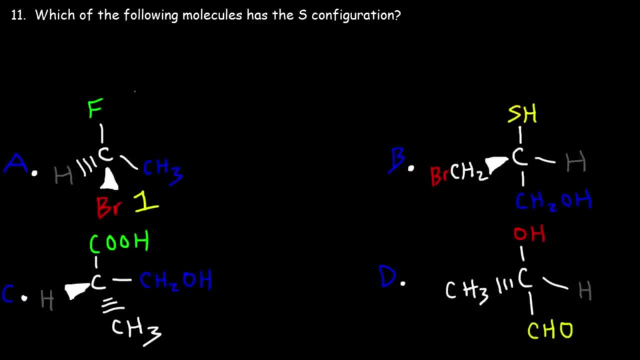 and then it's carbon. So fluorine is going to be group number 2, Carbon is 3 and H is number 4. So what you do is you count it from 1, 2, and 3, Ignore 4, So going in the direction starting from 1. 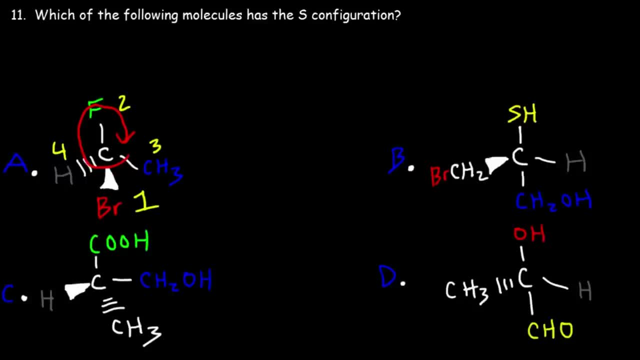 to 2 to 3. Notice that it's rotating in the clockwise direction, which is R. Now, before you count it, you need to make sure that group number 4 is in the back, which it is. So A is not the answer because it has the R configuration. 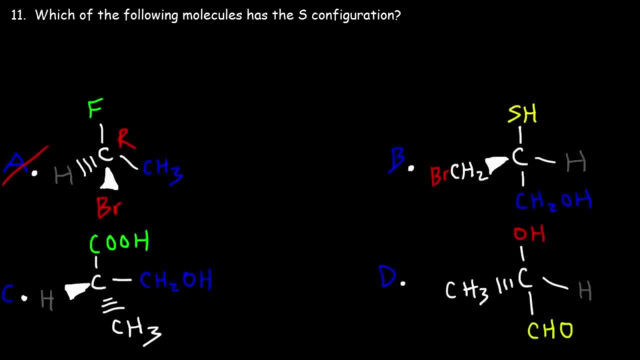 So we can eliminate answer choice A. Now let's move on to B. So we can see that it's relatively easy to assign the configuration whenever H is in the back. You just simply have to count it in a direction starting from 1 to 2 to 3. 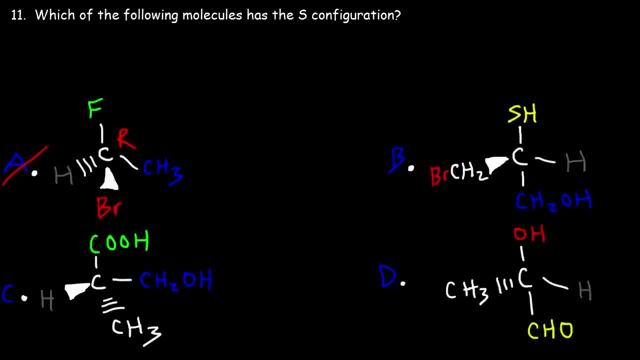 Now, what about when H is in the front? Well, let's do everything that we did. We know H is going to be number 4. Now, between these three groups, they all start with a carbon, But the CH3 doesn't have an oxygen, so this is going to be group number 3. 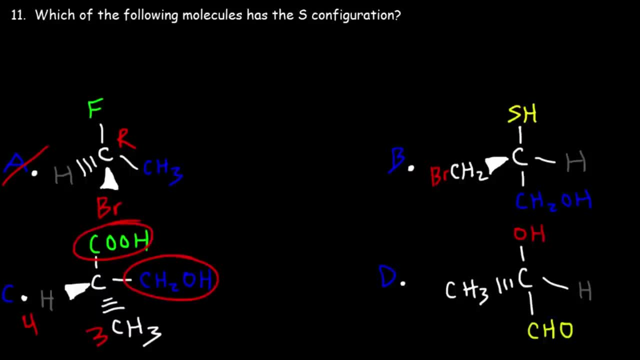 Between these two, which one will have a higher priority? Well, the carboxylic acid has more oxygens than the alcohol, So therefore, that's going to be group number 1 and this is going to be group number 2. So what you need to do is count it in a direction. 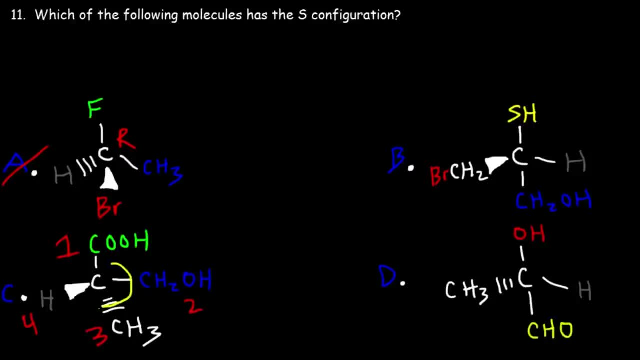 from 1 to 2 to 3, But because H is in the front, you need to reverse it As we go from 1 to 2 to 3. this is clockwise, But because H is in the front and we want it to be in the back, 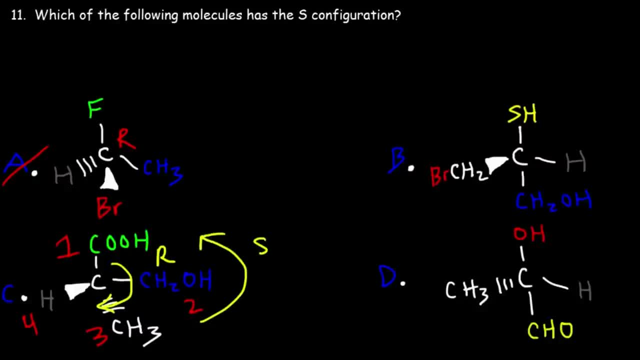 we need to reverse it. So we get S, Which means that C is the correct answer. So you always want group number 4 to be in the back. Now we know that B and D has to be R, But for the sake of practice, let's go ahead and work through those examples. 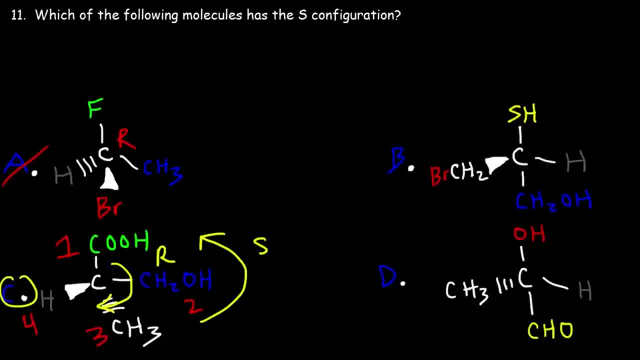 Let's prove that it's R Now in B. Group number 4 is not in the back. So what do you do in a situation like that? Well, Let's find out. So we know hydrogen is going to be group number 4, But which one is group number 1?? 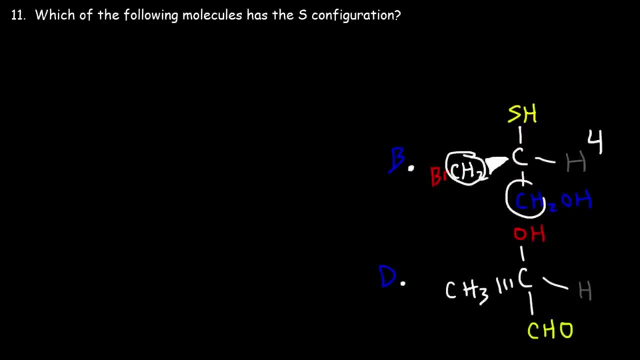 So notice that we have a carbon atom, a carbon atom and a sulfur. You need to compare the first atom that's attached to the center- carbon atom- before you look at the second atom. So you can't look at bromine yet, You have to focus on the CH2. 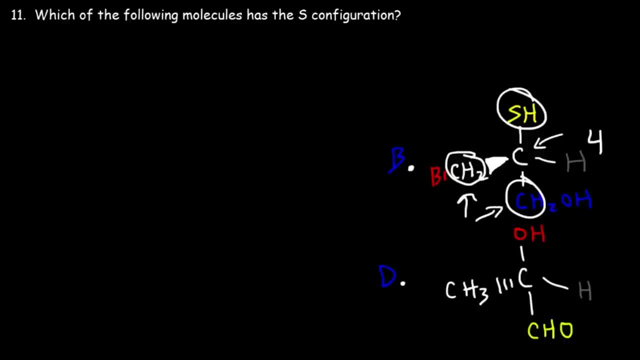 Sulfur has a higher atomic number than both of these carbon atoms. So therefore sulfur, or the SH group, is group number 1, it has the highest priority. Now. these two carbon atoms are similar, so let's move on to the second atom, relative to the chiral carbon. 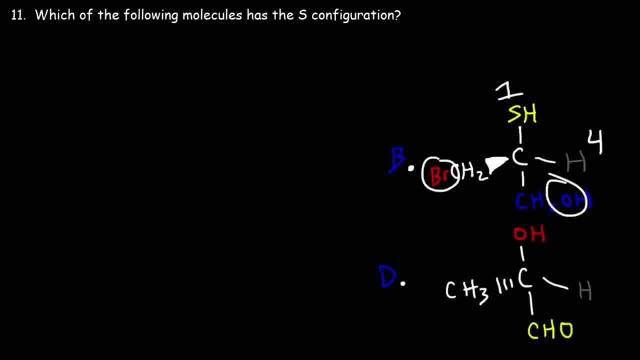 and let's see if there's a difference. Bromine has a higher atomic number than oxygen, So therefore, this is going to be group number 2 or group number 3. Now there's a method that you can use if you don't have one of those ball and stick models. 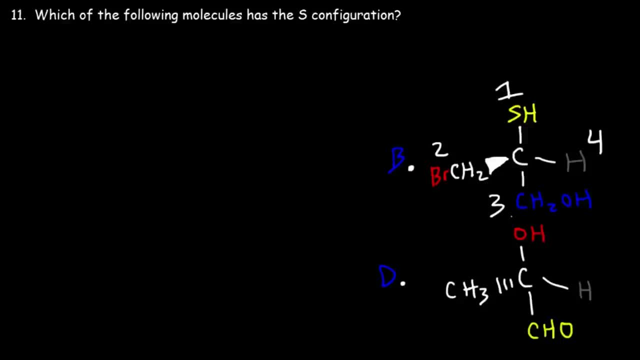 This is a method that I use to quickly determine if it's going to be R or S. If you have a group that's in the front or in the back, put it in a circle. So group number 2 is in the front, which means that we're going to have to. 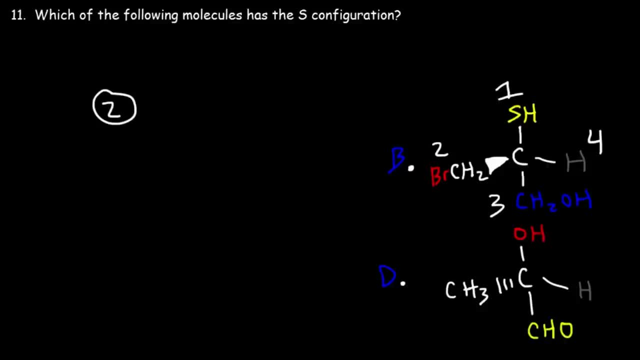 reverse our answer to get the right answer. when we assign R or S configuration, At the top we have number 1, To the right of number 1 we have a 4 and to the left of number 1 we have the 3. So you want to put the three numbers. 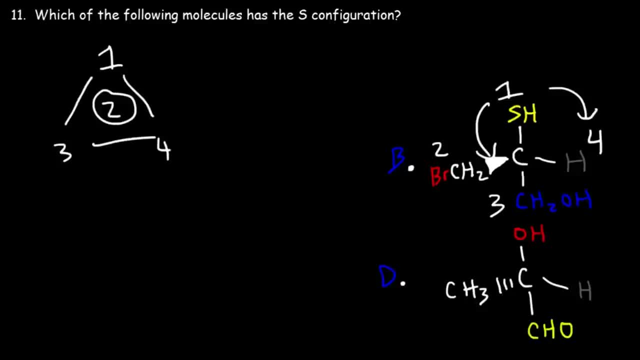 similar in the form of a triangle around the number that's in the circle. Now, currently group number 1 is on top. We want to rotate the molecule such that group number 4 is on top. So let's rotate it counterclockwise. So now 4 is going to be on the top. 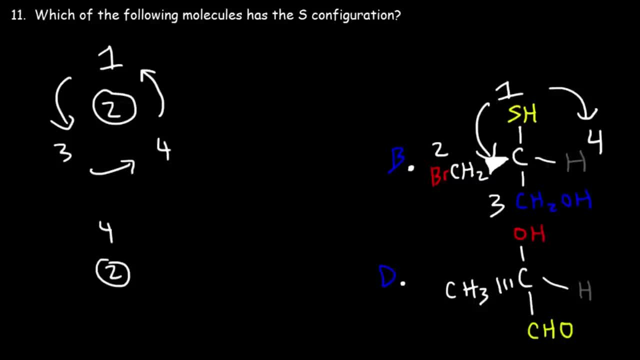 2 is still in the circle And keep in mind, the stuff that's in the circle represents what's in front. Now 1 is going to be to the left and 3 has moved to the right. Now what we're going to do is we're going to flip the molecule. 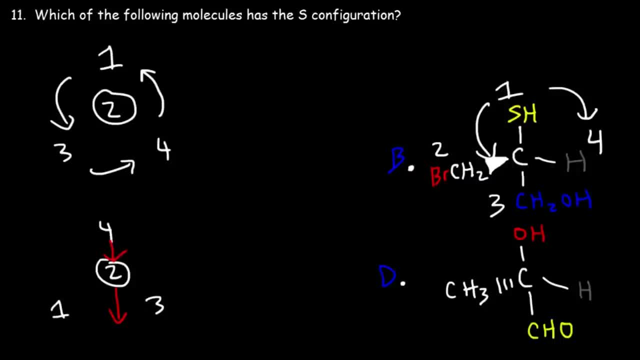 We're going to flip it in such a way that number 4 is going to kick out number 2, So 4 is going to be in the front. 1 and 3 are going to flip, So 4 is in the circle. 2 has been kicked out. 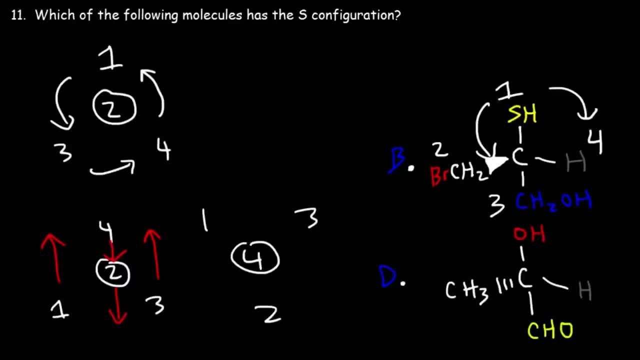 and 1 and 3 are at the top now. Now we can count it from 1 to 2 to 3. So right now this appears to be S counterclockwise, But because number 4 is in the front, we need to reverse it. 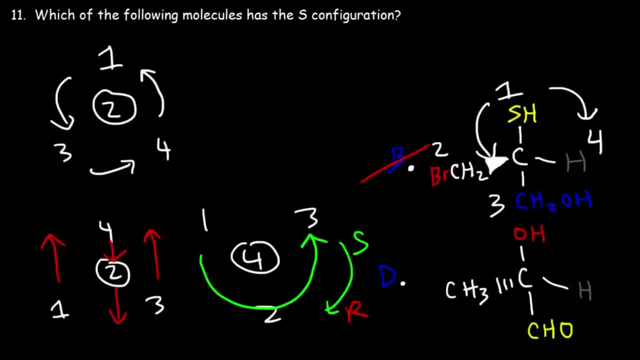 So the answer is R, Which means B is not an answer. Now what about the last one, D? What we're looking for is S, and we know that C is the right answer. So let's prove that answer. choice D has the R configuration. Feel free to try this method yourself. 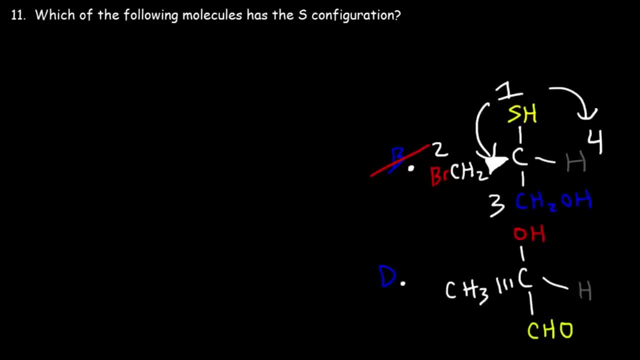 Go ahead and pause the video and try it. So first let's identify the 4 groups that we have. We know the hydrogen is number 4. Now, if we compare the carbon atoms with the oxygen, oxygen has a higher atomic number, so the OH group is number 1. 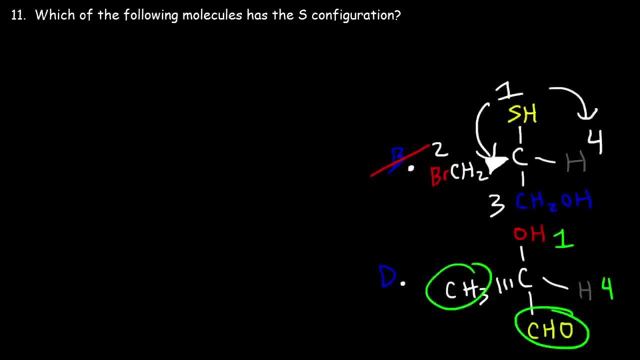 Now comparing the methyl group and the aldehyde group. The aldehyde group has an oxygen, so it's going to be the methyl group. So this is going to be number 2. The methyl group is number 3, So group number 3 is in the back. 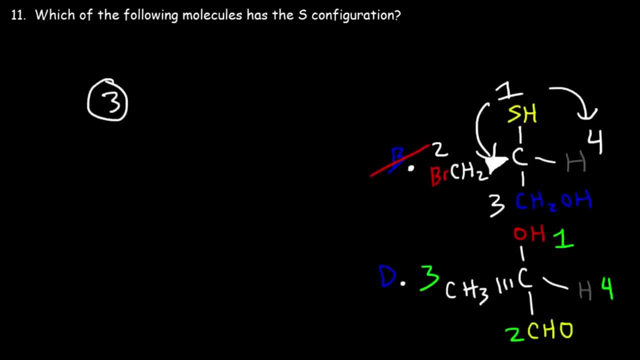 Let's put that in a circle, So for this one we don't have to reverse it, because what's inside the circle is already in the back. We want group number 4 to be in the back of the molecule Right now. group number 1 is on top. 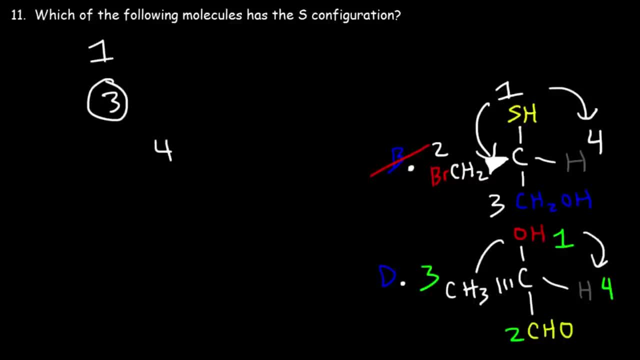 So let's put that here: 4 is to the right of number 2, 2 is to the left. So let's rotate the molecule counterclockwise. We want 4 to be on top So we can kick out 3. So now we're going to flip the molecule. 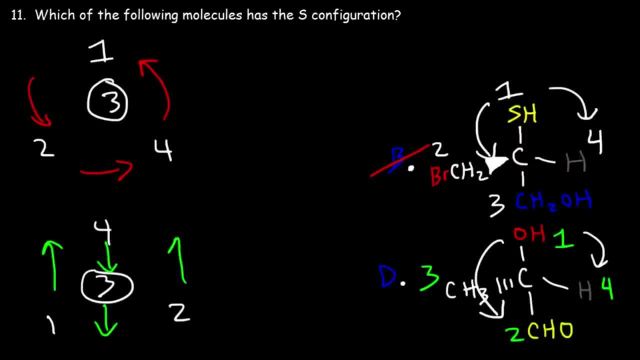 such that 4 kicks out 3, and 1 and 2 are going to flip to the top. So it's going to be 1, 2, 4 in the center, 3 below. So keep in mind: what's in the circle represents what's in the back. 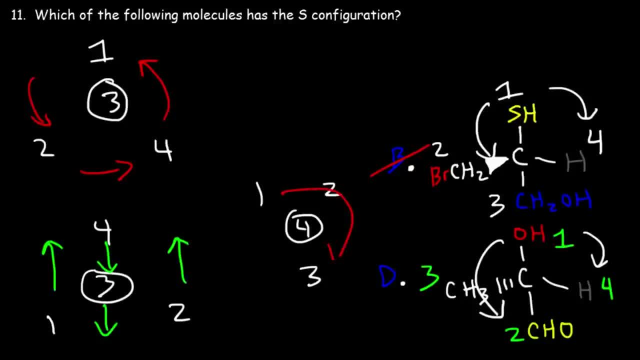 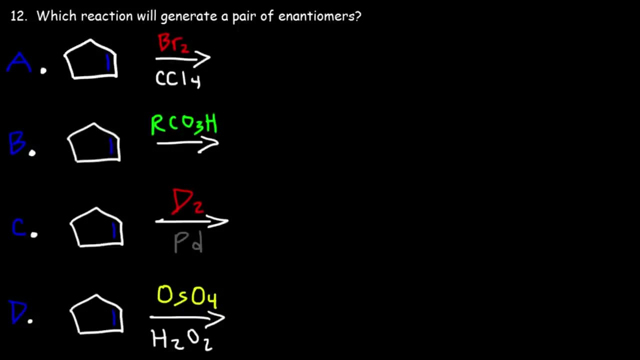 So we just got to count it from 1,, 2 to 3. So this is the R configuration. So therefore, only answer choice C has the S configuration. So answer choice C is the right answer. Number 12: Which reaction will generate a pair of enantiomers? 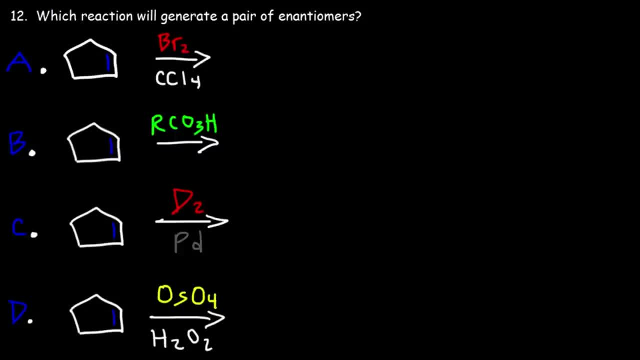 What do you think the answer is going to be? Well, let's start with D. If we combine an alkene with osmium tetroxide and H2O2 hydrogen peroxide, we're going to get 2 alcohol functional groups on the same side. 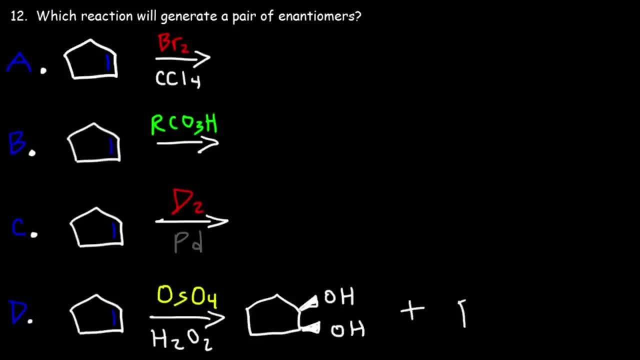 basically with syn addition, Now we can get 2 in the front and we can get 2 in the back. So these 2 molecules are they a pair of enantiomers or is it a single mesoproduct? It turns out that these are the same. 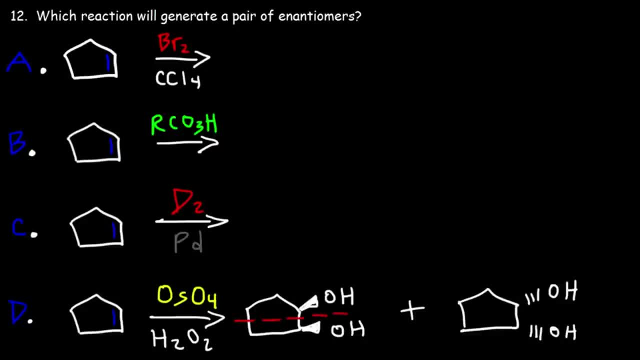 as hydrogen. Notice the symmetry. Even if the chiral center has changed configuration, If there is a line of symmetry, it will not be a pair of enantiomers. Instead we have a mesoproduct, Which means these 2 compounds are identical. So therefore, D is eliminated. 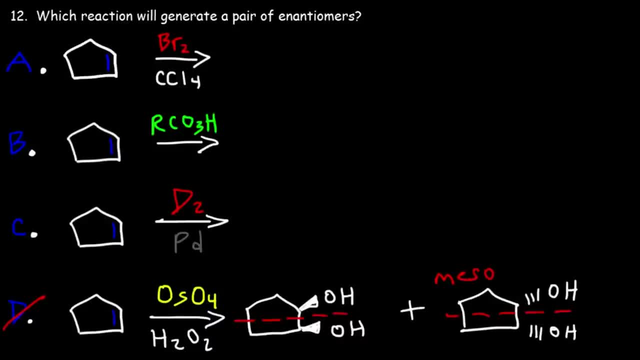 That's a mesoproduct. Now what about answer choice C Deuterium works the same way as hydrogen. Deuterium: will add across a double bond, turning it into a single bond, and the reaction proceeds via syn addition, Which means the 2 deuterium atoms. 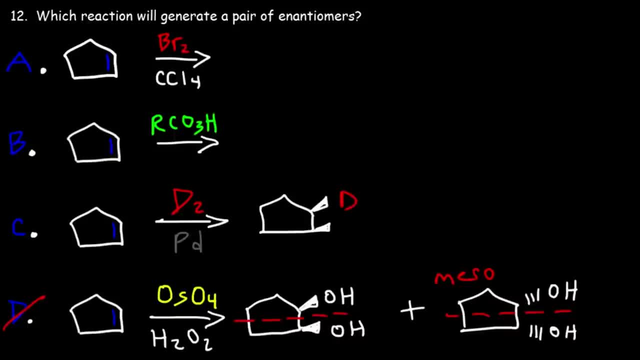 will be on the same side, So therefore this will generate a mesoproduct as well. So you get a single product. So answer choice C is eliminated. Now let's move on to B. If we combine an alkene with a peroxy acid, It could be RCO3H. 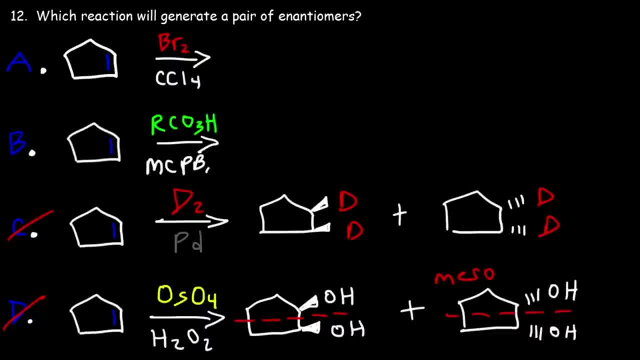 Another peroxy acid you might see is MCPBA. Basically they do the same thing. If we put these 2 together, we're going to get an epoxide. Now the epoxide reaction works with syn addition, Which means that it's on the same side. So we can write it like this: 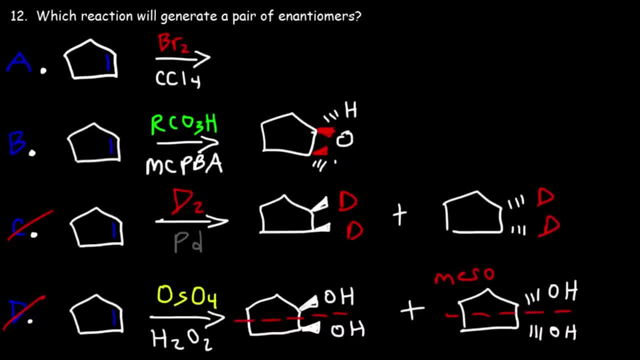 This is one way we can draw the product. We can also draw it like this as well. So, as you can see, There is a line of symmetry, And so it can't be a pair of enantiomers. if there's a line of symmetry, So this too. 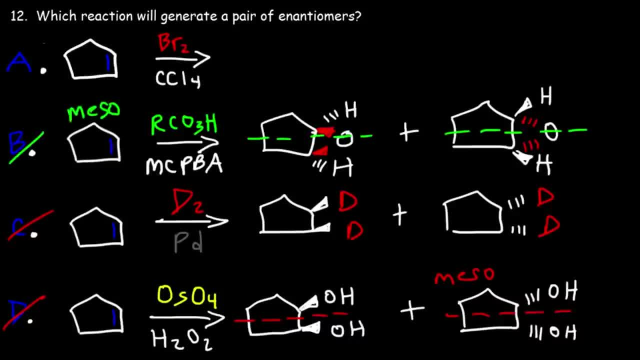 generates a mesoproduct, So B is eliminated, Which means A has to be the answer. Bromine adds across the double bond via anti-addition, And so the products will look like this. Notice that all chiral centers have been reversed in the two products, And also that we do not have a line of symmetry. 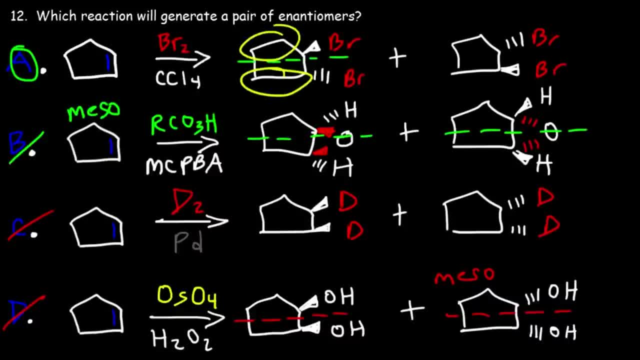 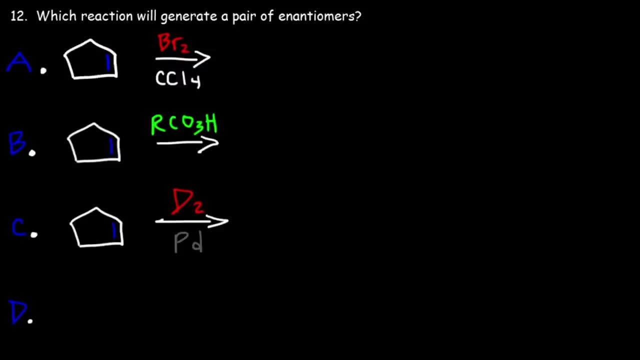 So, if you look at it carefully, This side is the same as that side And these two Br's are not the same. One is in the front And the other is in the back. Now you might be thinking: Well, there's two carbons here, Only one carbon here. 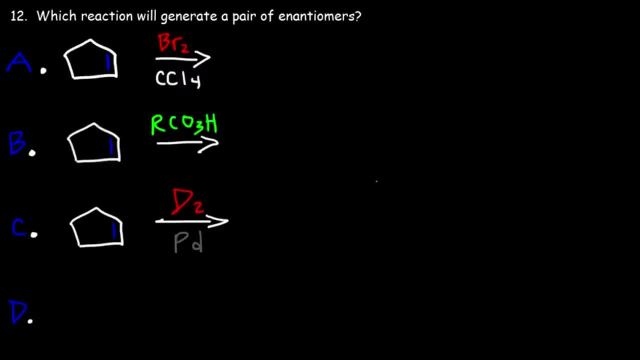 But if you draw it like carefully, Let's say If we draw it this way, The line of symmetry really exists here. So, as you can see, These two carbons, They're symmetrical about each other. This is on the line of symmetry, And these two bromine atoms. 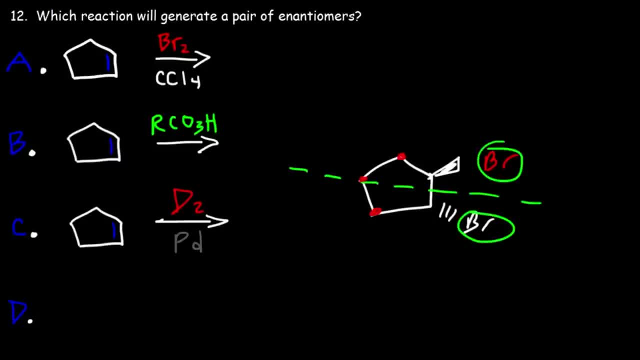 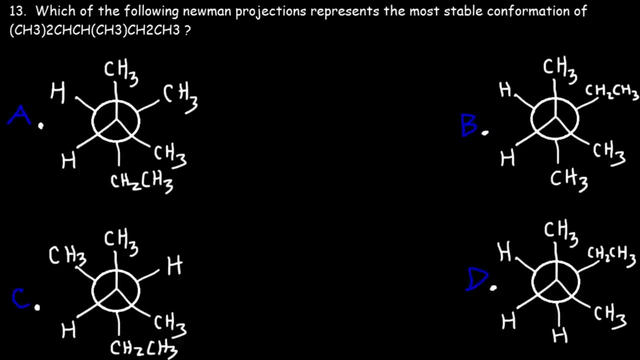 Because one is in the front And the other is in the back. They're not symmetrical, So that's why we don't have a line of symmetry. in this case, A would represent a pair of anandromous. Number 13: Which of the following Newman projections represents? 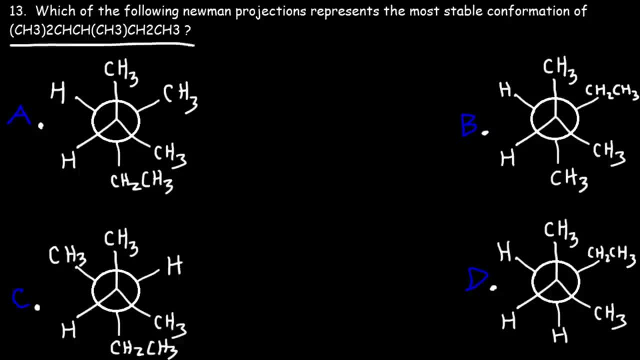 the most stable conformation of this molecule here. So Go ahead and try this problem. The first thing we should do Is we should draw a better structure. Let's expand the condensed structure. So let's start with the CH, So that carbon Has a hydrogen And it has two CH3 groups. 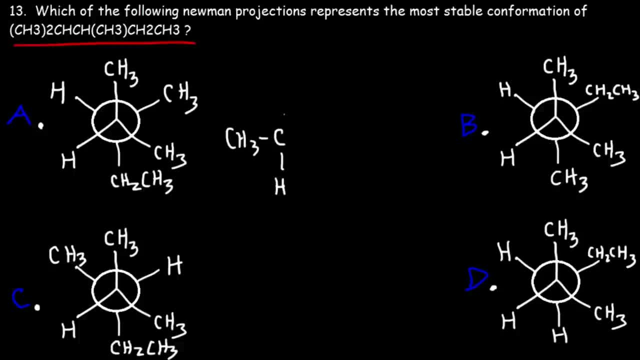 Attached to it. So it looks like this. Next, it's attached to another CH group. So basically, That's a carbon with a hydrogen And this CH Is attached to a CH3 And it's attached to A CH2CH3 group. So that's the structure That we have. 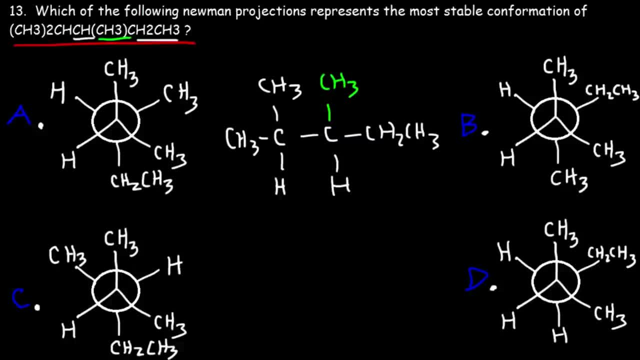 And looking at the answers, We can see that These two methyl groups Corresponds to These two methyl groups And this hydrogen Also corresponds to it. So therefore we're viewing it along The C2C3 bond, So the C2 carbon Is the one in the front. 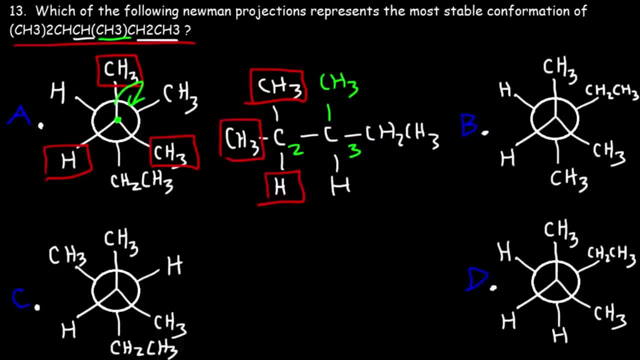 The C3 carbon Is behind it. We can't see it. Now attach the C3 carbon We have. I'm going to highlight it in yellow: We have a CH3 group, We have a hydrogen And we have An ethyl group. So now you know How to turn. 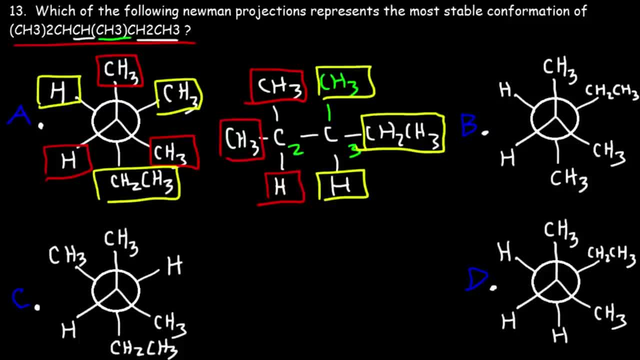 A condensed structure Into a muon projection. So, looking at A, B and C, A, B and C have the right Number of carbons, However, D does not. A, B and C all have Three methyl groups. Answer choice: D Only has two methyl groups, So therefore D doesn't have. 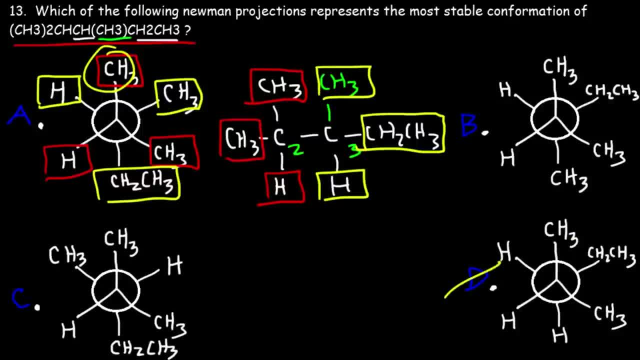 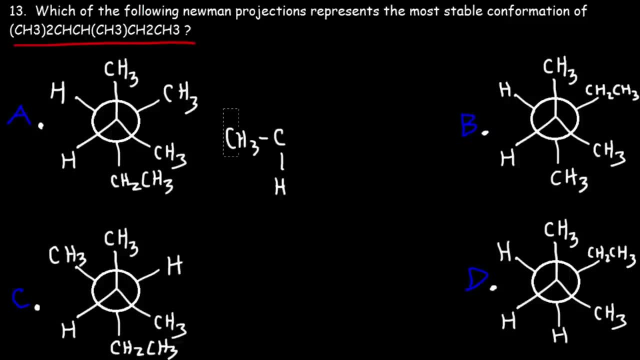 The right number of carbons, We can eliminate answer choice D. Now let's just get rid of a few things. So we need to identify the most stable Conformation Of the muon projection That represents this molecule Along the C2C3 bond. So how can we do this? 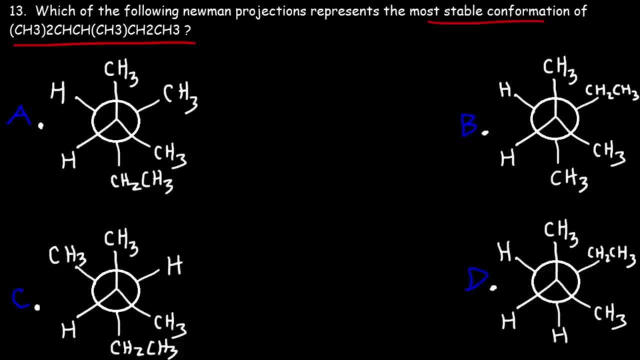 We need to count the number of C1C3 bonds Along the C2C3 bond. So how can we do this? We need to count the number Of C1C3 bonds Along the C2C3 bond, Along the C2C3 bond. 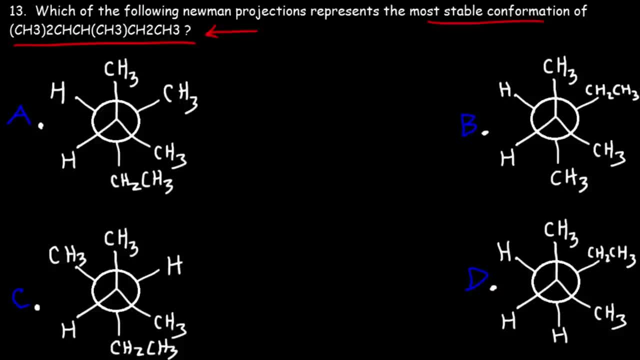 Along the C2C3 bond. Follow the number of GAUCH interactions. This is a GAUCH interaction. The CH3 groups are 60 degrees apart, So we will call this A methyl-methyl, A methyl-methyl-gAUCH interaction. This another methyl-methyl-gAUCH interaction. 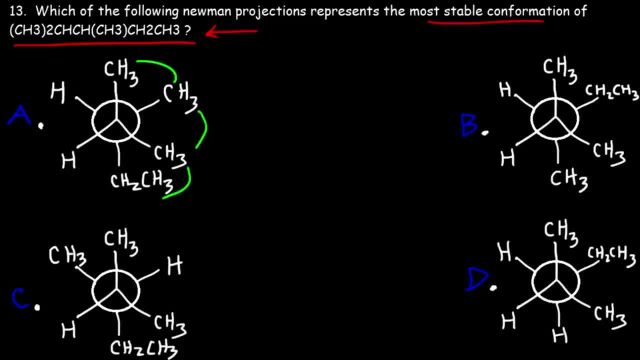 GAUCH interaction And that is a methyl ethyl GAUCH interaction. So A has three three GAUCH interactions, three GAUCH interactions And its no GAUCH interaction. B also has three gouge interactions. Here we have a methyl-ethyl gouge interaction, another methyl-ethyl and a methyl-methyl. 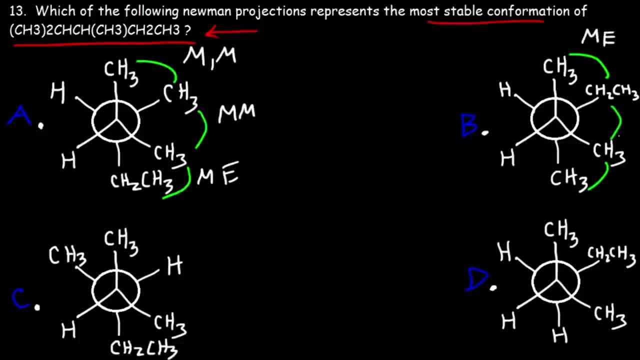 gouge interaction. Now, looking at answer choice C, there's only two gouge interactions: A methyl-methyl gouge interaction and a gouge interaction between a methyl and a ethyl group. So because answer choice C has the least number of gouge interactions and all of these are: 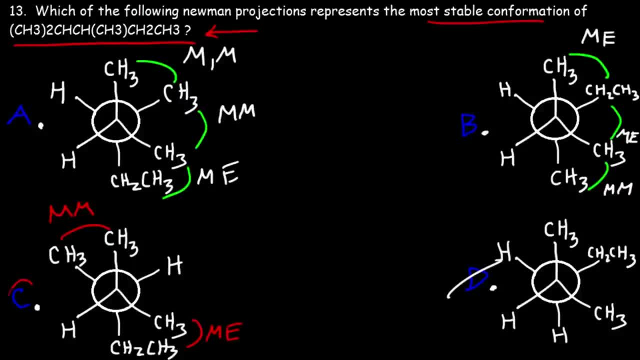 staggered conformations. answer choice C represents the most stable conformation Now between A and B. which one is more stable? So the methyl-methyl gouge interactions are the same. So we can cancel one One of them And the methyl-ethyl gouge interactions are the same. 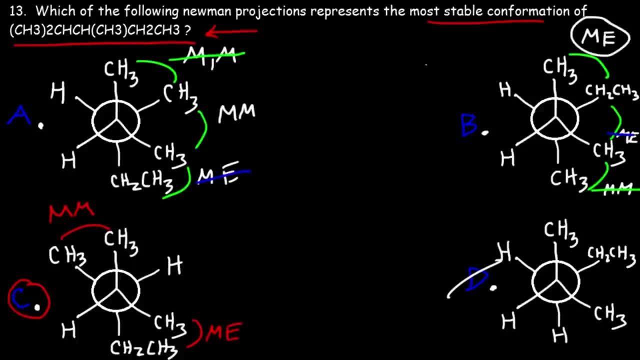 Now B has an additional methyl-ethyl gouge interaction. A has an additional methyl-methyl gouge interaction, So, which requires more energy To put a methyl group next to an ethyl group or two methyl groups next to each other. Now the ethyl group is bulkier or bigger than the methyl group, so there's going to be more. 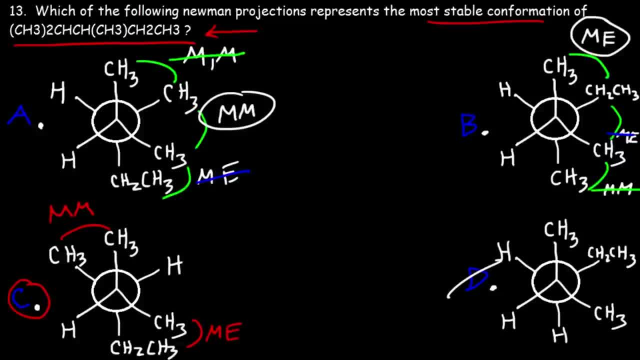 steric strain And a methyl interacts with an ethyl. So therefore, because there's more steric strain in answer choice B, it's going to be less stable than A. So if we had to rank it, C would be number one. 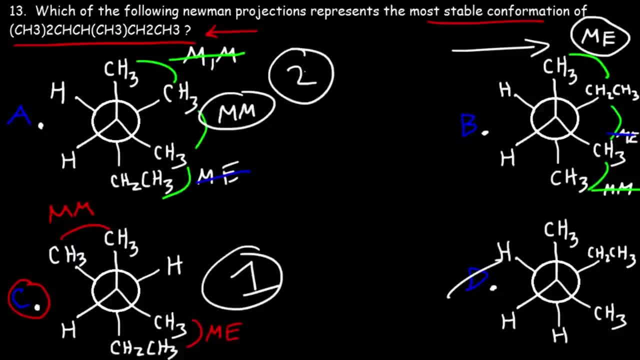 It's the most stable, Then A would be number two- It's the second most stable- And B would be number three. It's the least stable out of what's listed here due to the extra methyl-ethyl interaction And we can't compare D. 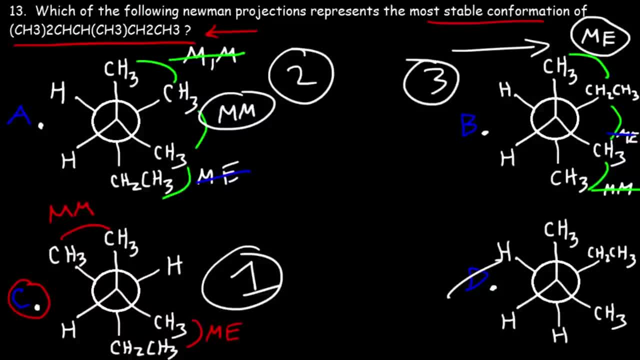 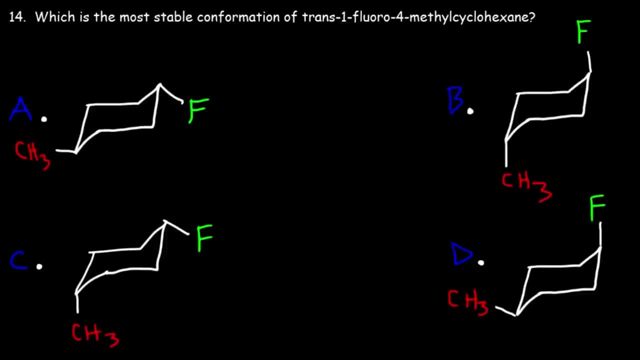 Because that represents A completely different compound. But C is the right answer for this problem, Number 14. Which is the most stable confirmation of trans-1-fluoro-4-methyl-cyclohexane. So first let's identify which of these represents trans and which ones are cis-isomers. 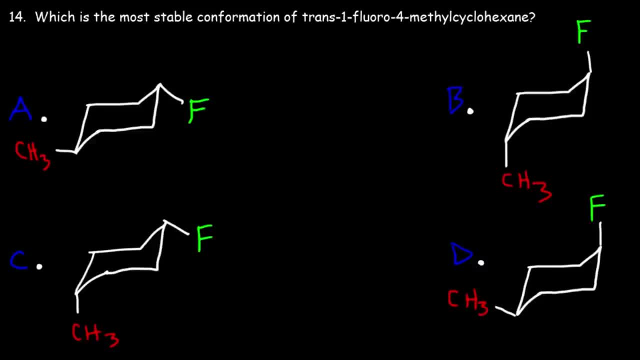 So A? is it a trans-isomer or a cis-isomer? The fluorine is in the equatorial position, which is 24.. So A is a trans-isomer or a cis-isomer? That's a trans-isomer, But notice that it's going down slightly. 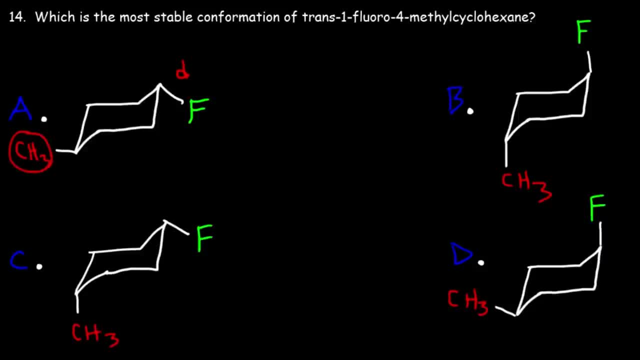 So it's equatorial down And the methyl group is in the equatorial position, but it's slanted slightly up. So if one position is up and the other is down, that is going to be the trans-isomer. Now, looking at answer choice B, the fluorine is in the axial up position. 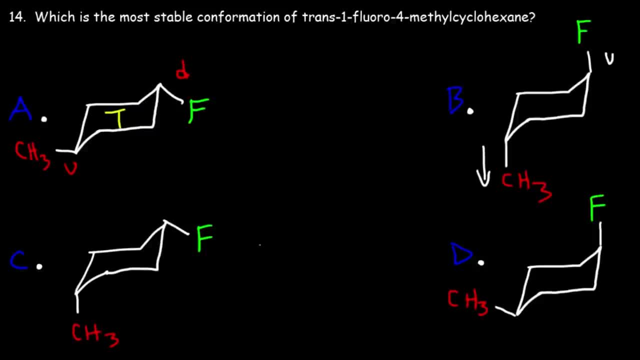 So I'm going to put U for up. The methyl group is in the axial down position, So that also represents a trans isomer. In answer choice C, the fluorine atom is in the equatorial down position and the methyl is in the axial down position. 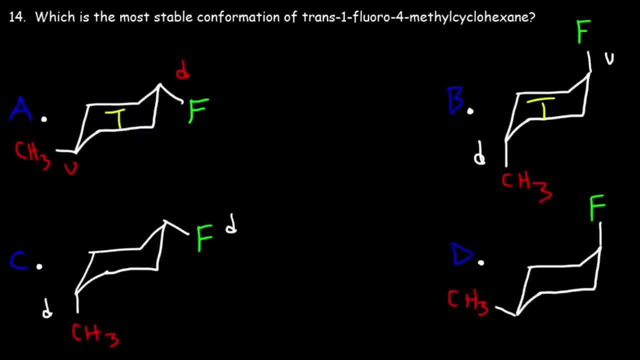 So because they're both in the same direction, that is, in the downward direction, this represents the cis isomer. Now for answer choice D: fluorine is in the up position and methyl is in the equatorial up position, So they're in the same direction. so this also represents a cis isomer. 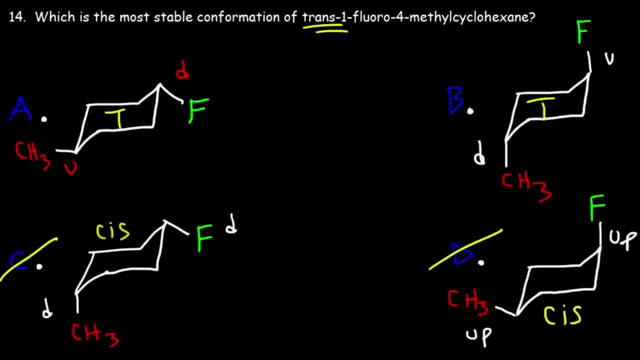 So we can eliminate answer choice C and D. We're looking for the trans isomer Now. in answer choice A, both groups are in the equatorial position. In answer choice B, they're both in the equatorial position. Which one is more stable, axial or equatorial? 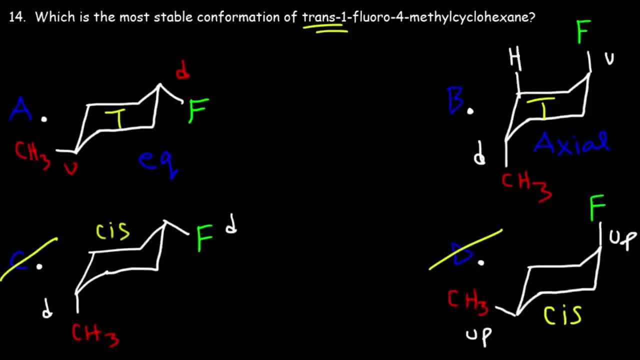 Well, there's something called 1,3-diaxial strain. So let's say, if we start from the fluorine On the third carbon, you have a hydrogen, And if you count in the other direction there's another one. 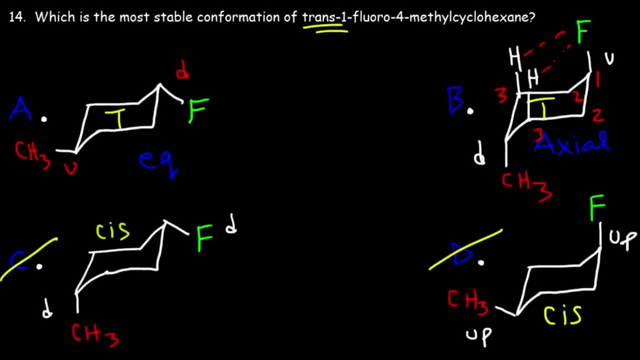 Fluorine interacts with these hydrogen atoms, making the axial position less stable. So therefore the most stable conformation is neutral, The one that has all the groups in the equatorial position. So answer choice A is the answer Number 15.. 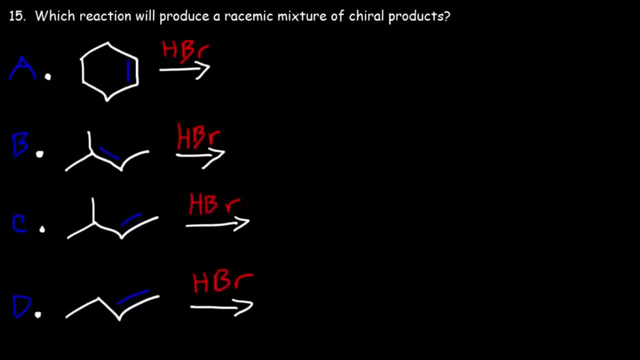 Which reaction will produce a racemic mixture of chiral products. So what do you think the answer is going to be? Well, let's go through each one. Once we add HBr to a double bond or to an alkene, the double bond is going to turn into a single bond. and we just got to add the bromine atom. 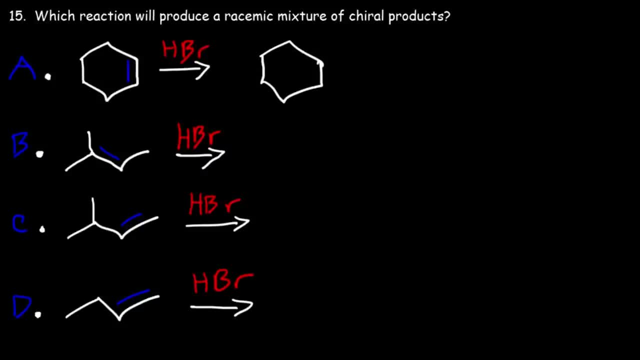 Now, this reaction typically occurs with macarmonic carve region, which is a combination of carbon atoms and a carbon atom. However, because the two carbon atoms across the double bond have the same substitution of both secondary carbons, this reaction is not regioselective. 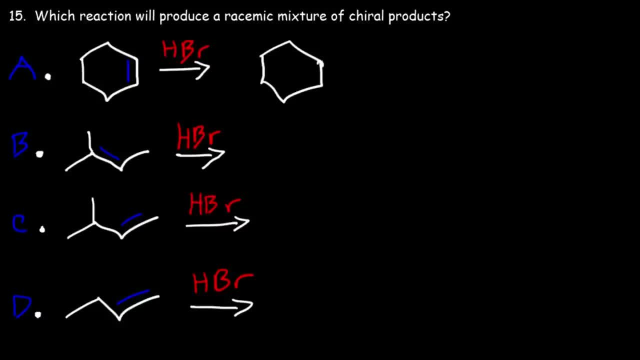 So you can put the bromine atom on any one of those two carbon atoms. So let's put it there. This particular product, is it chiral or achiral? The carbon that bears the bromine, does it have four different groups? 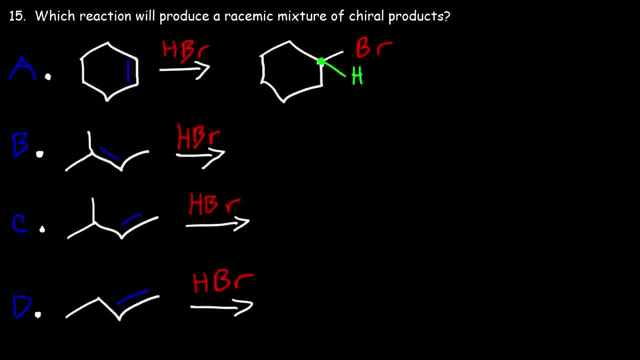 It has a bromine atom, It has a carbon atom, It has a hydrogen atom. But notice that the left side is equivalent to the right side. so it's not chiral. So that's an achiral product, which means we can eliminate answer choice A. 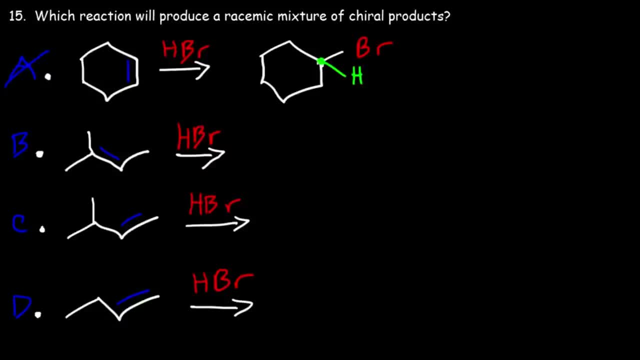 Now what about B? Will B generate an achiral product? Well, this carbon is secondary. This one is tertiary. The bromine is going to go on the tertiary carbon. The reason for that is because tertiary carbon is secondary. It's because tertiary carbocations are more stable and we can go over the mechanism. 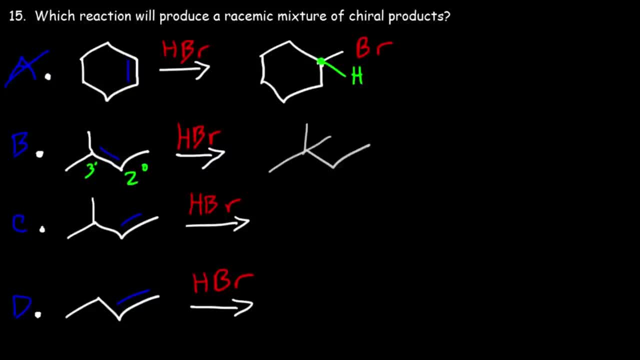 later, But for now, this is going to be the product, Now, this particular product. is it chiral or achiral? So, analyzing the carbon that has the bromine atom, that carbon has a bromine atom and ethyl group, But notice that it has two equivalent methyl groups. 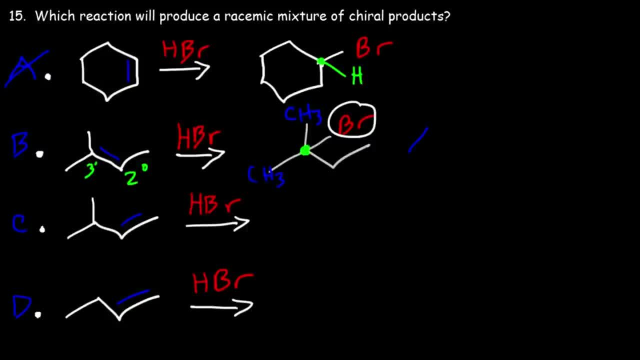 So it doesn't have four different groups, which means that it's achiral. So it's not chiral, So we can eliminate answer choice B. Now what about C? In this reaction there's going to be a carbocation rearrangement. 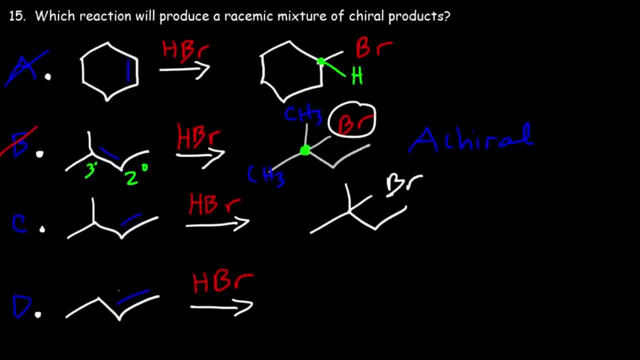 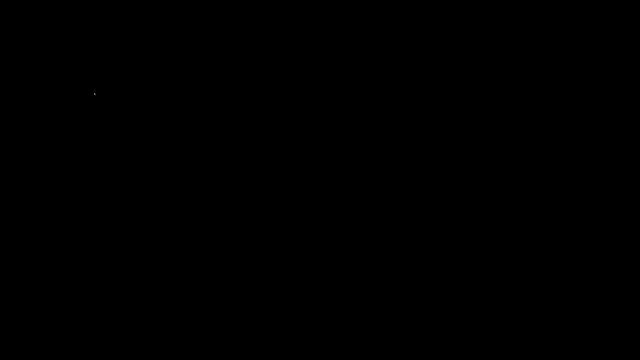 You're going to get the same product as answer choice B, So C is eliminated. The correct answer is D. But let's talk about why We have one butene and we're going to react it with hydrobromic acid. 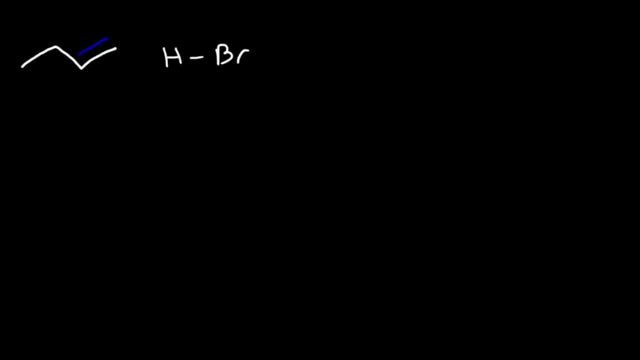 So in the mechanism, the first thing that's going to happen is the nucleophilic double bond is going to grab a hydrogen in HBr, expelling the bromine atom. Now, initially bromine has three lone pairs, But once the HBr bond breaks, bromine is going to pull the electrons toward itself. 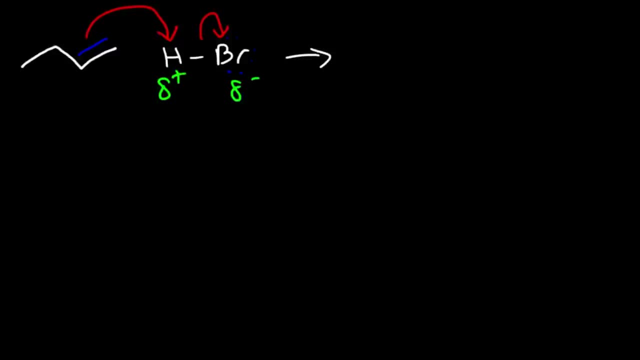 Bromine is more electronegative than hydrogen, And so when that bond breaks, that's why it pulls the electrons toward itself. Now, in this reaction, the nucleophilic double bond is going to grab a hydrogen in HBr, expelling the bromine atom. 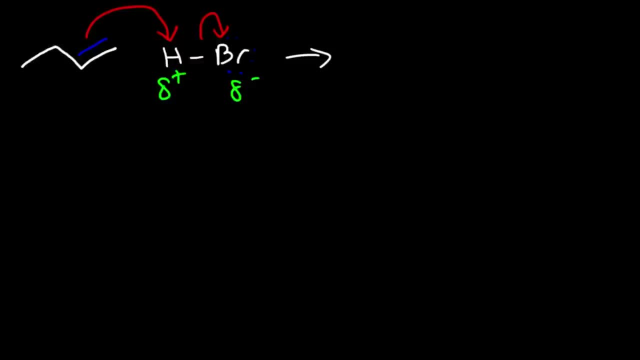 Now, initially, bromine has three lone pairs. So now where is the hydrogen going to go? Should we add the hydrogen to, let's say, the primary carbon or the secondary carbon? The hydrogen is going to go on the primary carbon. 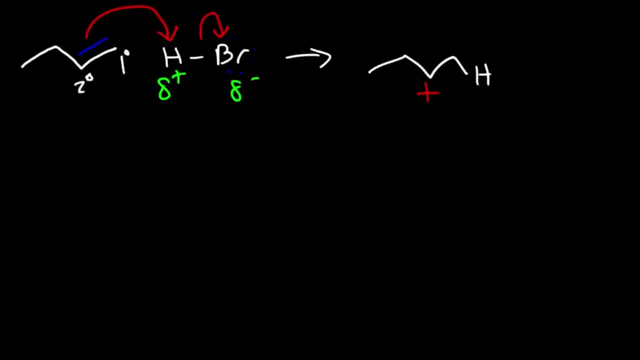 If we put it there, we're going to get a more stable secondary carbocation. If we put the hydrogen on the secondary carbon, we're going to get a less stable primary carbocation, which we don't want that. So now the bromide ion. 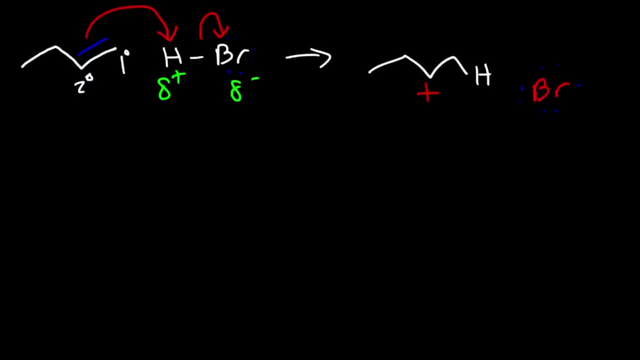 It has three low-pairs instead of three and it has a negative charge. It's attracted to the carbocation, So it can approach it from the front or the back, and that's why we can get a racemic mixture of products. 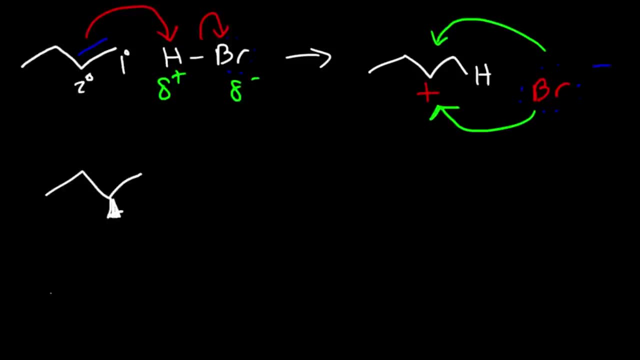 So if it approaches it from the front, we can get this product, or if it approaches it from the back, we can get this product. That's the problem, Alright. And both of these compounds are chiral. so if we analyze this carbon, it has a CH3 group. 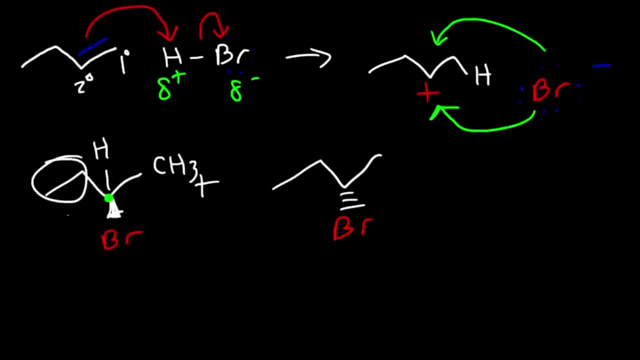 it has a bromine, it has a hydrogen and it has an ethyl group, So we have a racemic mixture of chiral products. Now, granted, this may not be a 50-50 equal racemic mixture- It could be 40-60,, 55-45, but we do have both enantiomers though. 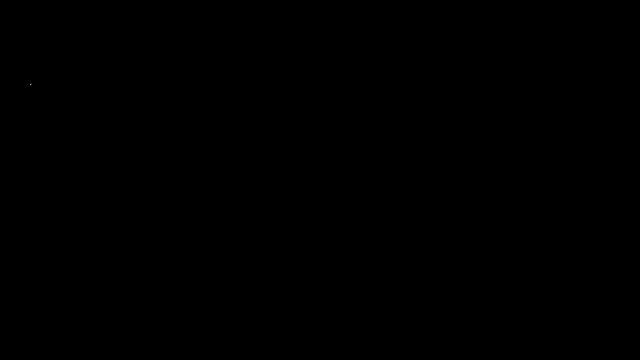 Now, what about the other reaction in part C? We mentioned that we're going to go over it. Let's talk about the mechanism. So, just like in the previous reaction, the double bond is going to react with HBr. It's going to acquire the hydrogen. And, just like before, it's going to react with HBr. So, just like in the previous reaction, the double bond is going to react with HBr. So, just like in the previous reaction, the double bond is going to react with HBr. 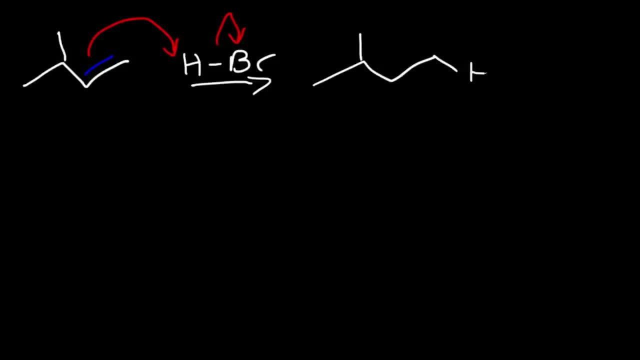 So, just like in the previous reaction, the double bond is going to react with HBr. We're going to put the hydrogen on the less substituted carbon, that is, the primary carbon, so we can get a more stable secondary carbocation. Now the secondary carbocation is adjacent to a tertiary carbon. 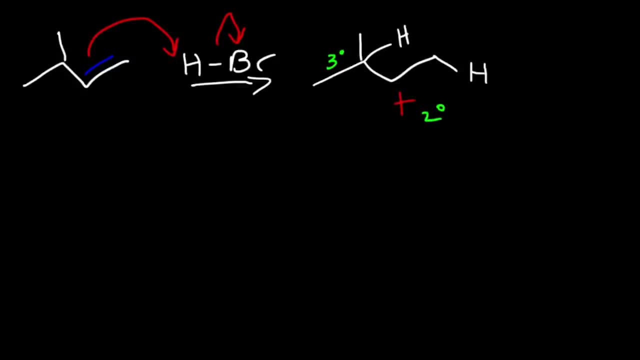 Whenever you see that there's going to be a hydride shift, And so this hydrogen is going to glide towards that carbocation, And so the hydrogen and the carbocation they're going to trade places. That's where this, this stoichiometry product, is going to be located. 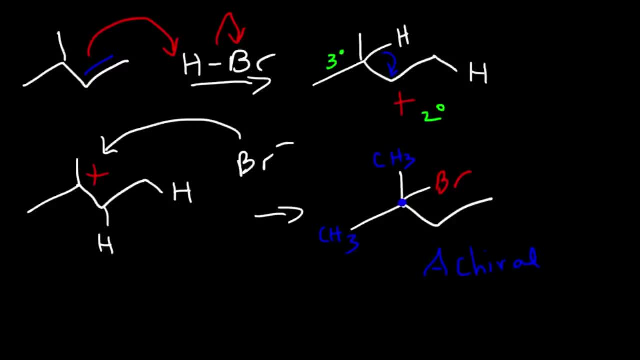 Here. for safety's sake, don't call this congratulate me or go play with your family and your dad. We don't need to play a party Because we don't play it, But if you break the trampoline, then you break beyond that because of contact. 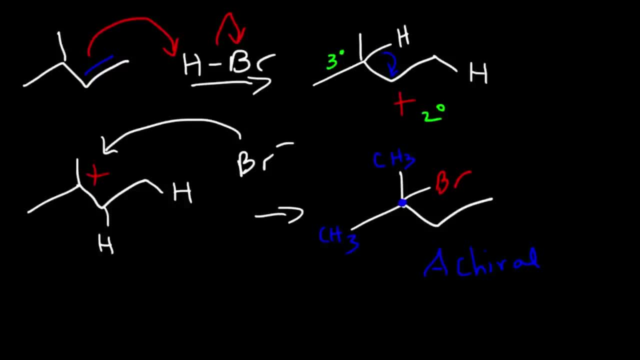 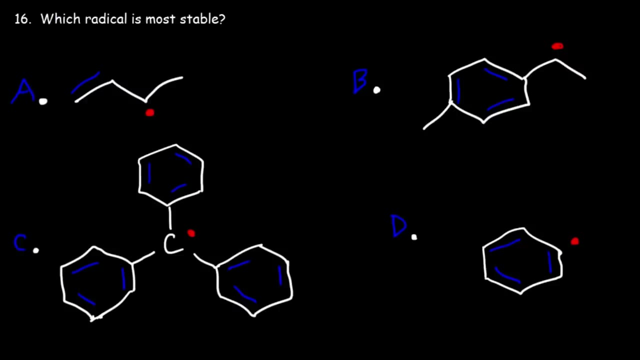 A and B. There's no carbocation rearrangement for those. so the first step is going to be the same. You just add HBr and then the bromide attacks the carbocation and you'll get the product. So that's it for this problem 16.. Which radical is most stable? Is it going? 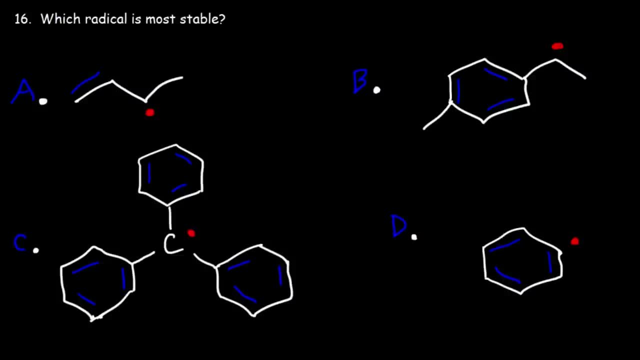 to be A, B, C or D. Well, let's identify each radical. So let's start with A. This carbon is secondary because it's attached to other carbons and it's adjacent to a double bond, So this is a secondary allylic radical. Now looking at answer choice B: this carbon. 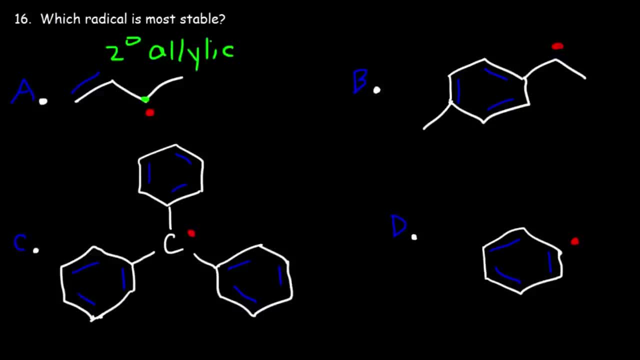 is also secondary and it's next to it's one carbon away from a benzene ring. So this is a secondary benzylic radical. Here we have an arrow radical. The unpaired electron is directly attached to a double bond. And for answer choice C we have a tertiary benzylic. 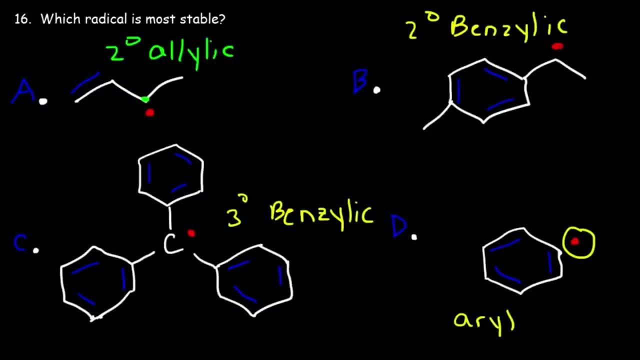 radical, And the reason why it's tertiary is because the carbon that bears the radical is attached to three other carbons and it's one carbon away from the benzene ring. So which of these is most stable? Well, it turns out that the tertiary benzylic radical is. 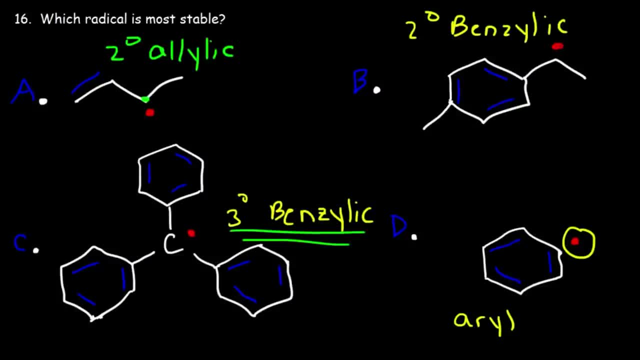 the most stable. The tertiary radicals are more stable than secondary radicals. By the way, this is a secondary arrow radical. The radical is attached to two other carbon atoms, So we have the most substituted radical in answer, choice C. but also notice that it's attached to three. 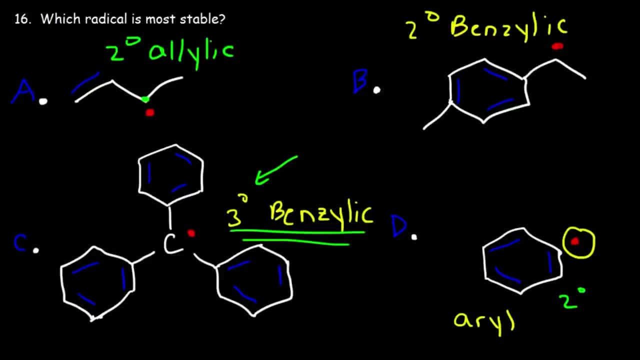 benzene rings. So there's a total of 10 resonance structures that you can draw. There's nine additional structures, including- well, if you add this one, then it's a total of 10, but not including this one. There's nine other resonance structures that you can draw. This compound only has a total. 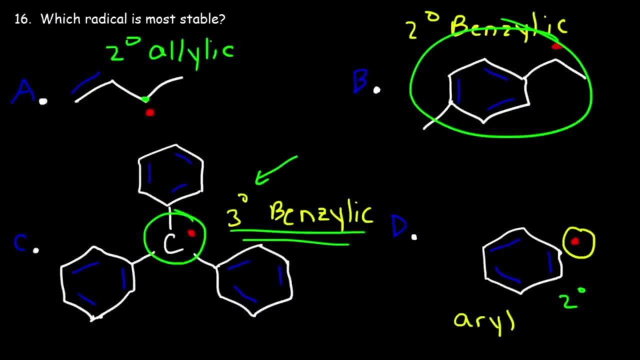 of four resonance structures. A only has a total of two resonance structures. D doesn't have any. D is the least stable. It's not good to put a radical directly attached to a double bond or directly on the benzene ring. So if we had to rank it, C is number one. It's the most stable, The second most stable. 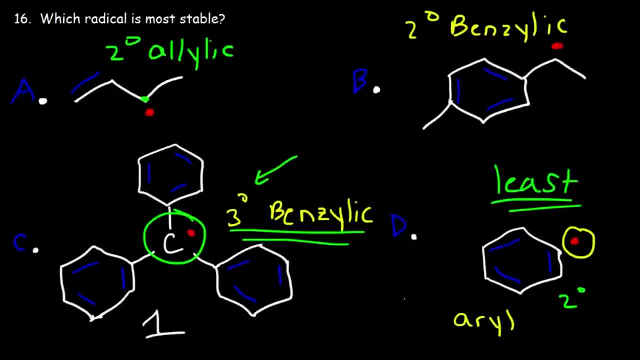 would you think? I think it's A or B. The second most stable is going to be B, The secondary benzylic radical. as we mentioned before, it can form four resonance structures, including the one that you see here, Whereas in A it can only draw. we can only get two resonance structures. So therefore, 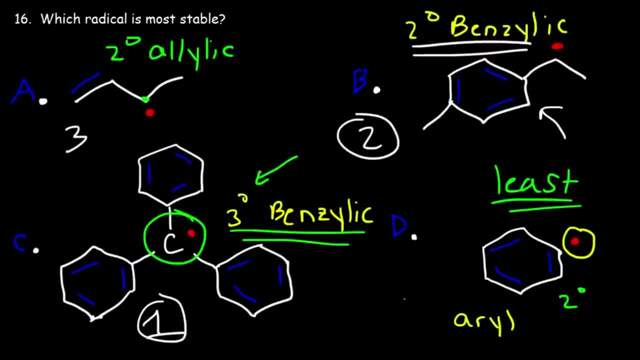 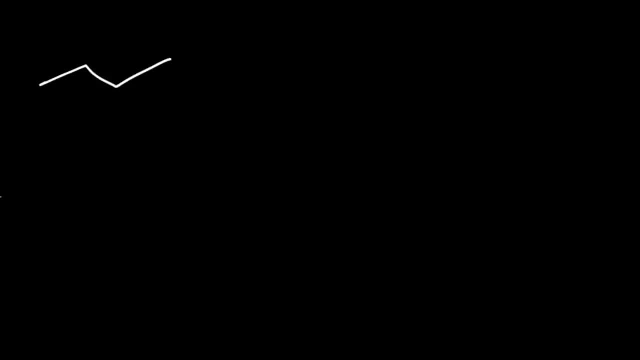 B is going to be the second most stable, A is the third most stable and D is the least. Now let's talk about the resonance structures that we can draw. Let's start with the secondary radicals. The first one is the secondary allylic radical. 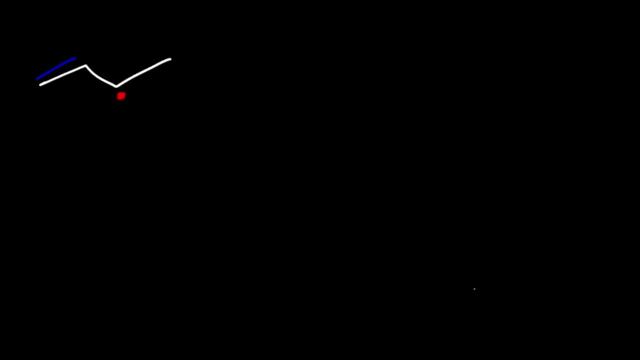 Now, when dealing with radical compounds, you need to use half arrows. Half arrows represent the flow of one electron and a full arrow represents the flow of two electrons. So the double bond basically has two electrons on it, So we can represent it like this One. 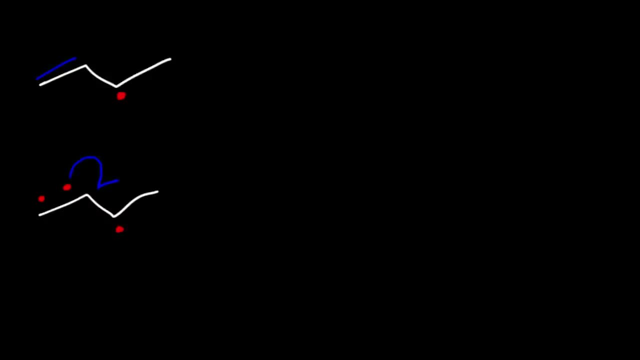 of the electrons will move to form a double bond And the other unpaired electron will move in this direction. The other one will stay where it is. So we're going to get this particular resonance form And there's going to be a radical 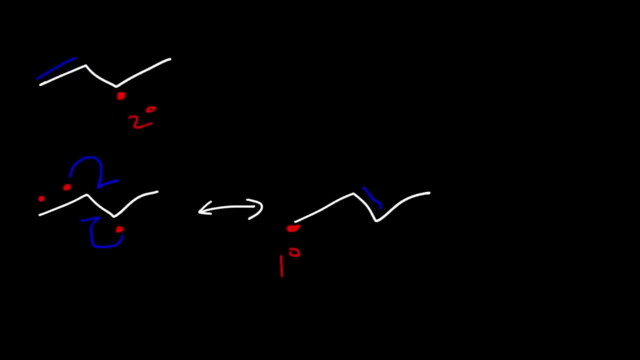 left on the primary carbon. Which of these two resonance contributors is more stable? Which one contributes more to the resonance hybrid? The one that's more stable is the secondary radical. Secondary radicals are more stable than primary radicals. So if you ever get a question to ask you which one is the major resonance contributor, it's simply the resonance. 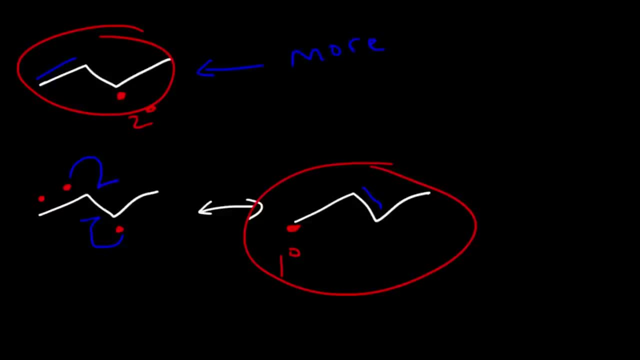 form that's more stable. Now, let's say, if you're going to draw the resonance structure from this form instead of using two dots here, Here's what you need to do. This is going to be three arrows that you need to show instead of two. So the first arrow and the second. 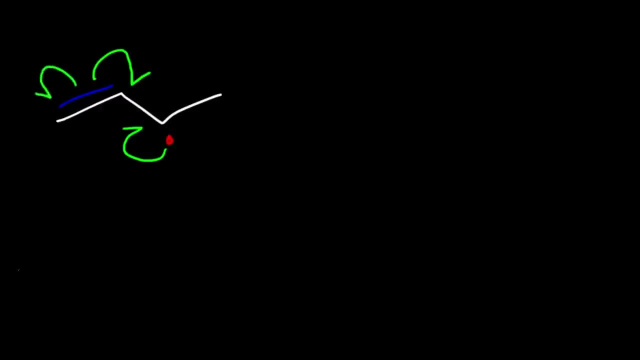 arrow is going to be the same. However, you need to show this third arrow where the radical is going to be placed on the primary carbon, And this would lead us to get this product. Now, going back to this compound, let's show all four resonance structures. So this is. 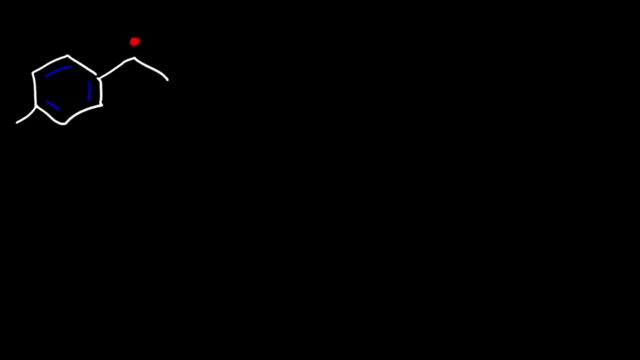 the primary carbon, You first break off two, so this is the burner itself. Follow my instructions here. The red of the two yellow bones is the second respond. Even though the first smoke up was, of course, a neutral bond, we got some red. So once we break off the second bond, 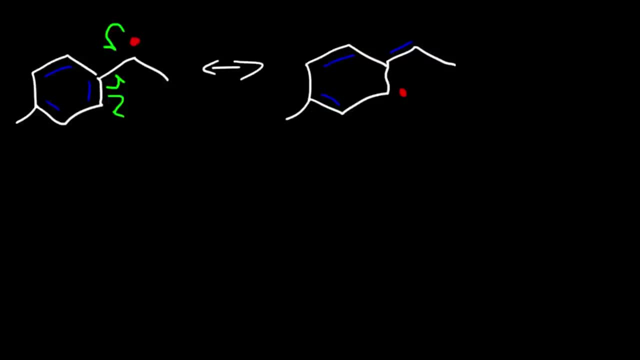 how red is the second bond? It's said this red is a realise phi-magnon. So right now, this to the next position. So one electron will move over here and this radical or that unpaired electron will combine with it to form a double bond. 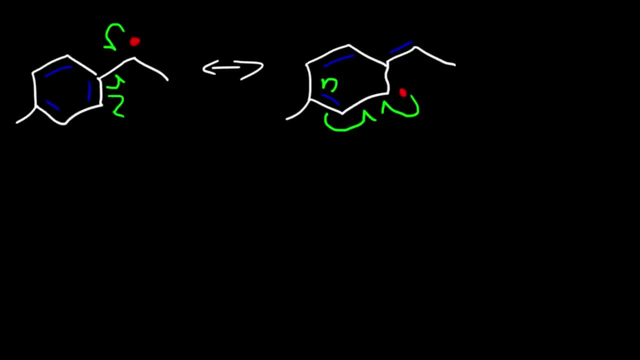 and the other unpaired electron will form a radical two carbons away. So now we have a double bond here, and this is a tertiary radical. Now for the last one. we can follow the same process, So this is the fourth resonance structure that we can draw. 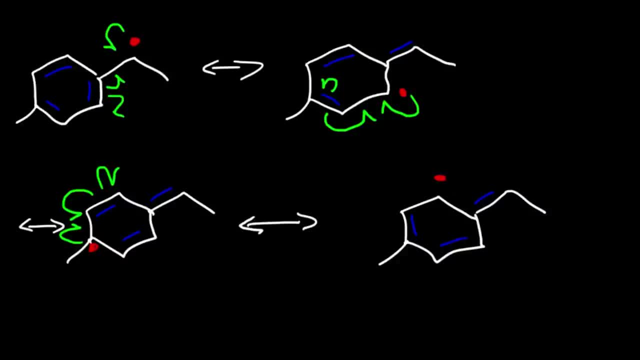 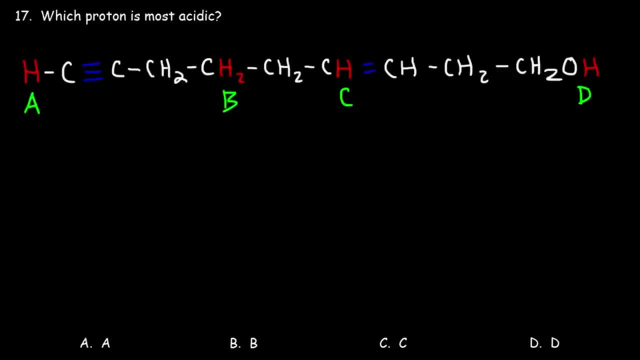 And so that's it. So now you know how to draw the different resonance forms when dealing with radicals. So now you know how to draw the different resonance forms when dealing with radicals and double bonds. Number 17. Which proton is most acidic? 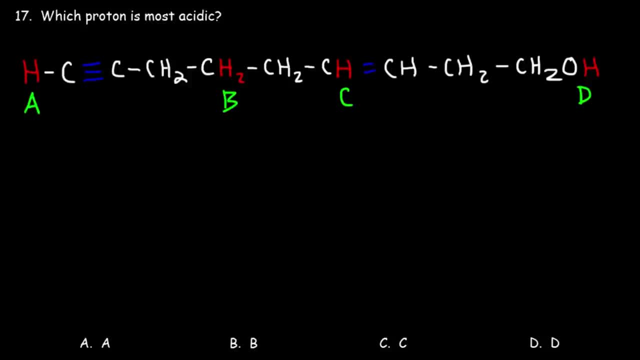 Well, let's find the pKa values, And whichever hydrogen has the lowest pKa value, that's going to be the one that's most acidic. So what is the pKa of a hydrogen that's attached to, let's say, an alkyne? 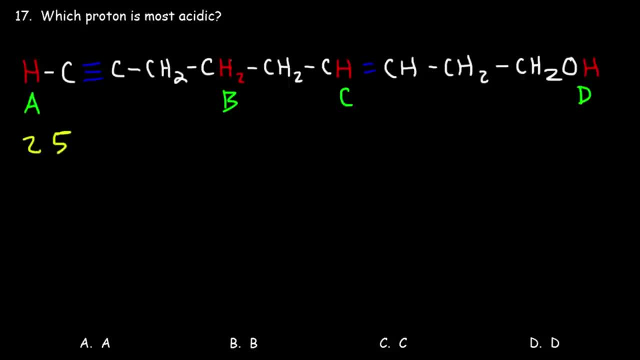 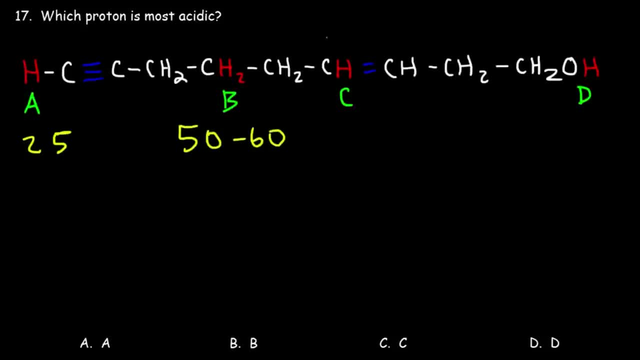 The pKa is 25.. The pKa is 25.. The pKa is very high. It's about 50 to 60.. A hydrogen that's attached to an alkane: the pKa is around 44,, if I remember correctly. It's somewhere in the 40s And for an alcohol the pKa is about 16 to 18.. So clearly we can see that the OH group is going to be the most acidic. It has the lowest pKa value. So D is the answer. So, if we had to rank it, this is the most acidic. The second most acidic is the hydrogen, the hydrogen that's attached to the alkane. This is the third most acidic And this is the least. 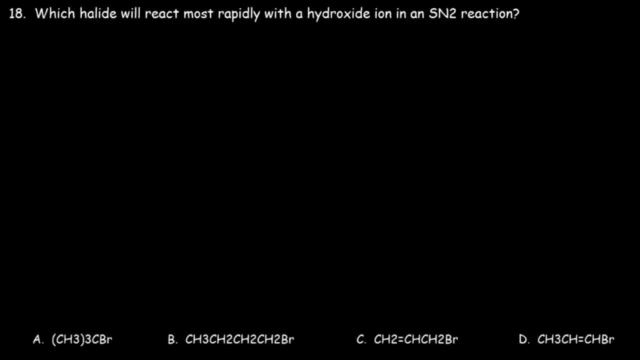 And so that's it for this problem, Number 18.. Which halide will react most rapidly with a hydroxide ion in an SN2 reaction? Is it A, B, C or D? Well, the first thing that we should do, 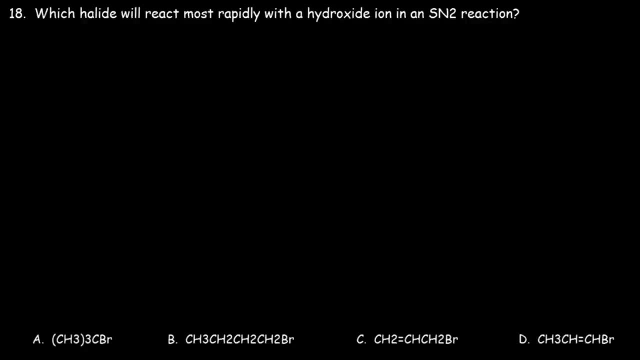 is, we need to convert the condensed structure into a line structure. So let's start with A. We have a carbon that's attached to three methyl groups and we have a bromine atom on it, So basically, this is a tertiary alkyl halides. 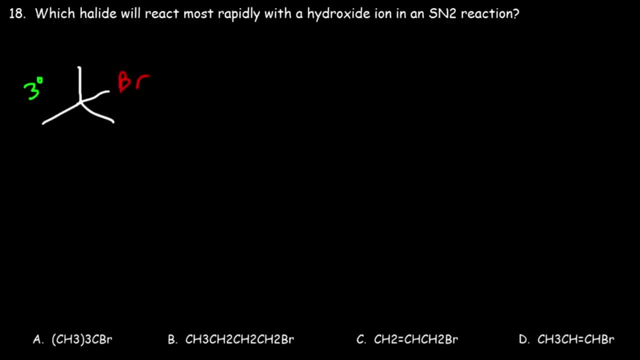 It turns out that tertiary alkyl halides do not work very well in an SN2 reaction, And the reason for that is due to steric hindrance. The hydroxide, which is the nucleophile, is going to have a difficult time. 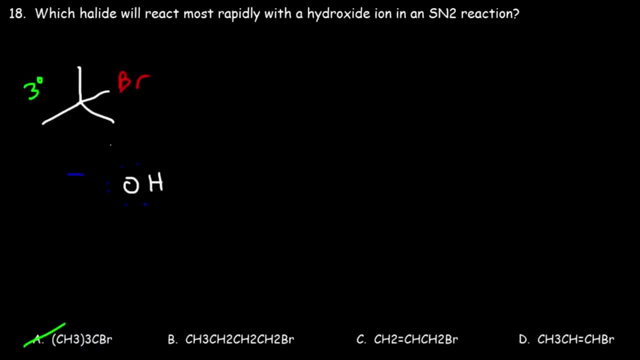 approaching the carbon that it needs to attack. And the reason for that is because these bulky methyl groups they block approach to the carbon that it has to attack. So those methyl groups block that carbon. They protect them from nucleophilic attack. And so that's why tertiary alkyl halides 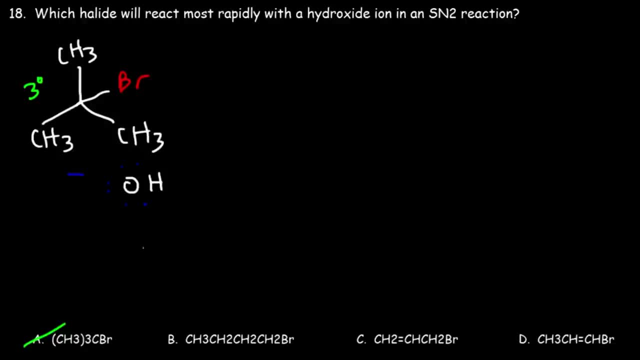 do not work very well for SN2 reactions. So A is eliminated. Now looking at answer choice B, this is one bromobutane, So we have four carbons and a bromine atom. That's a primary alkyl halide. 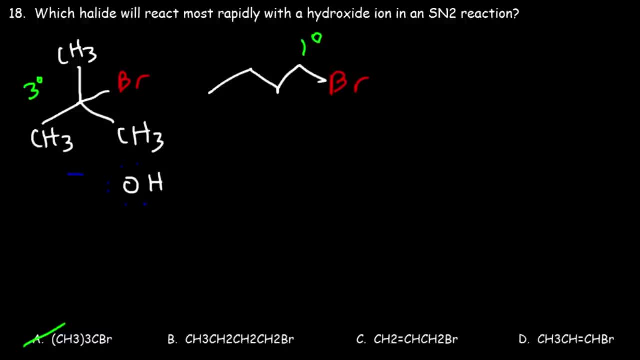 Primary alkyl halides work pretty well for SN2 reactions. Methyl halides work better than primary halides because the methyl carbon is very accessible to the nucleophile. Primary halides work better than secondary ones And secondary halides are more accessible than tertiary ones. 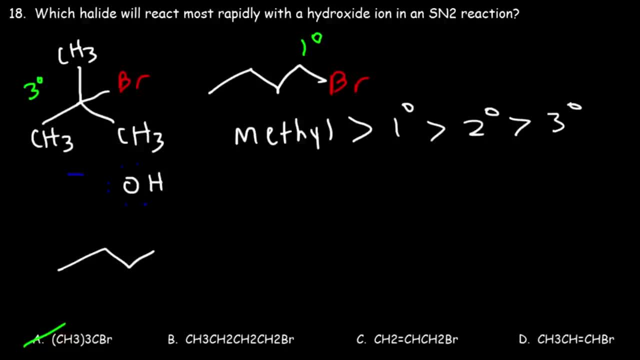 Answer choice C has three carbons and a bromine atom, But answer choice C represents a primary allylic halide And answer choice D represents a primary allylic halide. and answer choice D represents a primary allylic halide. C represents a vanillic halide. 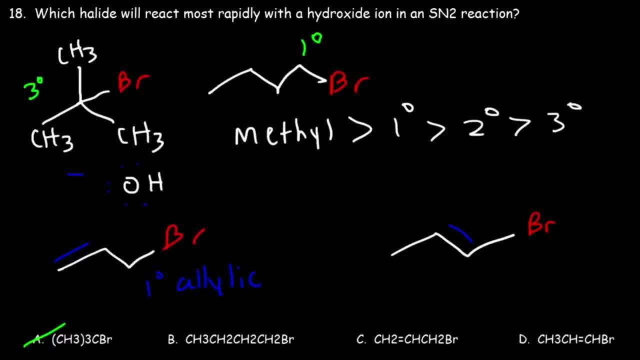 The bromine is attached to a carbon that is part of the double bond system. Now, something else that you need to know is that vanillic halides do not work at all for SN2 reactions and for SN1 reactions, So therefore we could eliminate answer choice D. 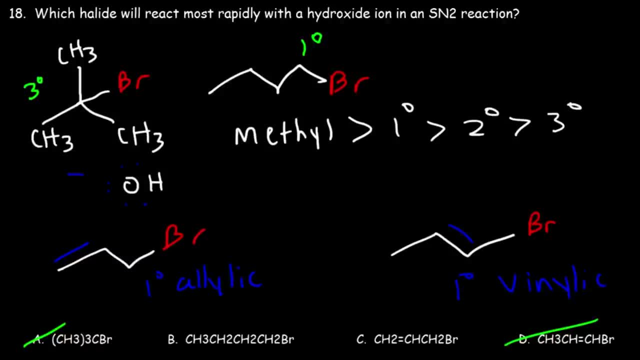 So we're between B and C. So which is better- A primary alkyl halide or a primary allylic halide? It turns out that allylic halides are more reactive toward SN1 and SN2 reactions than their alkyl halide counterparts. 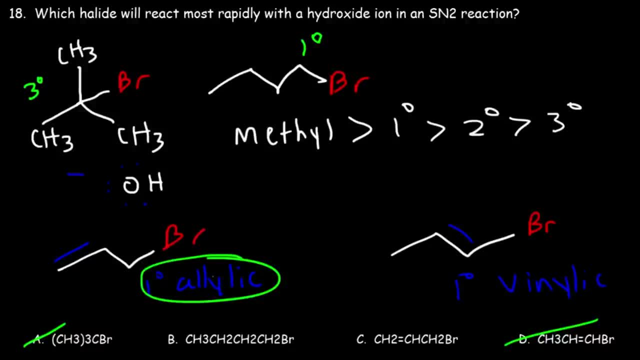 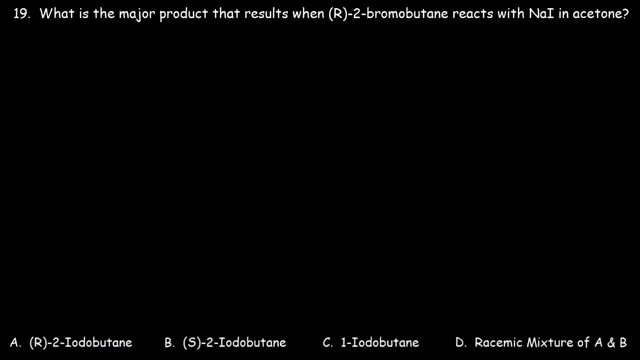 So a primary allylic halide works better than a primary alkyl halide. Okay, So C is a better substrate than B. It's going to react more rapidly in the SN2 reaction, So this is the answer 19.. What is the major product that results when R2 bromobutane reacts with sodium iodide and 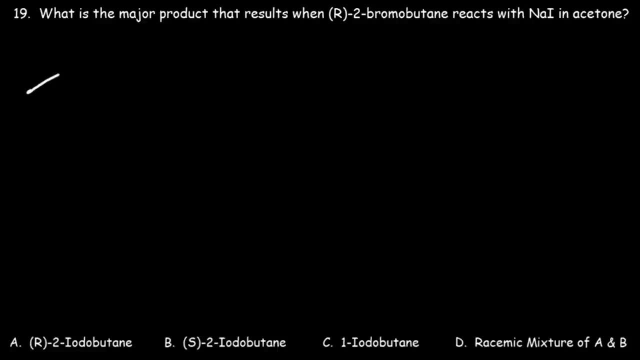 acetone. So first let's draw R2 bromobutane. We need to put the bromine atom in the front And we need to put the hydrogen in the back. So let's make sure it's R. The bromine atom has the highest priority. 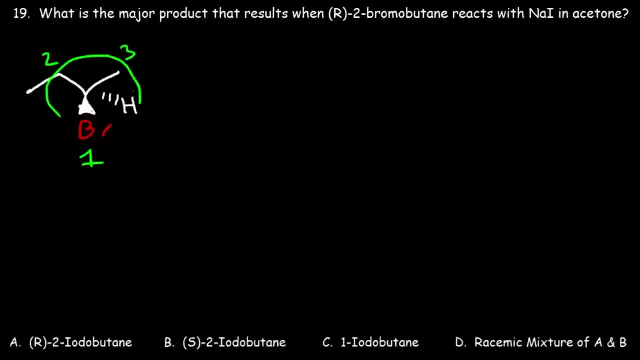 Next is the ethyl group, then the methyl group. So if we count it from 1,, 2, to 3, H is in the back, which is group number 4, we can see that we have the R isomer. 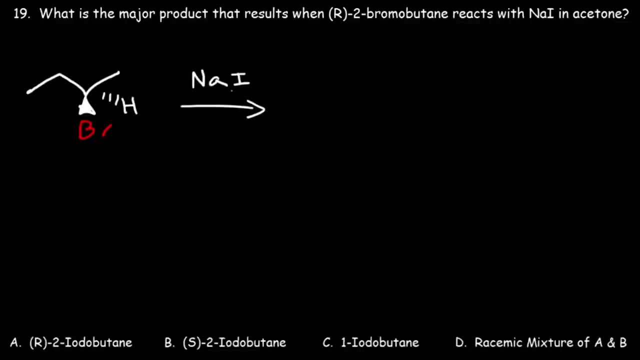 Now, we're going to react this with sodium iodide and acetone. So what kind of reaction is this? We're going to react this with sodium iodide and acetone. So what kind of reaction is this? We're going to react this with sodium iodide and acetone. 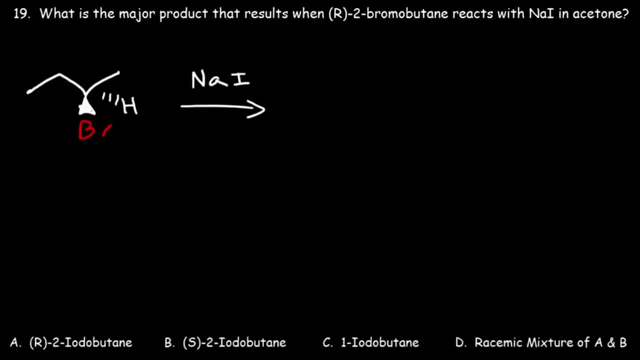 So what kind of reaction will we have? Is this an SN2 reaction? Is it an SN1?? Typically, when you have an alkyl halide reacting with some sort of nucleophile, you have to think about nucleophilic reactions and elimination reactions. 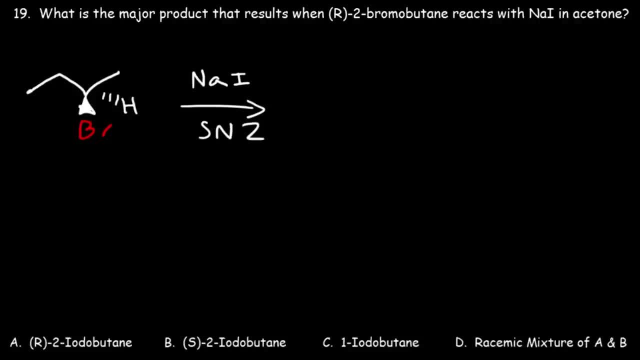 This particular reaction is an SN2 reaction. We have the secondary alkyl halide and sodium iodide, The iodide part 19.. It's a good nucleophile. Acetone is a polar aprotic solvent. Aprotic solvents do not have any OH or NH groups and they work well for SN2 reactions. 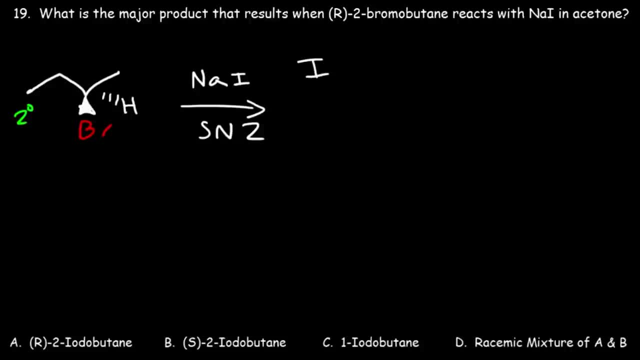 What kind of product will we get? In the SN2 reaction, the iodide is going to attack the substrate. It's going to act as a nucleophile. It's going to attack the carbon from the back, back, expelling the bromine atom Because it approaches it from the backside. we're 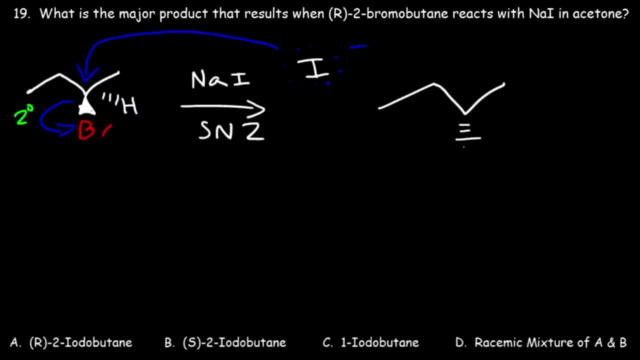 going to have inversion of configuration, So the iodide is going to be in the back and now H is in the front. So before we had the R isomer, now we have the S isomer. So the product is 2-iodobutane but the S isomer. so B is the answer, The only way. 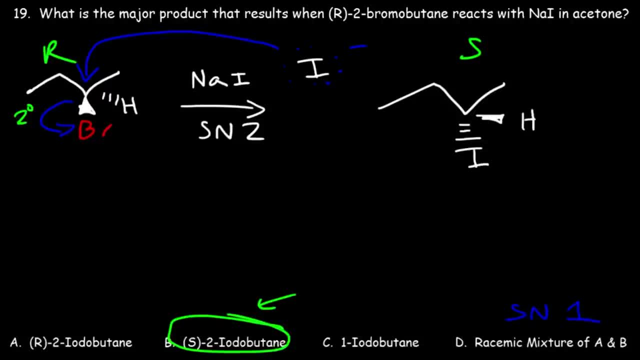 we can get a mixture is: if it was an SN1 reaction, Then D would be correct. but this is an SN2 reaction which doesn't yield a racemic mixture. It only gives you the inverted product. So SN2 reactions always occur with inversion of configuration. So B is the answer. 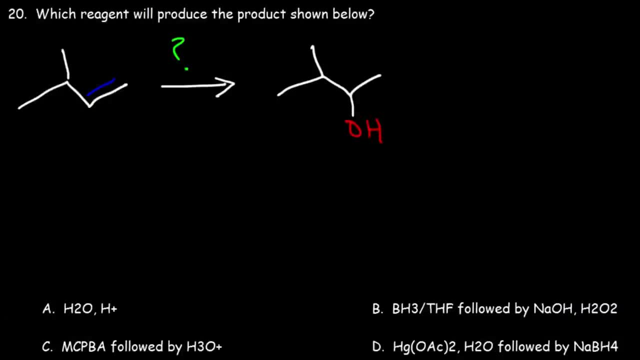 Number 20.. Which reagent will produce the product shown below? So how can we convert three metals into one? Well, let's start with answer choice. A Water with H plus is equivalent to H3O plus. This reaction will give us an alcohol, but rearrangements will occur. It turns out that 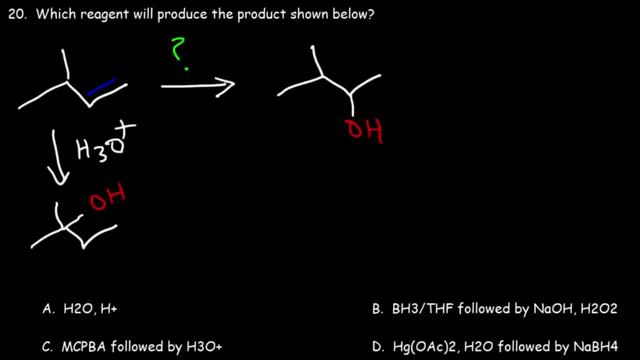 the OH group will be on the tertiary carbon, which is not what we want. So answer choice A is not the right answer. Now let's focus on answer choice B. We know that the Videodlaughing agent forms is on the tertiary carbon. however, 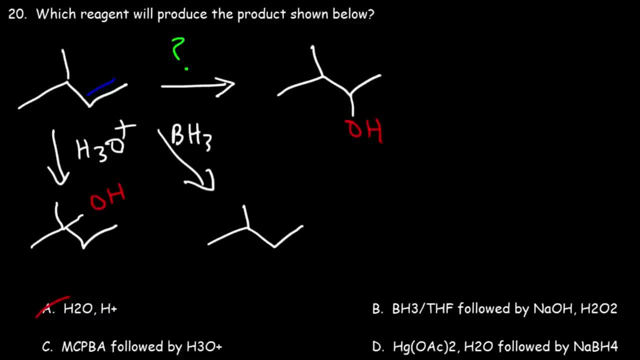 the oh group or OH group can form on its own and will be eggs of sucrose and gum. This is the way we'll be doing the test For question B. we will choose nothing but the OH group. Question C: Why wouldn't we choose the OH group? 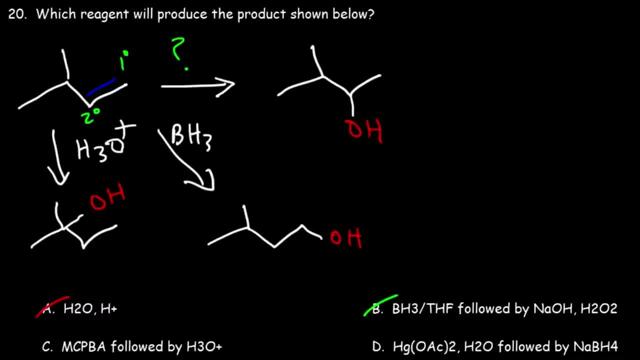 Because each of the two nuclear compounds b is not going to replace the other. 1. won't give us the answer that we want. Now answer choice C: We have MCPBA, metachloroperoxybenzoic acid. Once we add that, we're going to get an epoxide which will look 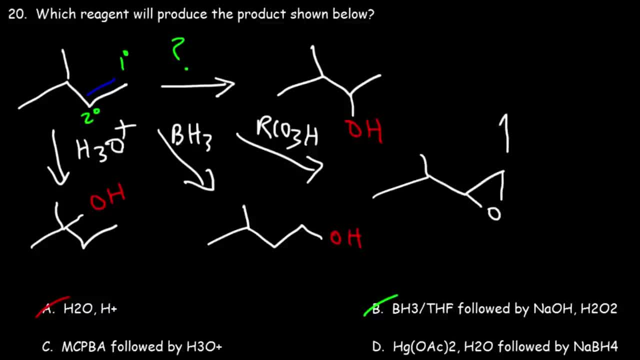 like this: And then, once we add H3O+, the ring will open, giving us two alcohols, which we don't want. two alcohols, We want one. We don't want a diol. So C is eliminated, The only one that will. 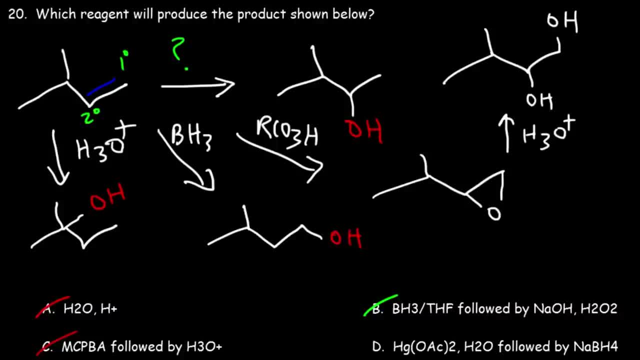 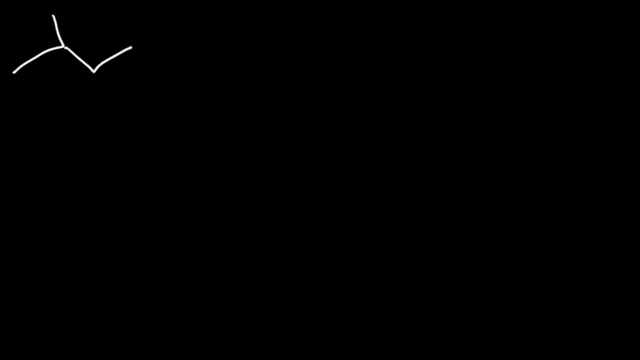 give us the Morkovnikov product without rearrangement, is mercury acetate with water, followed by sodium borohydride. So D is the right answer. Now let's go over a few things, particularly the mechanism of some of these reactions. So let's react this alkene with H3O+. 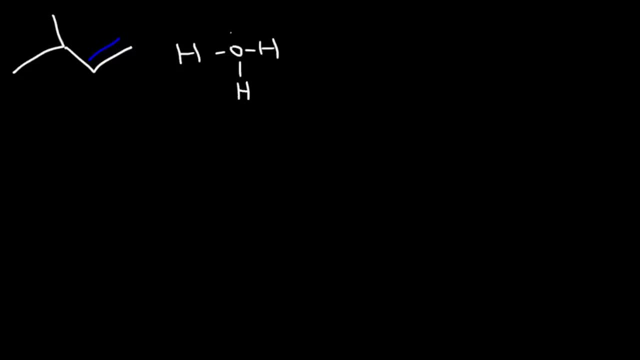 So the first thing that's going to happen, the double bond is going to grab a hydrogen expel in water. Now we're going to add the hydrogen on the less substituted carbon of the double bond, that is, on a primary carbon. If we do that, we're going to get a secondary. 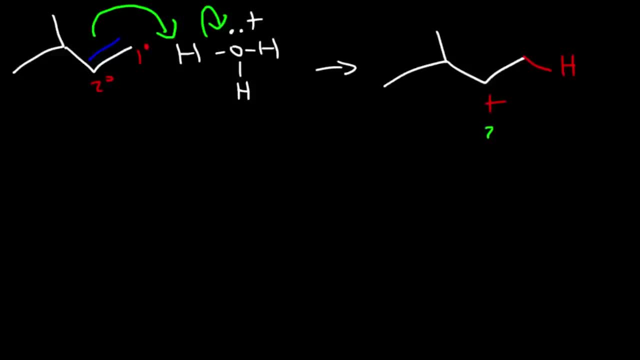 carbocation. Now the secondary carbocation is adjacent to a tertiary carbon, which means that hydride shift occur, and so now what we have is a tertiary carbocation. at this point water is going to react with it. so now oxygen now has the positive charge anytime. oxygen has three bonds. 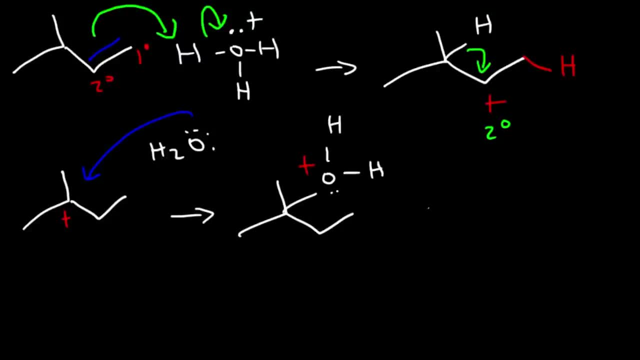 it's going to have a plus charge. now what we need to do is use another water molecule to get rid of one of these hydrogen atoms. so the final answer is this particular alcohol: 2-methyl 2-bionol. so, as we can see, a is not the 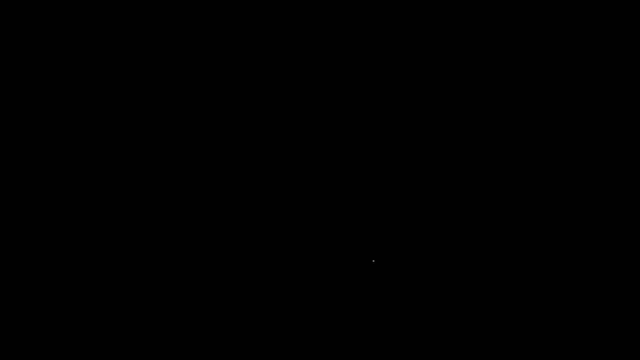 right answer is not the product that we want, so now let's move on to be so. once we add boron, i'm going to write it like this: once we had bh3, it's going to react with the alkene form in this product, the hydrogen is going to go on the more substitute carbon, since hydrogen is more. 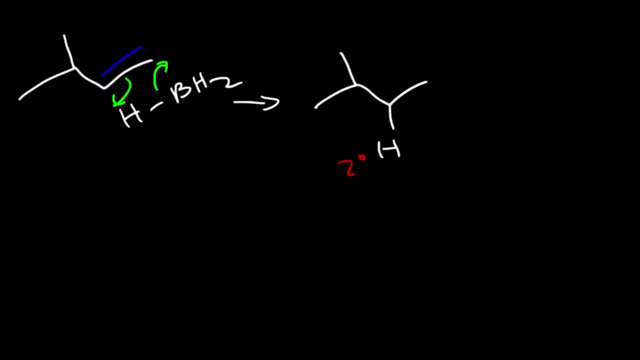 electronegative than boron, and the bh2 group will go on the less substituted carbon. now, once we add sodium hydroxide with hydrogen peroxide, the net result is that the bh2 group will be replaced with an OH group, and so this is the product for that reaction. now let's talk about 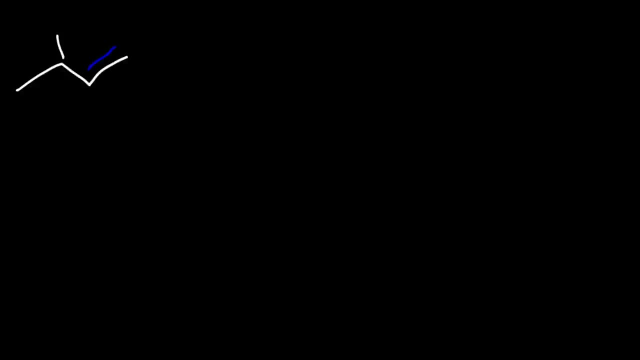 the reaction in part C or answer choice C. so first we're going to react it with a proxy acid, RCO3H or mcpb8. this will give us an epoxide. now, once we add HgO plus to it, which I'm going to- 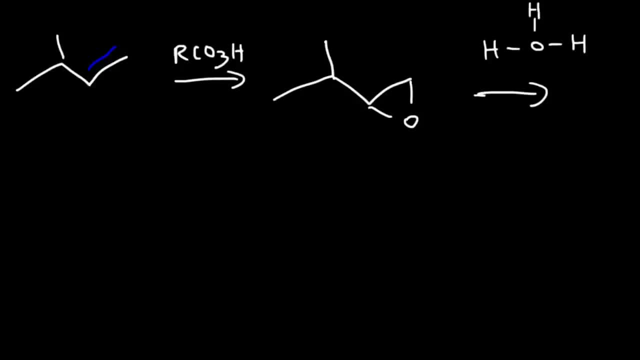 write it out. the oxygen is going to receive a hydrogen from HgO plus, so it's going to be activated, and once HgO plus loses the hydrogen, it converts into water. now water is going to attack the secondary carbon as opposed to the primary carbon. 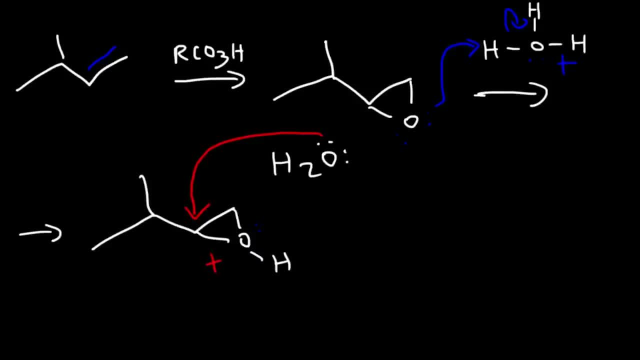 it turns out that the secondary carbon has more partial charge than the primary carbon, and so that's why water is attracted to it. if you draw the resin structure of this molecule, which bond should we break this one or this one? if we break this bond, this will. 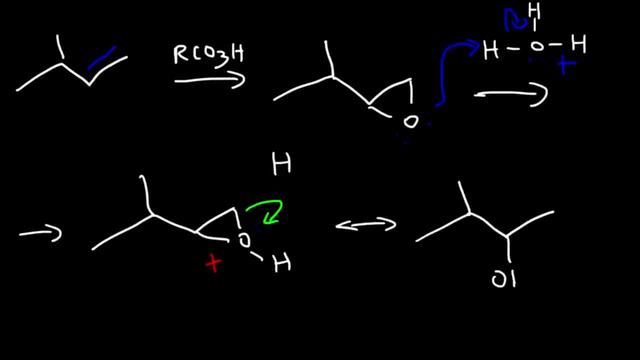 give us a primary carbocation which is not stable. however, let's say, if we break the other bond, this will lead to a more stable resin structure which is a secondary carbocation. now, the resonance hybrid is somewhere in between these two structures. so, because this carbon has a positive charge in one of 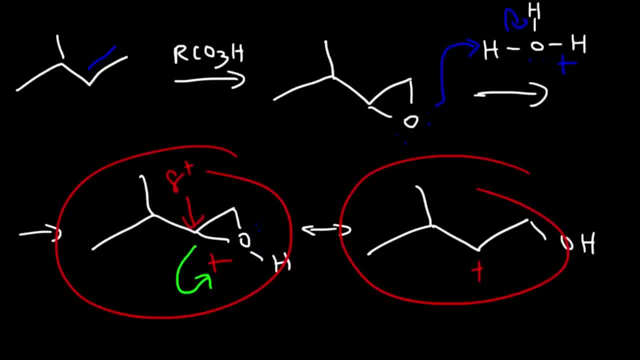 the resonance forms, then this one has to have significant partial positive charge, which means water is attracted to that carbon, so it's going to attack the secondary carbon and not the primary one. so we're going to have an OH group on this carbon and a water on the other one. 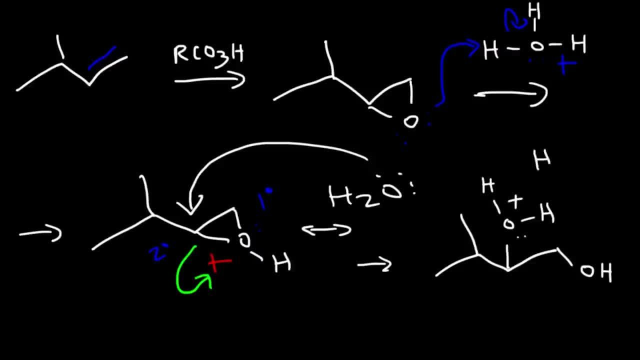 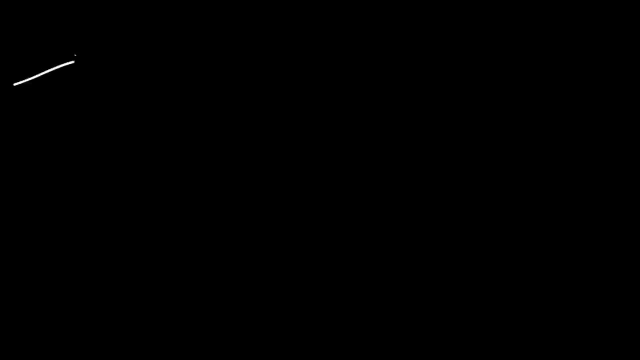 so now all we need to do is use another water molecule to get rid of one of the hydrogens, and so now we have a diol which occurs with anti addition, but that's not the product that we're looking for. now. let's focus on the oxy. 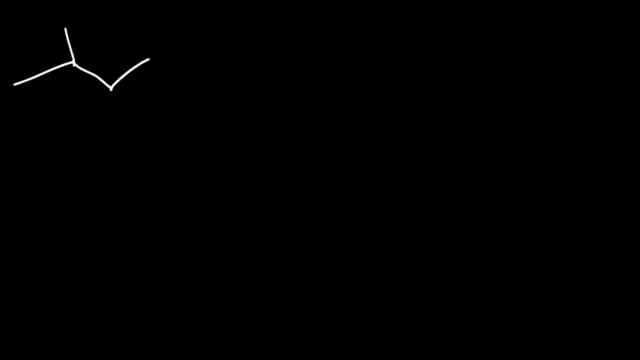 mercuration, de mercuration reaction. so the alkene will react with mercury acetate. the mercury atom has a lone pair. so the double bond is going to attack the mercury atom, causing one of the acetate groups to multiply. and then the double bond is going to attack the mercury atom, causing one of the acetate groups to 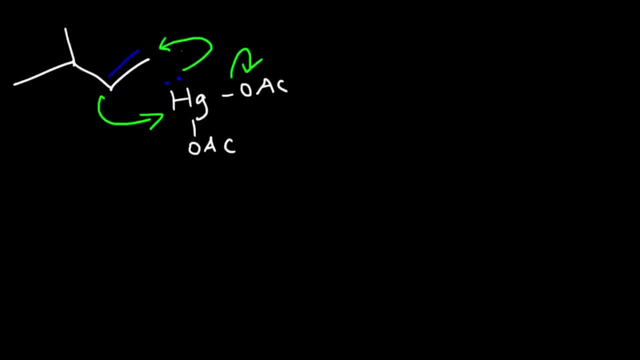 expelled and the lone pair on the mercury atom will simultaneously react with the double bond. So we're going to get this cyclic mercurinium ion, which looks like this: At this point, mercury has a positive charge, the acetate that was kicked out has a negative charge. Now this carbon, just like before in the 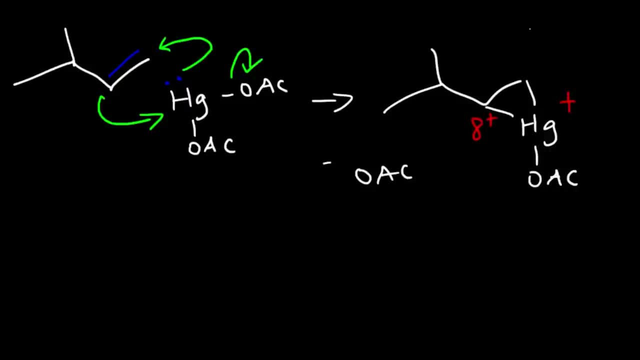 other example has a significant amount of partial positive charge, So the water that's in the reaction will be attracted to it, So it's going to attack from this side, causing this bond to break, And so the mercury atom is going to be on the primary carbon, On a secondary carbon. we have an oxygen Now. 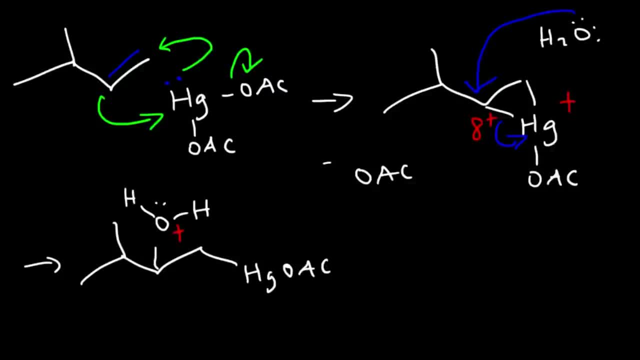 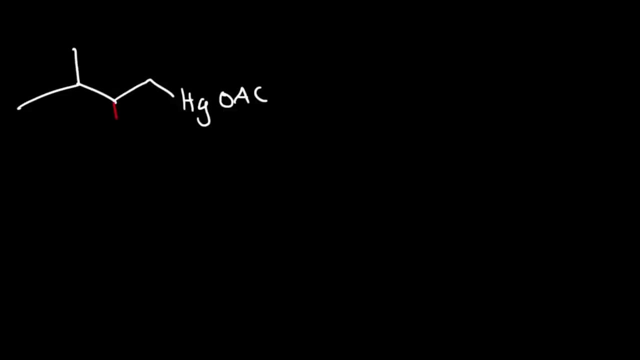 we need to remove the hydrogen. We can use water or, better yet, we can use acetate, which is a weak base. So now we have this intermediate And in the last step, we need to add sodium borohydride. Now, the mechanism for this step is not precisely known, but we do. 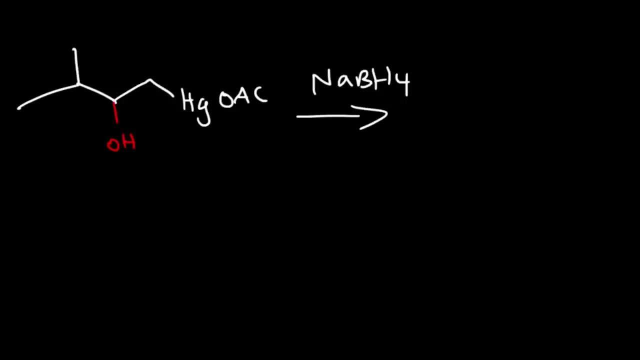 know the end result. The end result is that the mercury group will be replaced with hydrogen. Now, since we don't have to show the hydrogen, we could simply write the final product like this: It's 2-methyl, or rather 3-methyl 2-butanol, And so that's it. 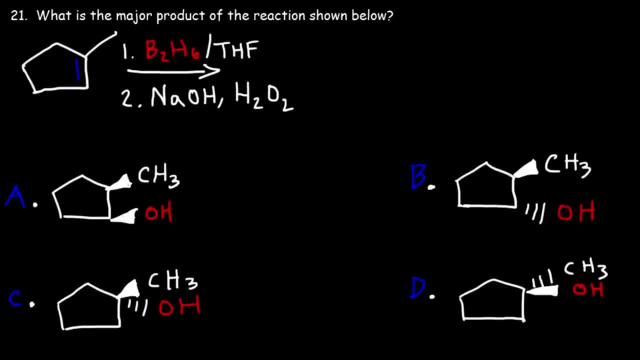 Number 21.. What is the major product of the reaction shown below? So we have a cycloalkene and a hydroboration oxygen, Hydroboration oxidation reaction. What do you think the major product is going to be? Well, first let's look at the VGO chemistry. We have a secondary carbon and 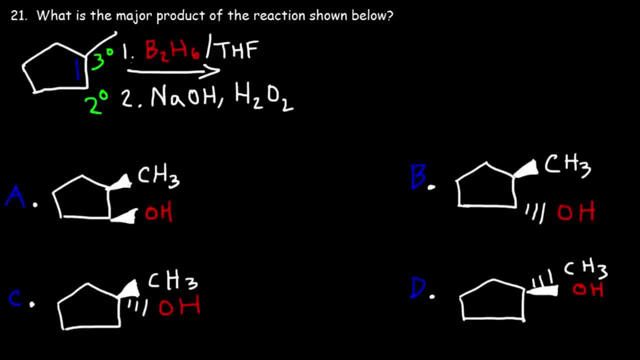 a tertiary carbon that are part of the double bond system. Now, the hydroboration oxidation reaction is an antimicrobial reaction, which means that the alcohol, the OH group, should be on the less substituted carbon, that is, the secondary carbon, In this instance an antimicrobial carbon addition reaction. So therefore C and D will 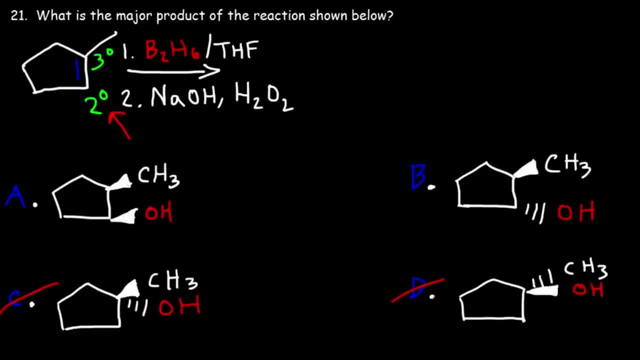 not be the answer, We can eliminate those two. So now let's move on from the VGO chemistry and let's analyze the steriochemistry of the reaction In answer choice A: the methyl group and the alcohol group, their cis with respect to each. 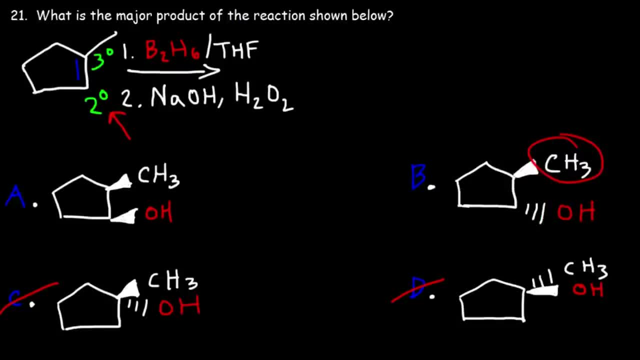 other. Here it's trans- Which one will be the right answer. So what we need to know is that the hydroploration oxidation reaction occurs with syn addition. Now, the syn addition, it doesn't have to do with the methyl group, because the methyl group 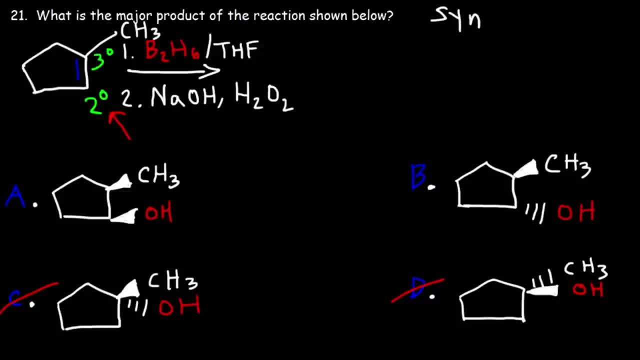 was already present in the reaction. The syn addition is between the hydrogen and the OH, So in both cases the methyl group is in the front. So let's re-write that Now we need to put the OH group on the secondary carbon and the hydrogen on the tertiary carbon. 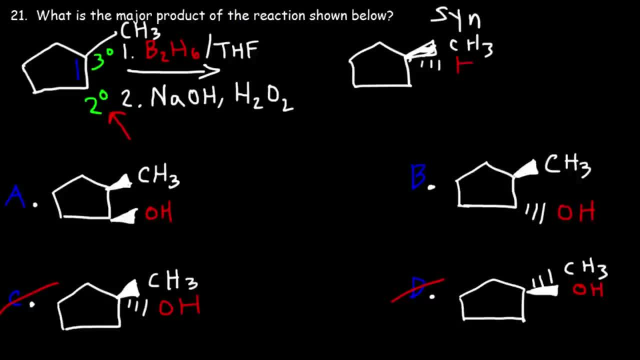 So the hydrogen has to be in the back. I'm going to put it in red. We're adding the hydrogen to it And because the OH group and the hydrogen has to be syn with respect to each other- meaning they have to be on the same side- the OH group has to be in the back. 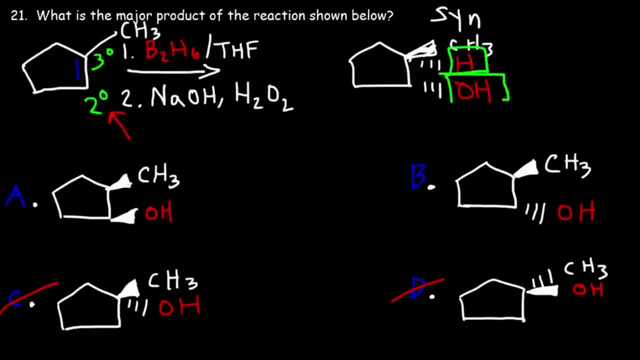 So this reaction, The reaction is syn addition with respect to the hydrogen and the OH group that are added across the double bond, But it's trans if you compare the OH group and the methyl group. So therefore, the correct answer is answer choice B. 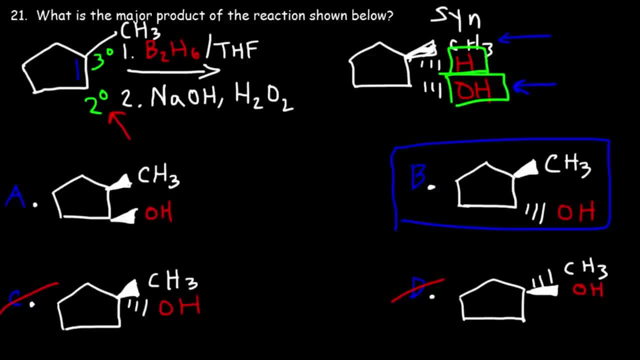 So the reaction is syn addition, but that's It's syn with respect to the H and the OH. It appears to be trans because you don't look at the hydrogen. It's syn with respect to the H and the OH. The hydrogen's not visible here. 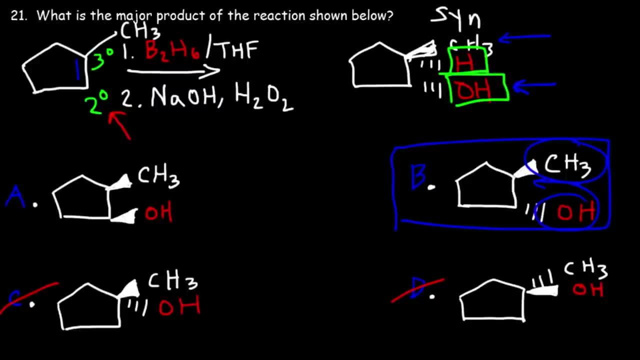 If you're just looking at the CH3 and the OH, it will be trans, But with respect to the hydrogen and the OH, those two groups should be on the same side. So B is the right answer for this problem, Number 22.. 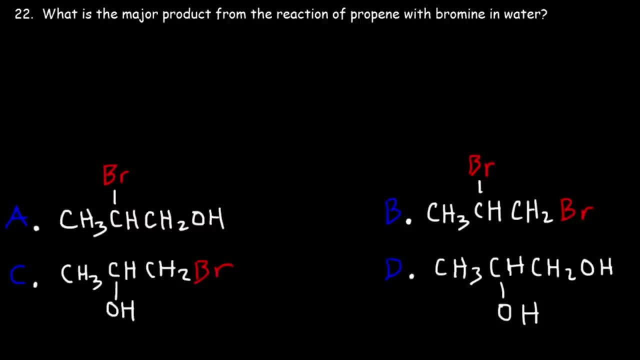 What is the major product from the reaction of propene with bromine and water? So propene has three carbons and a double bond, And so we're going to react it with Br2.. And so we're going to react it with Br2.. 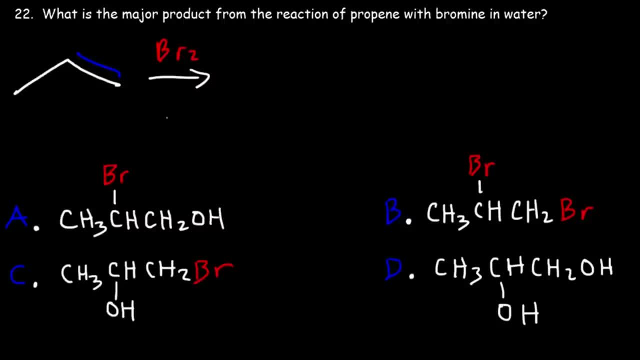 And so we're going to react it with Br2 and H2O. Whenever you react an alkyne with bromine and water, you're going to get two functional groups: You're going to get a bromine atom and you're going to get an OH group. 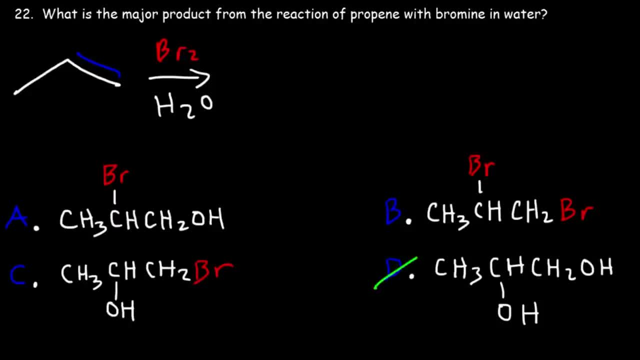 So we can eliminate answer choice D. We're not going to get two alcohol groups and we're not going to get two bromine atoms, So we're either between A or C. Now it turns out that the more electronegative atom goes. 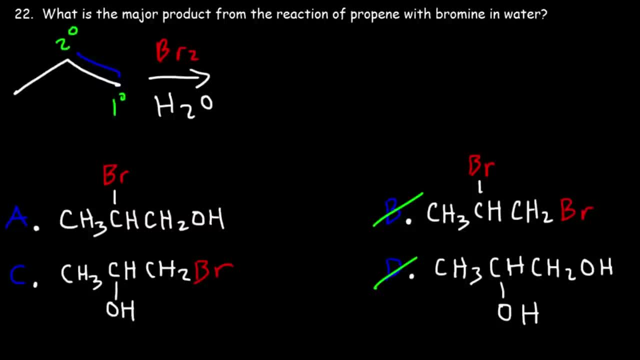 in the more substituted carbon. How do we measure that which is the OH group? So the OH group is going to go on a secondary carbon and the bromine is going to go on a primary carbon. So the correct answer is answer choice C. 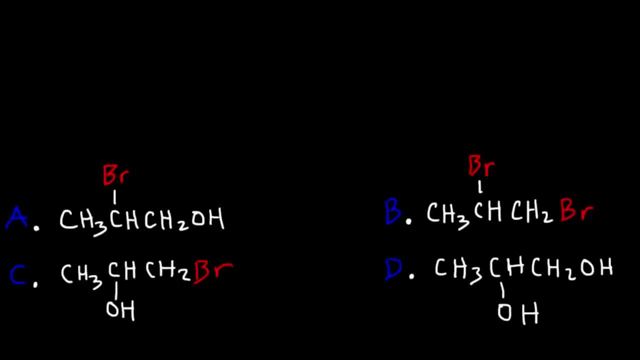 But let's write up a mechanism for this reaction. So the first thing that happens is that the alkene reacts with bromine. So the double bond is going to attack one of the bromine atoms, expelling the other, and at the same time bromine attacks the double bond. 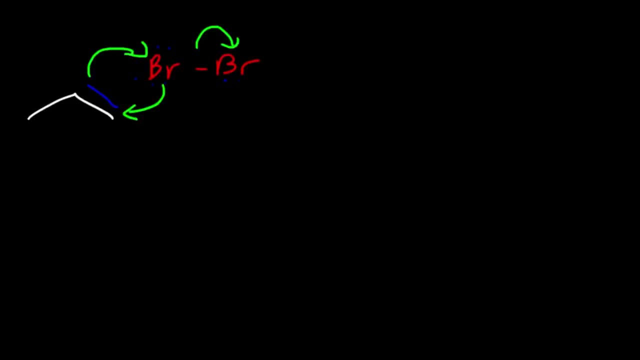 So initially bromine has three lone pairs And the bromine that gets attacked is going to use up one of its lone pairs. It's going to form a cyclic intermediate, so it's going to have two lone pairs left over And it's going to have a positive charge. 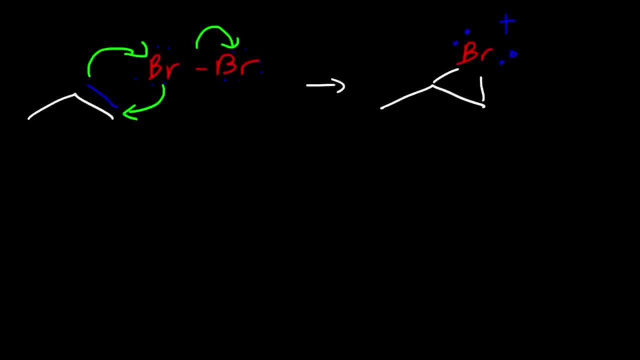 The other bromine atom leaves as bromide and it's going to have four lone pairs and a negative charge. Now we have water in the solution and because the reaction is dissolved in water, there's a lot more water molecules than bromide ions. 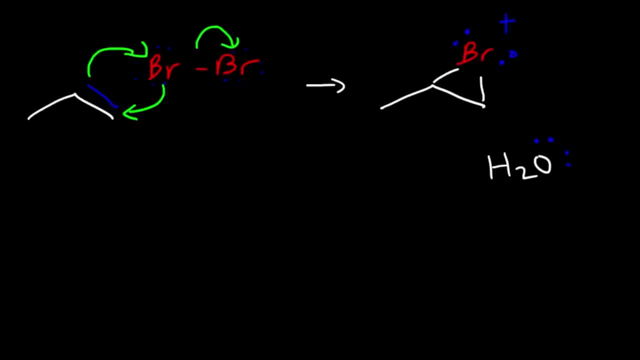 So water is going to attack the carbon. Now keep in mind there's considerable partial positive charge on the secondary carbon And water. it has an oxygen. for both It's going to have a partial negative charge. That oxygen is attracted to this partially positive carbon atom. 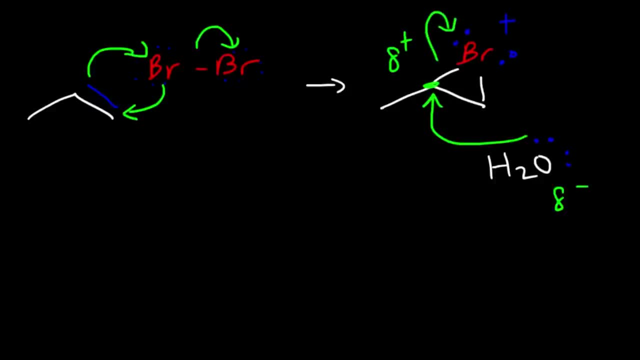 It's going to attack it from the back, expelling the bromine atom to the other side, And so that's why the oxygen is on the secondary carbon and the bromine is on the primary carbon. It's because of the backside attack. 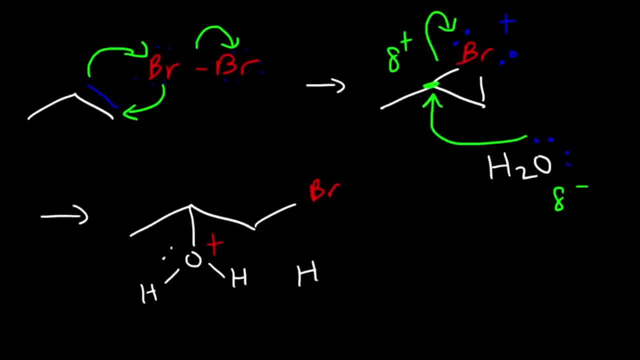 Now the oxygen has a positive charge. There's one more step in this reaction. We need to use another reaction. We need to use another water molecule to get rid of this hydrogen, And so this is going to be the product: It's 1-bromo-2-propanol. 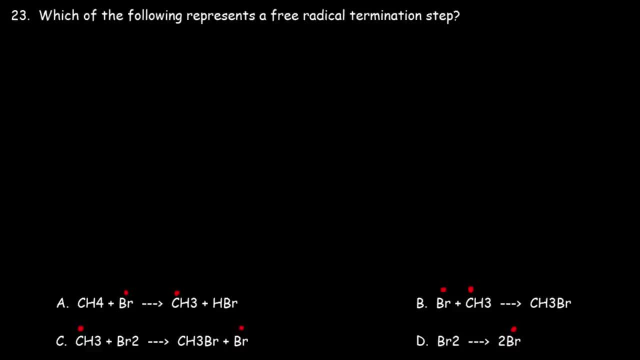 Number 23.. Which of the following represents a free, radical termination step? Is it going to be A, B, C or D? So here are some things that you need to know. Let's say if you have a reaction: A plus B turns into C plus D. 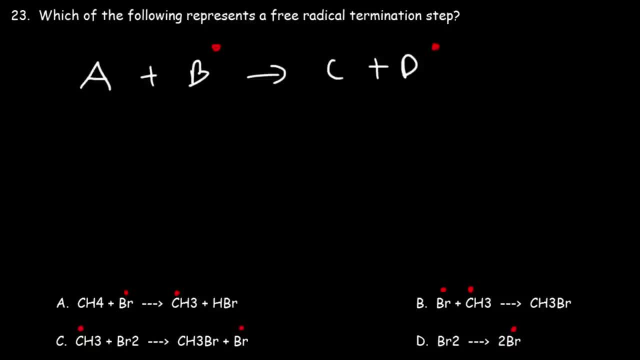 Any time you have two radicals, one on each side, this is going to be a propagation step. If you have a radical on the left and on the right side, Now, let's say, if you have two radicals on the left side, this is going to be a termination step. 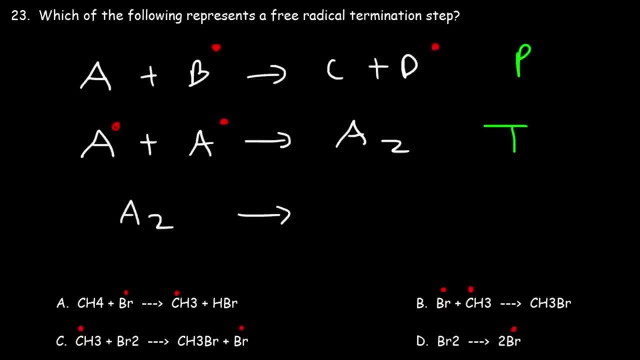 And if you have two radicals on the right side as opposed to the left side, this is an initiation step And that's a quick and simple technique to distinguish initiation from propagation and from termination. So we're looking for a termination step, So we're looking for the reaction that has two radicals on the left side. 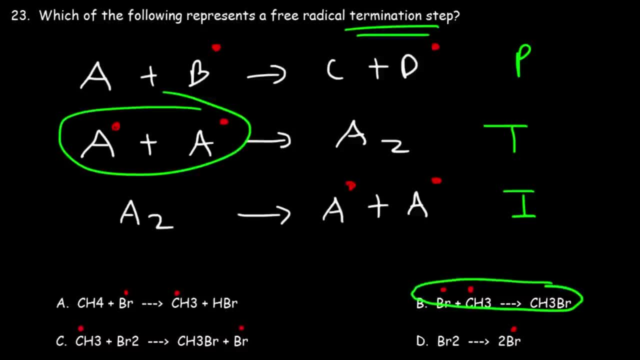 So answer choice B fits that description. So B is the answer. B is a termination step. Now look at answer choice A. Is it initiation or propagation? Because there's a radical on the left and on the right side, it's a propagation step. 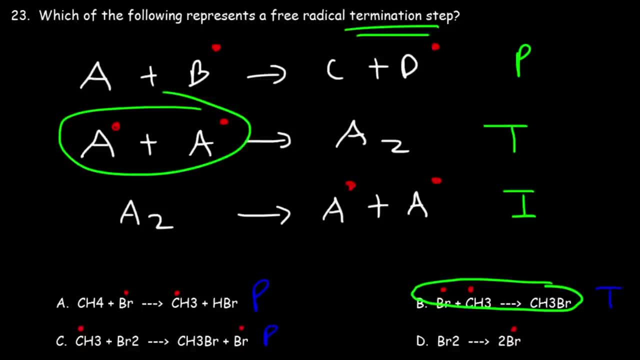 The same is true for C. Look at answer choice D. We have two radicals on the right side, So that's an initiation step, And so that's it for this problem, Number 24.. What is the major product of the reaction shown below? 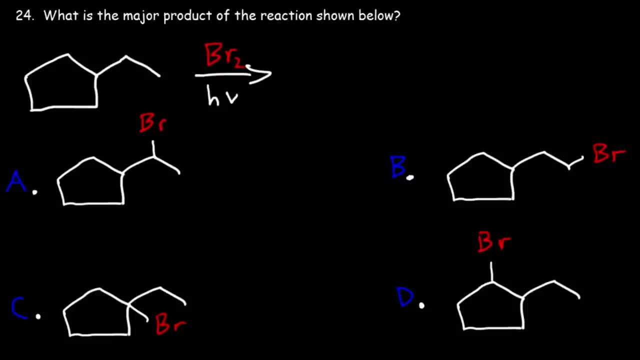 Is it A, B, C or D? Now, what you need to know for this type of problem is that when you mix bromine with HV- either UV light or even heat- it's going to be a radical reaction. And whenever you have a halogen reacting with an alkane. 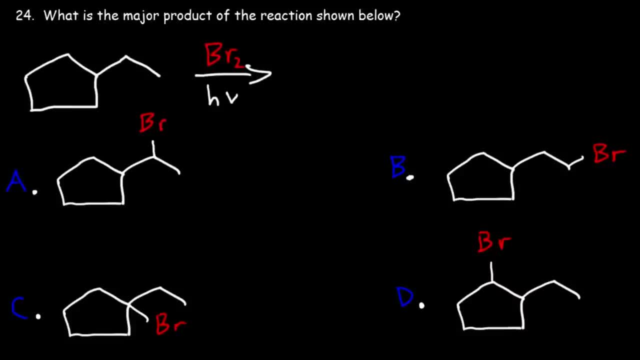 this is an alkane. under radical conditions, the bromine is going to replace the most substituted hydrogen. So if you have a primary hydrogen, a secondary hydrogen and a tertiary hydrogen, it's going to replace the tertiary hydrogen. Now we do have a tertiary carbon. 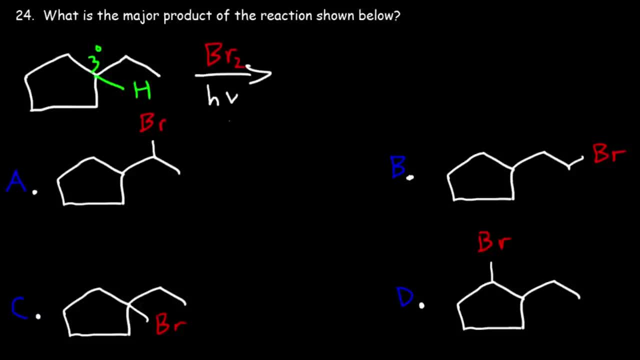 This carbon is tertiary, which means the hydrogen attached to it is tertiary. So bromine is very selective. It's going to go for the tertiary hydrogen. Now, if we had chlorine, chlorine is non-selective. It's going to go for any hydrogen that it can get its hand on. 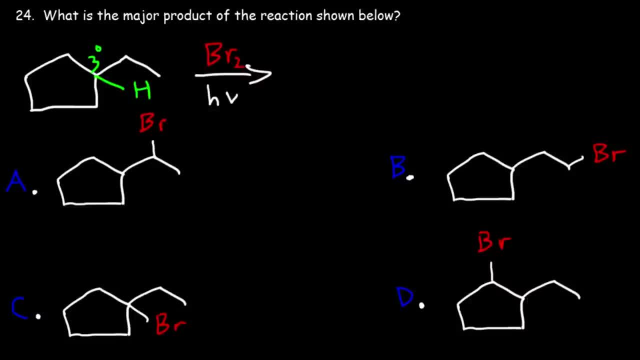 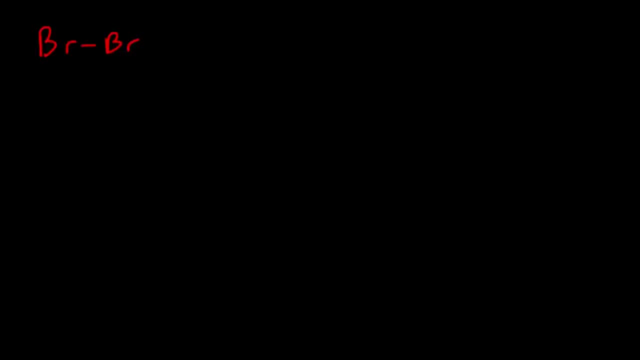 It's very reactive. Bromine is less reactive, more selective, So it's going to replace the tertiary hydrogen, which means that C is the right answer. Now let's go over the mechanism of that reaction. So the first thing that happens once we add UV light: 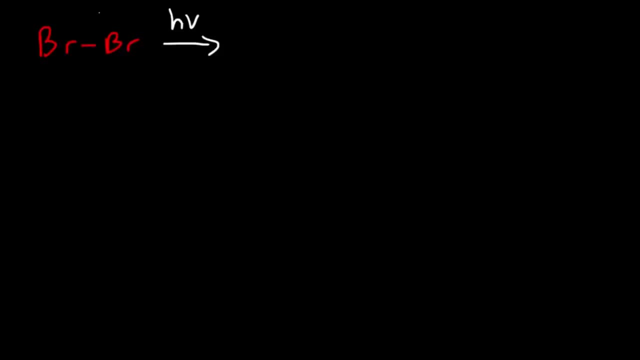 the bromine molecule is going to split into two parts Once it gains enough energy. each bromine atom is going to take one electron and the two electrons in that box. So we're going to get two bromine radicals Once we generate the bromine radical. 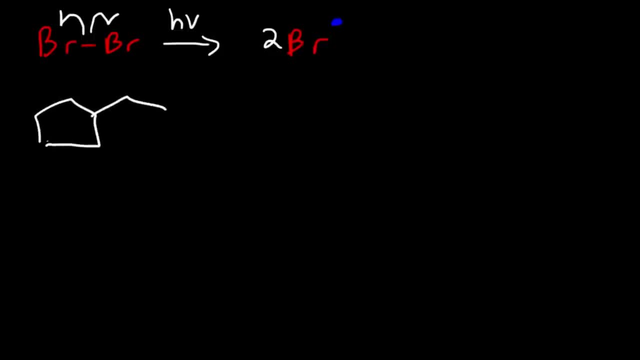 in that initiation step. the next step is going to be a propagation step. The bromine radical is going to react with the tertiary hydrogen. So there's two electrons in this bond. One of those electrons will be used to form the bond between H and Br. 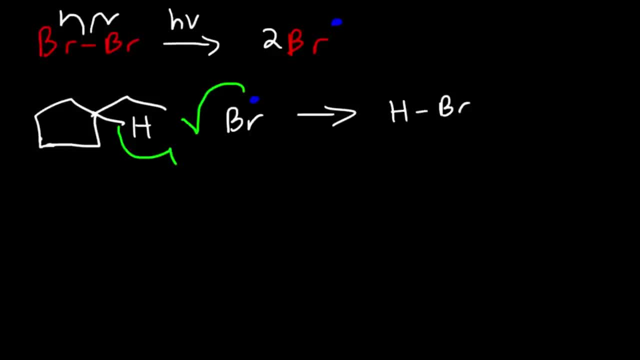 So that's going to be a side product. The other electron it's going to stay on the tertiary carbon, So we're going to get a tertiary radical. Now this radical, we can react it with another bromine molecule, since we have plenty of them in the reaction. 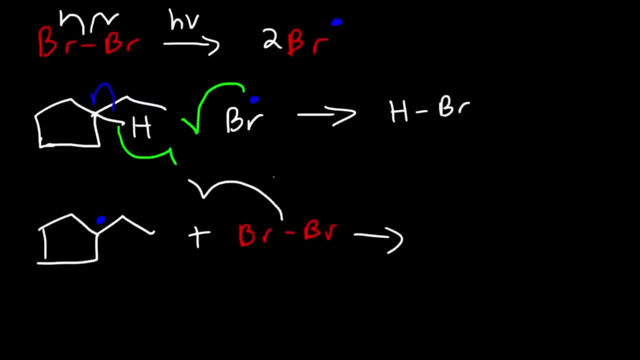 So one of the electrons in the bond between the two bromine atoms will react with the radical, giving us the product. The other bromine atom is going to take the other electron with it, regenerating the bromine radical. So that is a propagation step. 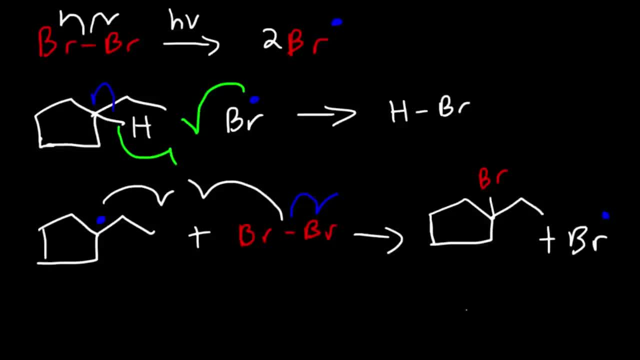 since we have one radical on the left and one on the right. Alternatively, we can get the same product using a termination step, So we can start with the tertiary radical and react it with a bromine radical. So these two would simply combine. 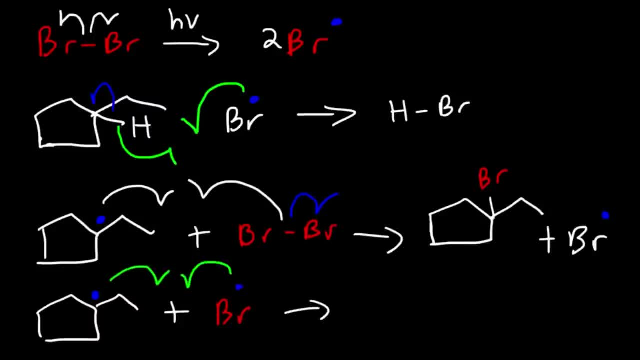 And keep in mind when dealing with radical reactions. typically, you're going to be using half arrows, which represents the flow of one electron. A full arrow represents the flow of two electrons, And so those are the different ways that you can get the product. 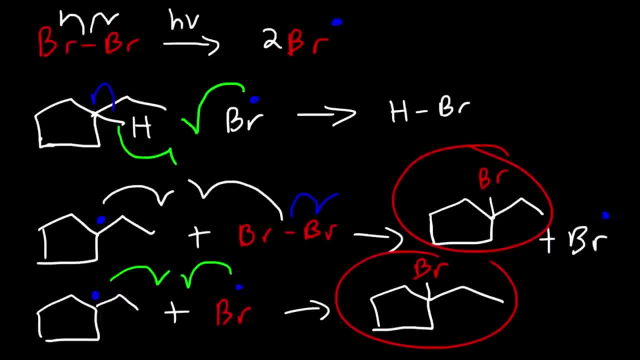 You can get it through a propagation step or even a termination step. The propagation step is more likely because there's a lot more bromine molecules than bromine radicals. The amount of bromine radicals in a solution is very small, So this step. 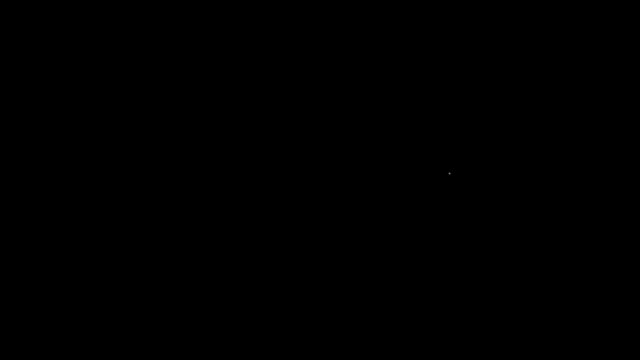 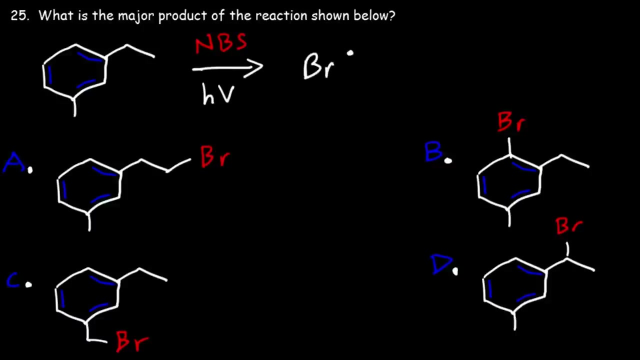 will occur more frequently. 25: What is the major product of the reaction shown below? NBS with heat or light works the same way as Br2 of HV. NBS produces radical bromine very slowly when activated with heat or light. So we know that the radical bromine 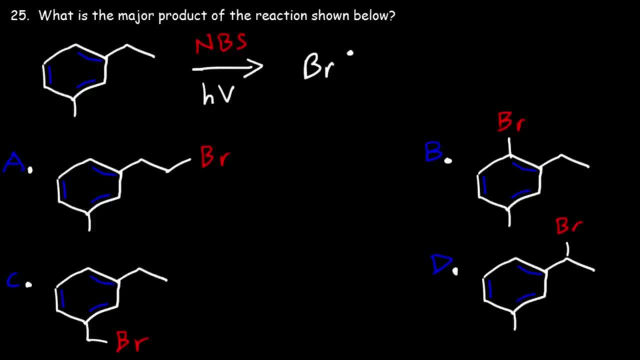 is going to replace the hydrogen. that will lead to the most stable radical. In the last example, the reason why it went for the tertiary hydrogen is because of the stability of a tertiary radical. A tertiary radical is more stable than a secondary radical, which is more stable than a primary radical. 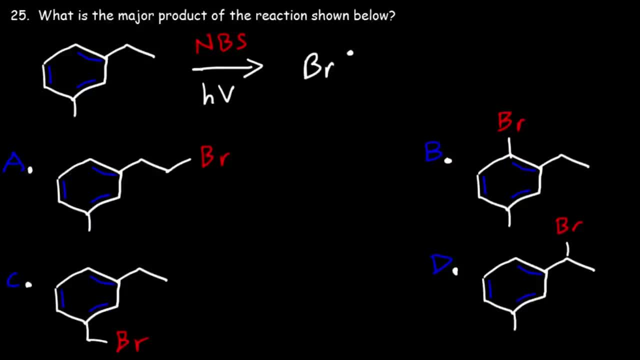 So what we need to do is figure out which radical is more stable. Looking at answer choice A, the bromine is on this carbon. So let's say, if we take away the bromine atom and just simply put a radical there, Will that radical be the most stable radical? 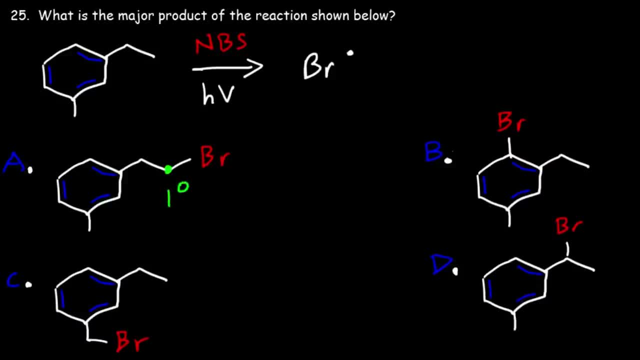 If we take away bromine, that's going to be a primary radical Here. if we take away the bromine, it's a vanillic radical. Vanillic radicals are not stable, so we can eliminate answer choice B. Now if we put it here, 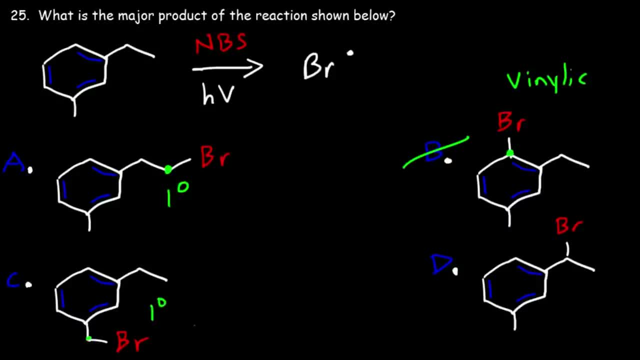 this is going to be a primary radical, but because it's one carbon away from the benzene ring, it's a benzylic radical, which means that it's stabilized by resonance. So C is a good answer. but if you look at D, 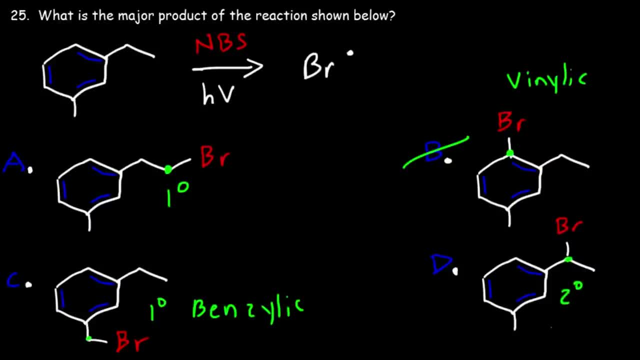 it's a secondary radical and because it's one carbon away from the benzene ring, it's also benzylic. It turns out that you can get a mixture of C and D. However, the question was the major product of the reaction. 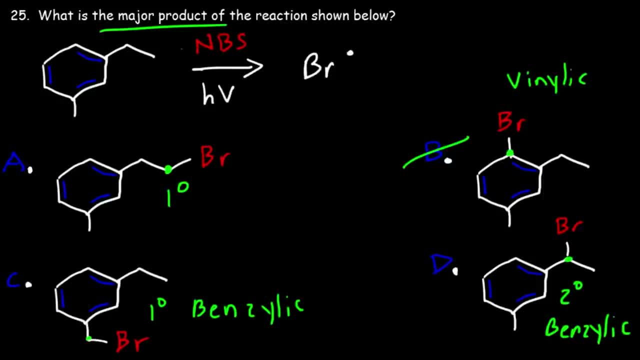 Because a secondary benzylic radical is more stable than a primary benzylic radical. D is going to be the answer. The major product is D, The minor product is C. You won't get A or B, and if you do get it, 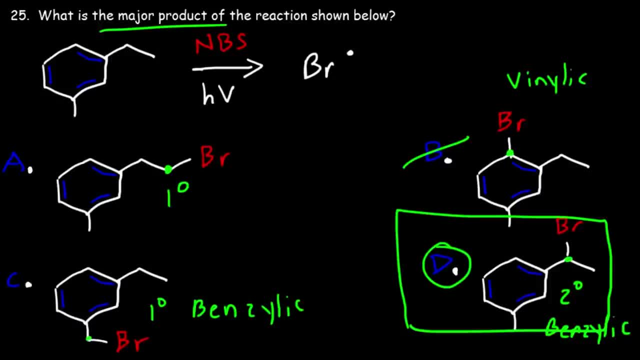 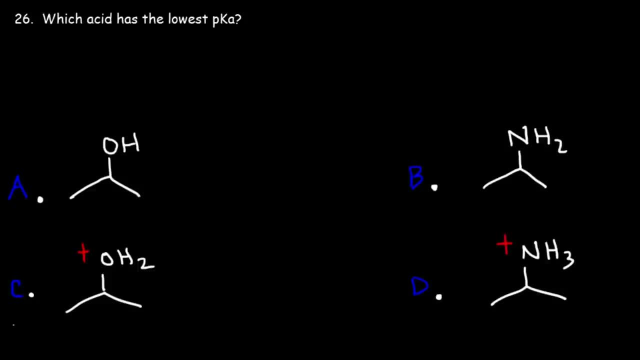 it's going to be very, very, very, very low, But D is the answer Number 26.. Which acid has the lowest pKa? Is it going to be A, B, C or D? So how can we find the answer? Well, we can use the trend on a periodic table. As you travel from A to B, from left to right, acidity increases due to increase in electronegativity. So an OH group is always more acidic than an NH2 group. Keep in mind, the typical pKa of an alcohol is 16 to 18. And for an amine it can be anywhere from 35 to 40. So we're looking for the one with the lowest pKa. We're looking for the strongest acid. 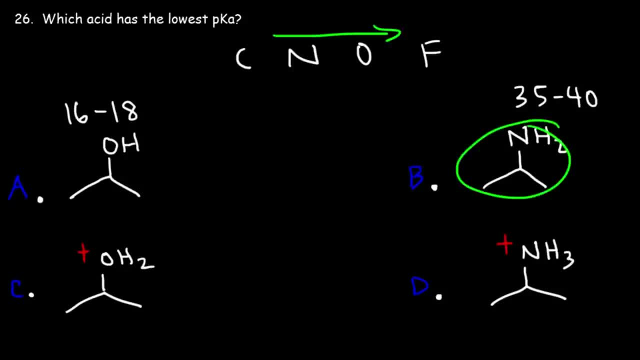 Now which one is more acidic- An amine or a protonated amine? Any time you add a hydrogen to something, the one with the positive charge is going to be more acidic than the neutral one. A protonated amine has a pKa of about 9 to 10.. 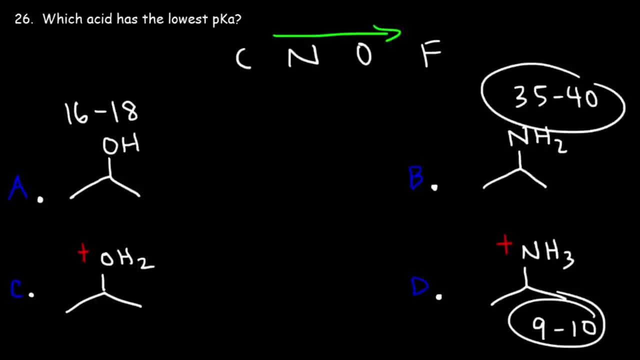 As you can see, this is much lower than this one, So we can eliminate answer choice B. And the protonated amine is more acidic than the alcohol, so we can get rid of A. Now the protonated alcohol is even more acidic. 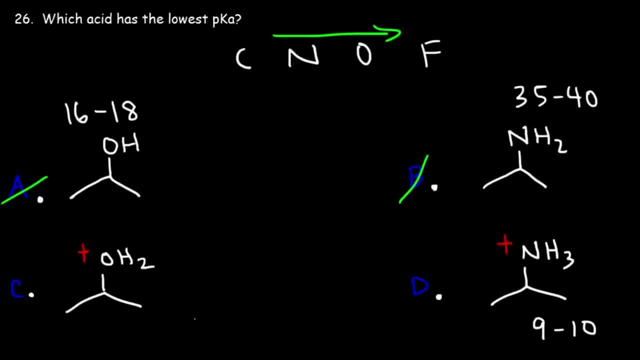 If OH is more acidic than NH2, then OH2 must be more acidic than NH3+, So clearly the correct answer is C. A protonated alcohol has a pKa somewhere in the negative range. It could be like negative 2 or negative 3,. 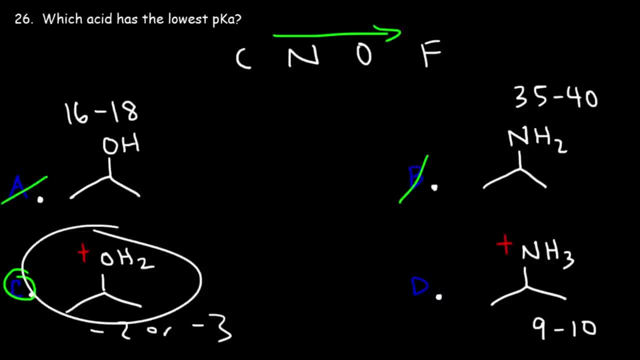 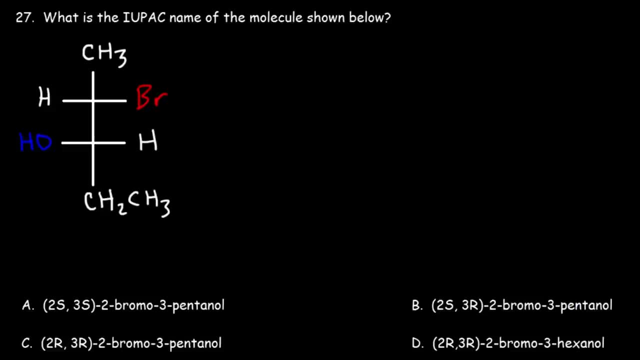 but it's very acidic. So this is the answer, Number 27.. What is the IUPAC name of the molecule shown below? So first let's identify the longest chain. So this is going to be carbon 1,. 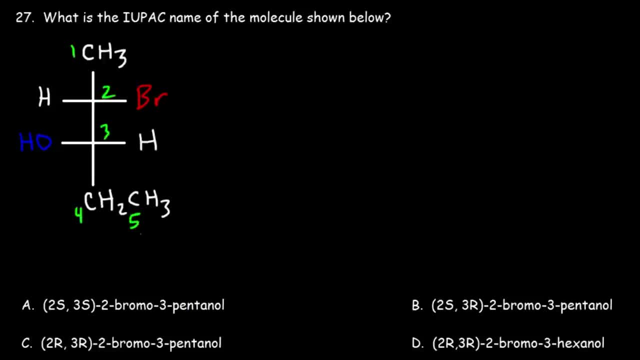 2,, 3,, 4, 5.. We want to count it in that direction so we can get a 2-bromo and the alcohol in 3.. If we count it the other direction, we're still going to get the OH on 3,. 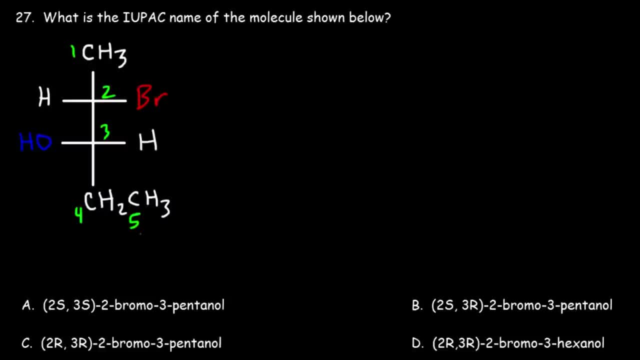 but the bromine will be on 4.. And you want to count it in such a way to get the lowest numbers, So we want to count it from the top to the bottom. So there's 5 carbons and the functional group is in alcohol. 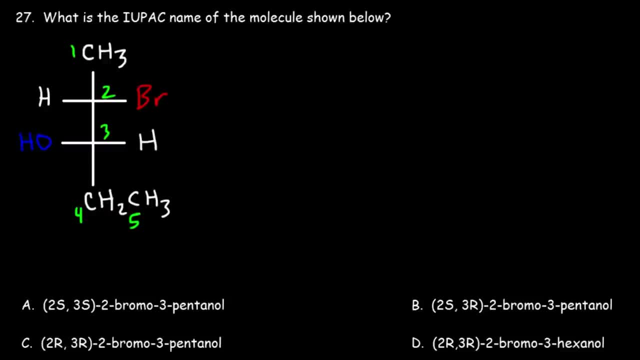 so it's pentanol, which means that we can eliminate answer choice D. So everything else is the same: 2-bromo 3-pentanol. The only thing that's different is the configuration, So we need to determine. 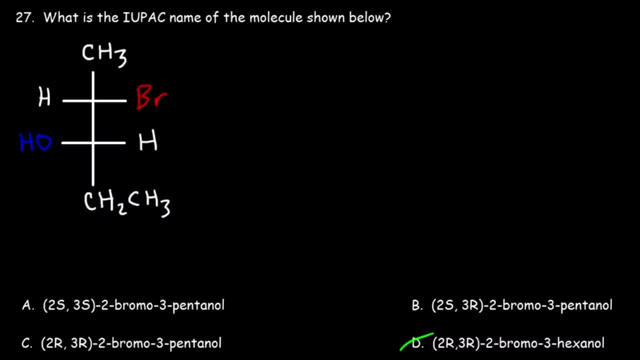 if we have an R or an S isomer. So let's start with this chiral center, carbon number 2.. Now we know that the hydrogen is group number 4. It has the lowest priority. Bromine has the highest. 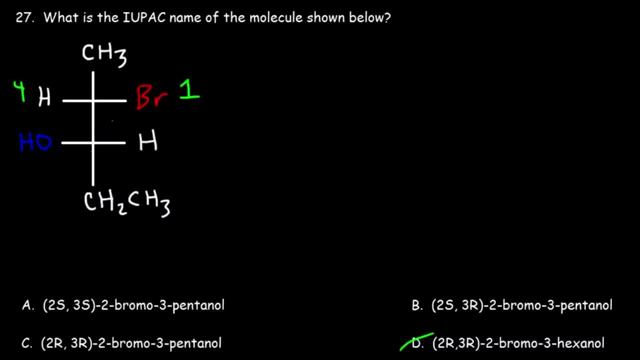 This entire group here is going to be group number 2.. And then number 3 is the methyl group. Now, what you need to know when dealing with a Fischer projection is that the groups on the sides, in this case the H and the Br. 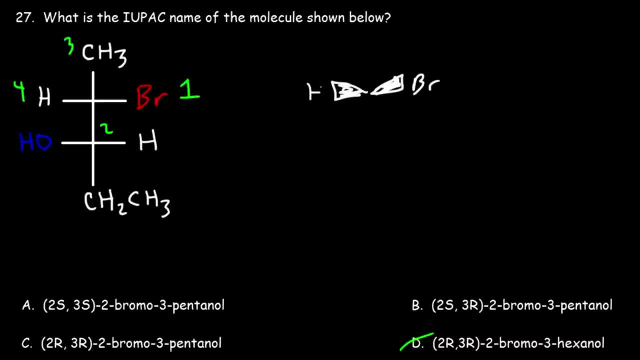 they're in the front, So we need to reverse it. The group above and below they're in the back. So keep that in mind. Now let's go ahead and count it, So starting from 1, going towards 2,. 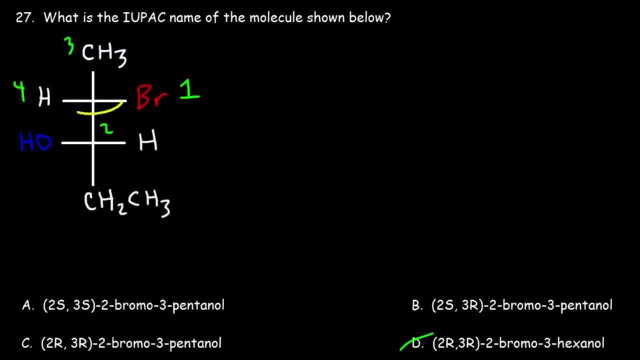 and skipping 4, go from 1 to 2 to 3.. If we travel from 1 to 2 to 3, notice that we're rotating in the clockwise direction, which would indicate R, But because H number 4,. 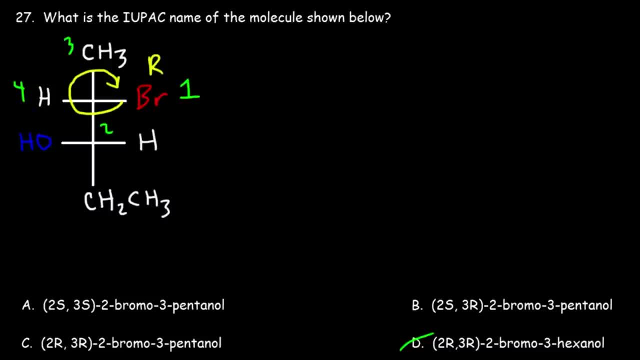 is in the front, we need to reverse it. So therefore, this is going counterclockwise or opposite to the direction of a clock. Therefore, this is the S isomer. So on carbon 2, keep in mind, this is carbon 2,. 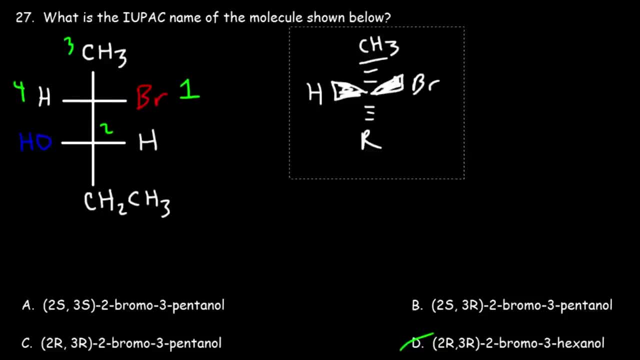 this is carbon 3.. On carbon 2, we have an S configuration, So therefore it's not going to be 2R, It has to be 2S. So now the last thing we need to do is find out the other chiral center. 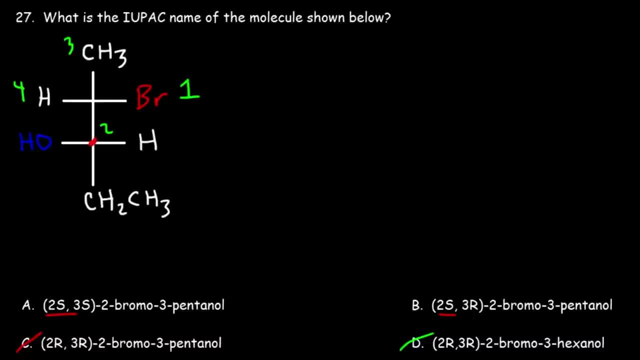 if it's R or S, So OH has the highest priority. If you compare this group with this carbon, oxygen has a higher atomic number. Next, if we compare this carbon and this one, there's no difference. So we've got to move on to the next group. 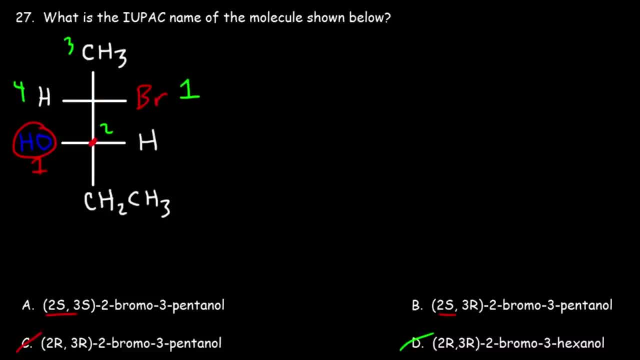 Bromine has a higher atomic number than the second carbon. So this entire group above that's going to be- let's call it- group- number 2.. H is number 4, and the ethyl group is number 3.. So counting it from 1 to 2 to 3,, 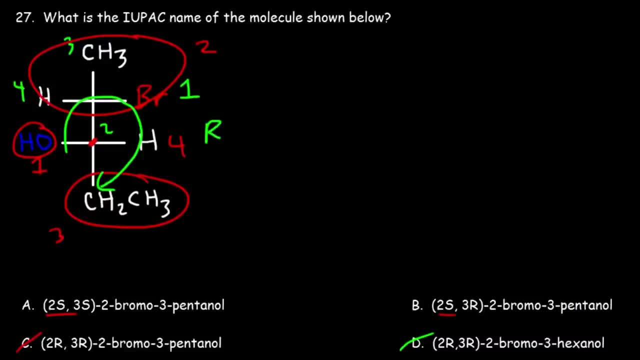 ignoring 4,. this appears to be the R isomer, But we need to reverse it, since group number 4,, in this case the hydrogen, is in the front. So because it's in the front, we're going to reverse it. 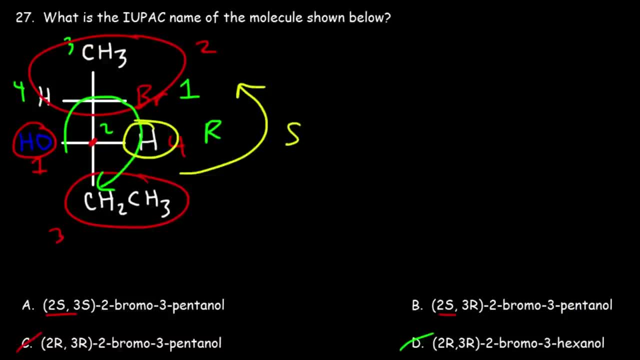 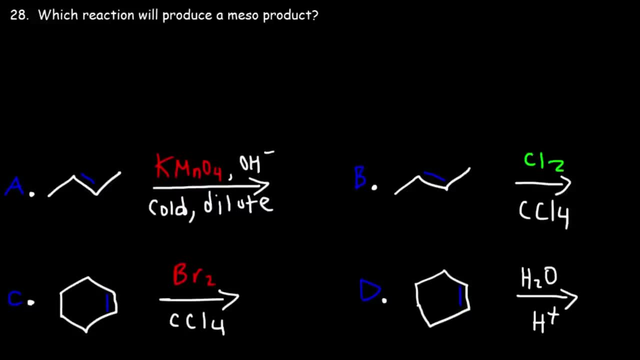 and now it's going to be S, So it's 2S and 3S. Therefore, answer choice A is the right answer, Number 28.. Which reaction will produce a mesoproduct? Go ahead and pause the video. 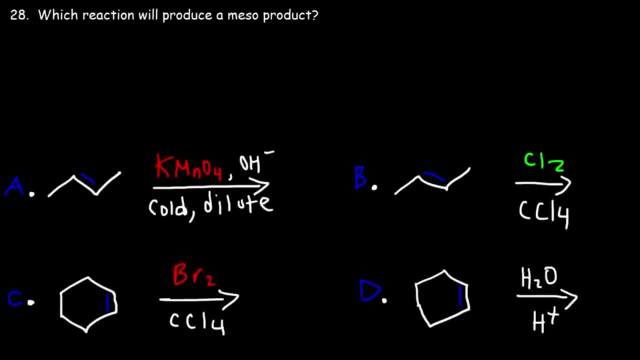 Work on this problem, It turns out that the answer is B. Now let's talk about why. Let's go through each one. So here are a few things that you need to know. Let's say, if you have a cis, alkene. 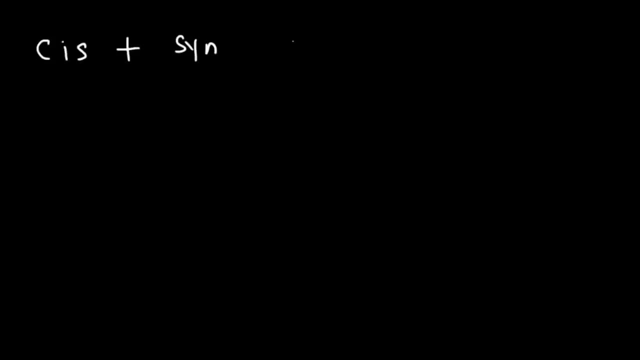 plus a syn addition reaction, this will lead to a mesoproduct. if the product has a line of symmetry- so that's important- If it doesn't have a line of symmetry, then this will lead to a pair of enantiomers or potentially even diastereomers. 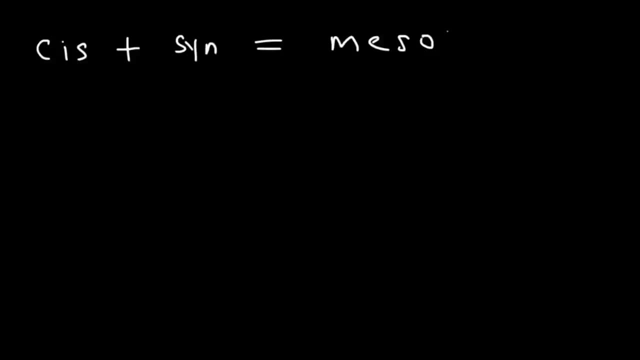 depending on the structure. But let's assume that we do have a line of symmetry for all of these examples, It's going to be a mesoproduct. Now, if we have a cis alkene and, let's say, an anti-addition reaction, 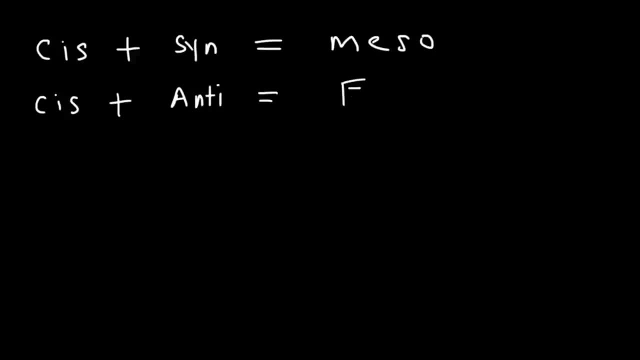 this will lead to a pair of enantiomers. So I'm going to write EN for enantiomers. Now, let's say, if we have a trans alkene plus, let's say, a syn addition reaction, This will also lead to a pair of enantiomers. 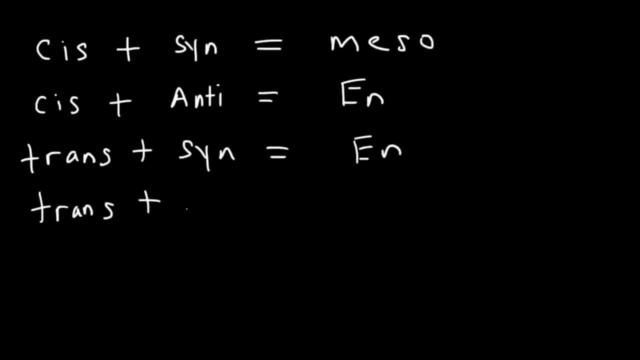 And if we have a trans alkene plus an anti-addition reaction, this will lead to a mesoproduct, if there's a line of symmetry. So let's consider the first reaction. So here we have a trans alkene and we're going to react it with potassium. 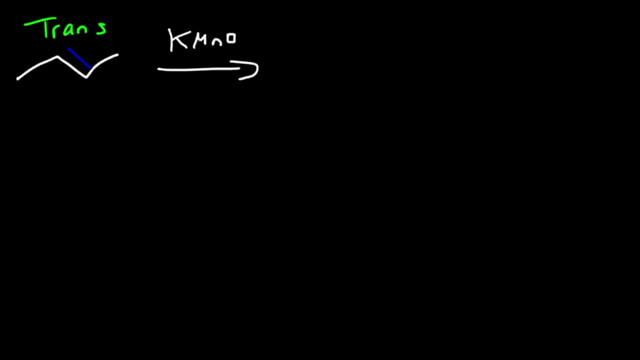 permanganate under basic conditions as indicated by the base hydroxide. The temperature's going to be low and the concentration is also low. So this reaction under cold, dilute conditions will produce a diol And this is a syn addition reaction. 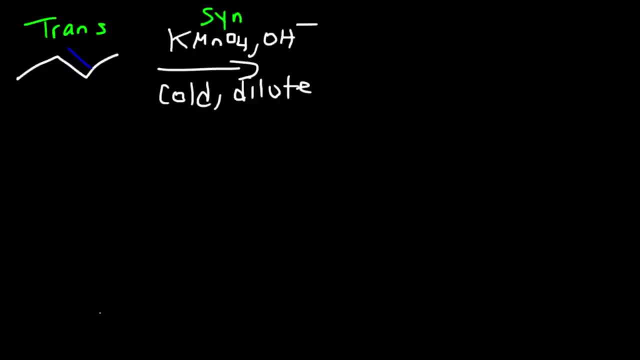 So the two alcohol groups will be on the same side. So this is going to be the product, But notice that we don't have a line of symmetry And a trans alkene plus a syn addition reaction would lead to a pair of enantiomers. 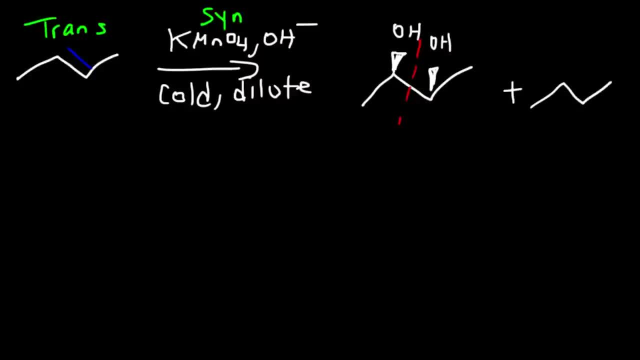 So the other product that you can draw will look like this. So we get a mixture of two products for this reaction. So that's how we can eliminate answer choice A. Now let's focus on answer choice C. We'll get back to B later. 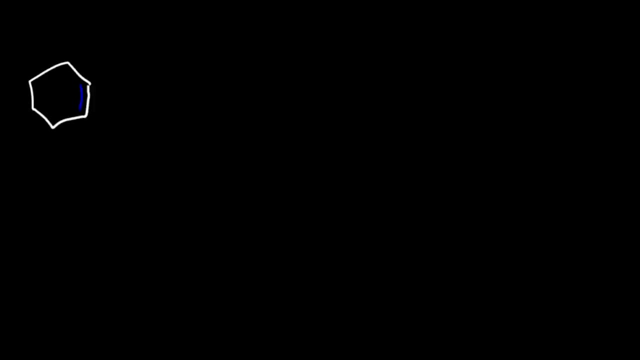 So we have cyclohexene, which you can view it as a cis alkene, And we're going to react it with bromine and carbon tetrachloride. The solvent, carbon tetrachloride, is inert, so you don't have to worry about it. 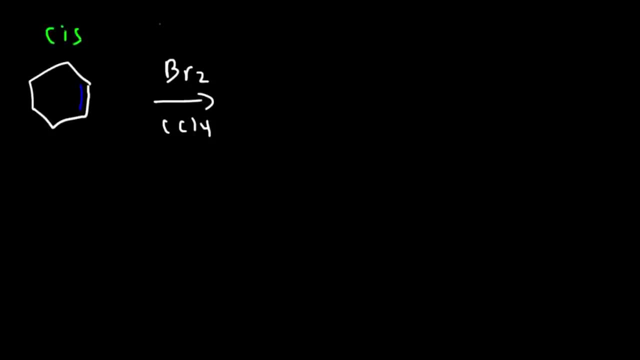 So we have a cis alkene and an anti addition reaction. This will lead to a pair of enantiomers. Because it's anti, we're going to put one bromine atom in the front and the other in the back And, as you can see, we do not have. 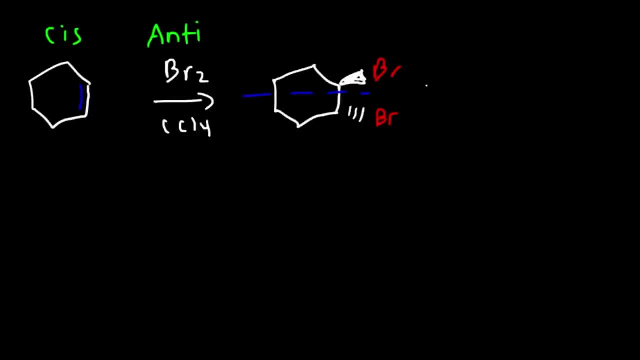 a line of symmetry. To draw the enantiomer, simply reverse the chiral centers, And so this is going to be the product of this reaction. Now let's move on to part C. So this time we're going to react. 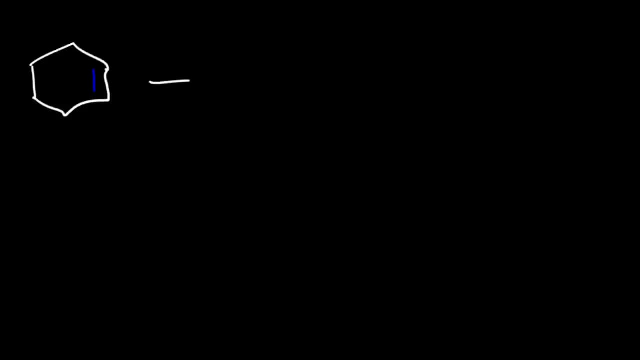 cyclohexene with water under acidic conditions, which is equivalent to H3O+. So the only thing that's going to happen is the alkene will be replaced with an alcohol And we're going to add one OH group And, as we can see, the carbon that has the OH. 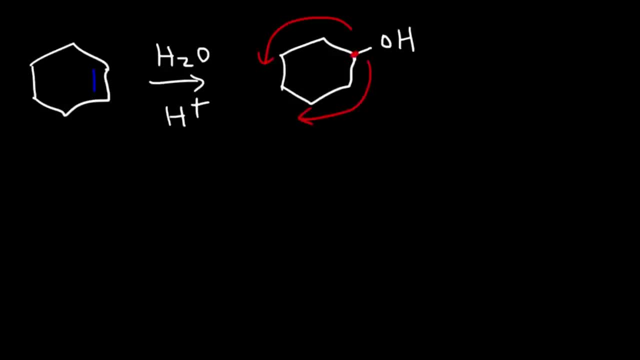 group is not chiral. The left side is equivalent to the right side, So therefore we get a single product And it's not a mesoproduct. We only have one chiral center. We don't have two chiral centers. 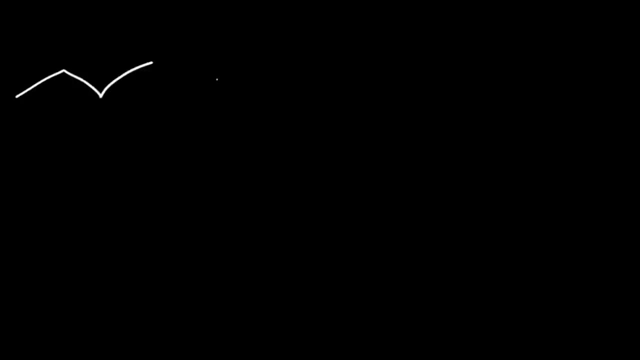 Now let's talk about answer choice B, which is the answer. So we have a trans alkene and an anti emission reaction. This will lead to a mesoproduct if it is applying, excuse me, a line of symmetry. So one chlorine atom, we're going to put it in the front. 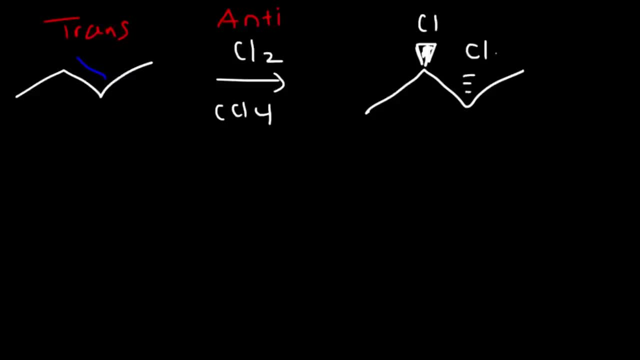 and the other one. we're going to put it in the back, facing the same direction. initially. Now single bonds have free rotation so we can draw a different conformant. So if we change the conformation by rotating this molecule, 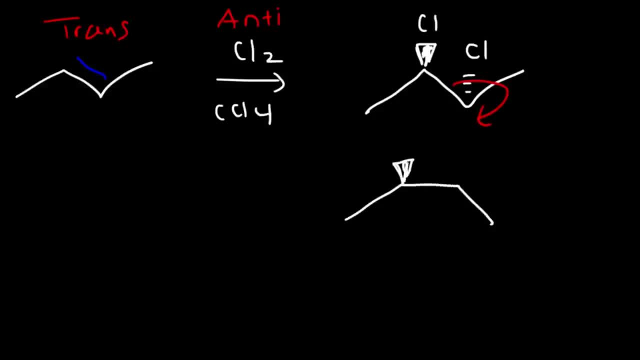 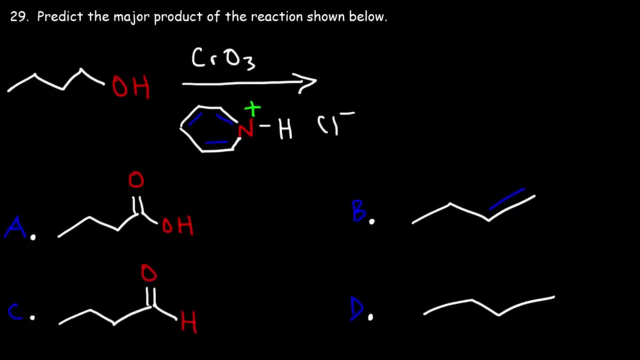 we get a mesoproduct. The Cl that was in the back is now in the front, And so notice that we do have a line of symmetry, Which means that this is a mesoproduct Number 29.. Predict the major product of the reaction. 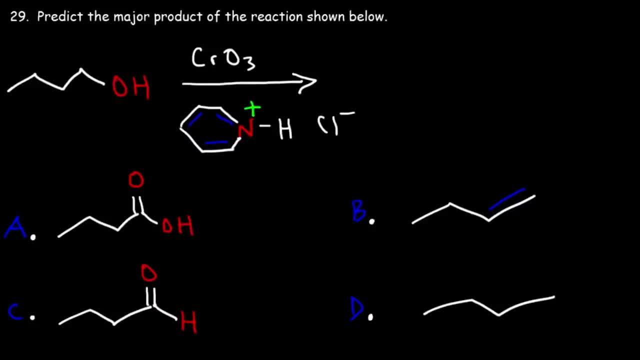 shown below. So we're reacting one butanol with pyridinium chlorochromate, So we have a primary alcohol. and which of these products will be the product of the reaction? Are we going to get a carboxylic acid? 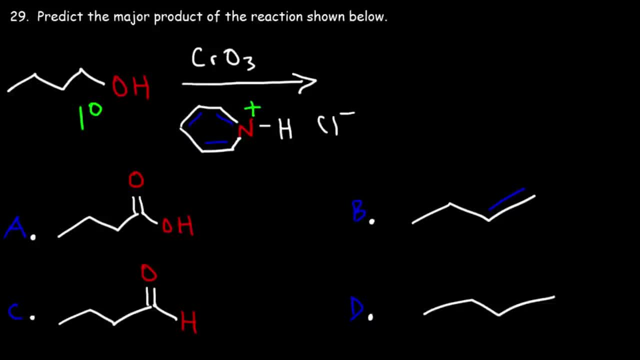 an aldehyde, an alkene or an alkane. Chromium trioxide is an oxidizing agent, so it won't be reduced into an alkane and we're not going to get an alkene. It turns out that this entire reagent is equivalent. 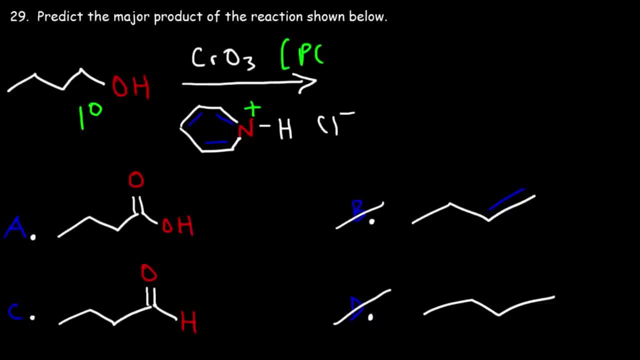 to PCC. PCC converts the primary alcohols into aldehydes. Now you don't need to know the mechanism of this reaction, but you simply need to know what this reagent will do If you have a secondary alcohol. 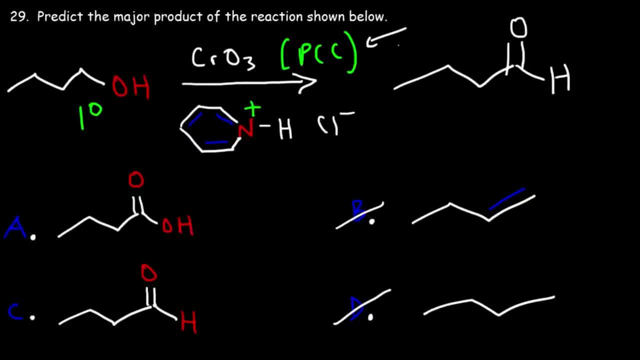 it can oxidize it into a ketone, But know that it will convert a primary alcohol into an aldehyde. So C is the answer. PCC is a mild oxidizing agent. Now, if you have a strong oxidizing agent, 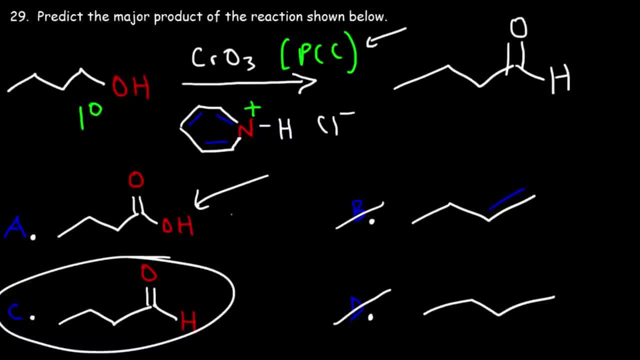 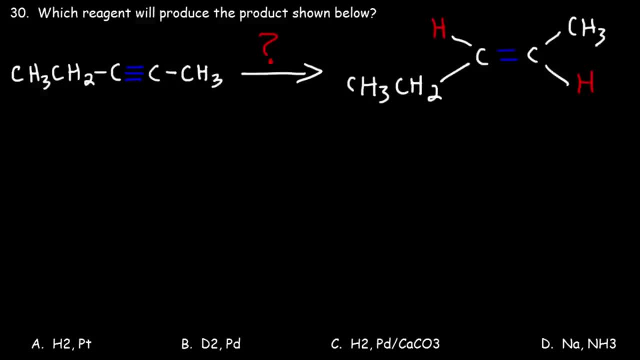 it can oxidize the primary alcohol to a carboxylic acid, But PCC won't take it that far. Number 30. Which reagent will produce the product shown below? Is it going to be A hydrogen gas with a platinum catalyst? 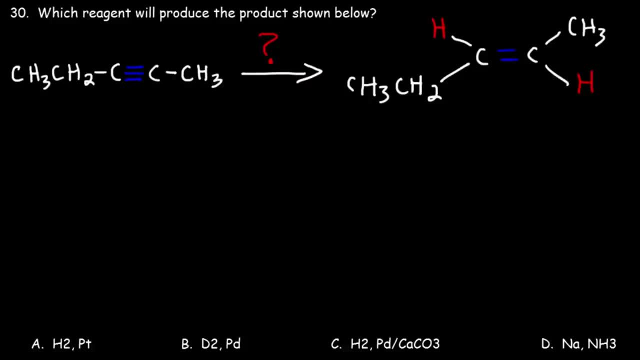 B- deuterium gas with a palladium catalyst, C- hydrogen gas with palladium mixed with calcium carbonate, Or D sodium metal mixed with liquid ammonia, Which one will convert the alkyne into a transalkene. So we can draw the alkyne. like this. So the alkyne has 5 carbon atoms. Let's call this carbon 1,, 2,, 3,, 4, and 5.. Now what's going to happen if we add hydrogen gas with a platinum catalyst? 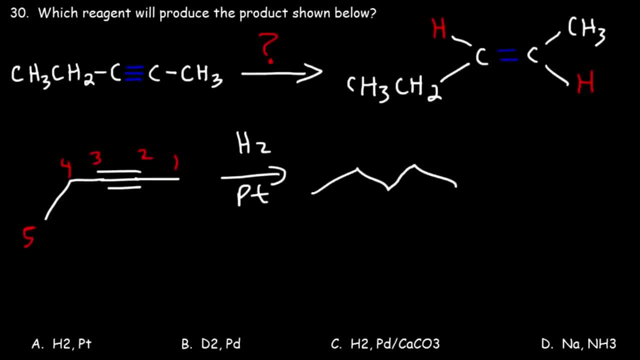 This will simply convert it to a 5 carbon alkane, So we can eliminate answer choice A. Now what about answer choice B? What if we add deuterium? and what's going to happen if we use a palladium catalyst? Well, this will be reduced to an alkane, but by means of the addition of deuterium atoms instead of hydrogen atoms. To convert the alkyne to an alkane first we need to add two deuterium atoms. Now it won't stop here. 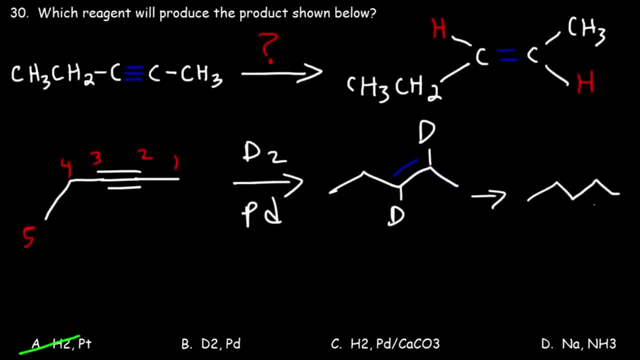 This will continue to continue To go from the alkane to an alkane. we need to add two additional deuterium atoms, So this is going to be the product of answer choice B, which is not the answer that we're looking for. 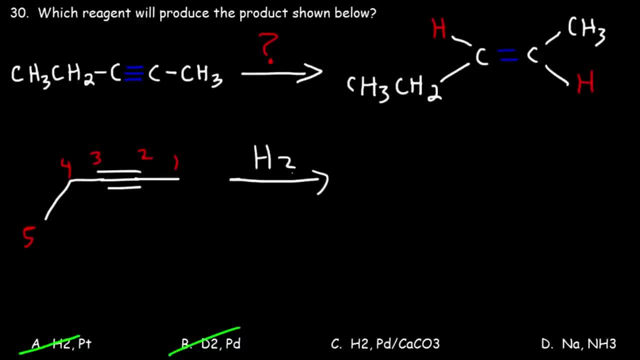 Now what about mixing hydrogen gas with palladium over calcium carbonate? What's going to happen? This is basically the Lindler's catalyst. The Lindler's catalyst is basically hydrogen gas using the palladium catalyst, but it's a deactivated palladium catalyst. 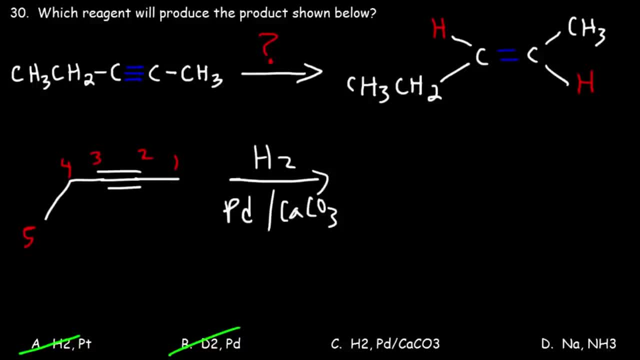 It's deactivated once you add an ionic compound to it. Instead of calcium carbonate, you can add barium sulfate. So if you see palladium over barium sulfate, this still represents the Lindler's catalyst. So what it's going to do is: 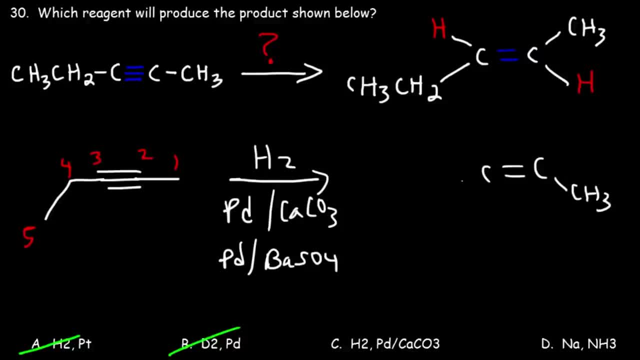 it's going to convert it into a cis-alkene as opposed to a trans-alkene. So this is the product of the Lindler's catalyst using this as the reactant. So we can eliminate answer choice C, which means that we know.